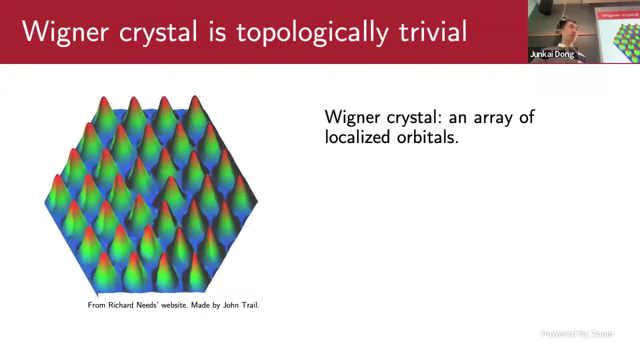 trivial Here. You can see that Wigner crystal is basically just an array of localized orbitals. However, usually when you have a topological electronic system you fill some topological band, and topological bands are not made of localized orbitals. 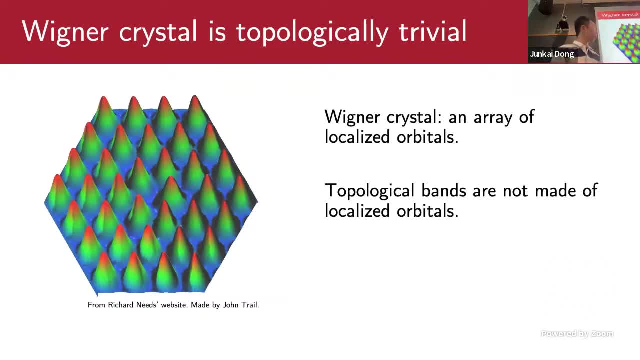 When you run your eyes on wave functions of topological bands, you need necessarily you need to get parallel tails, and you know they're not exponentially localized. So I think there is an interesting question to be asked here, which is: is there even? 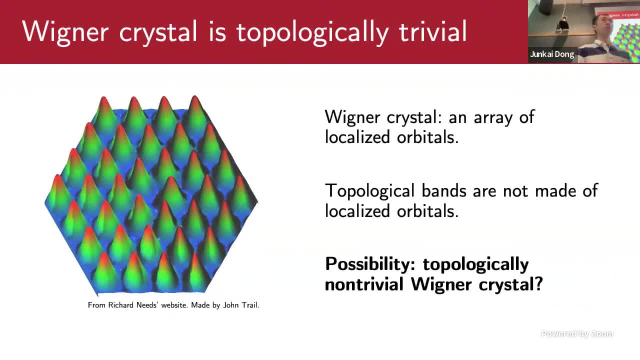 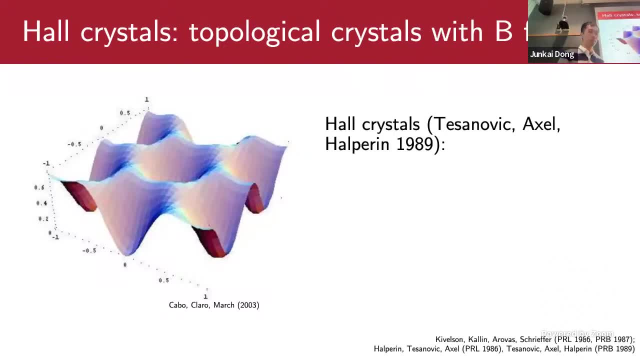 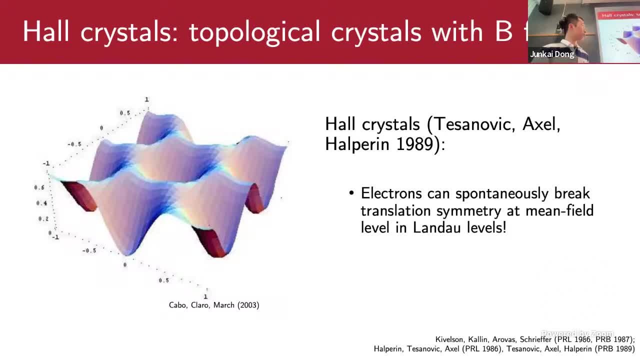 quite complicated interaction for electrons in lambda levels. They put electrons in magnetic field and they control the filling such that the electronic filling is exactly one per magnetic flux. So electrons will exactly fill one lambda level And due to the engineered interaction they showed that under Hartree-Falk approximation. 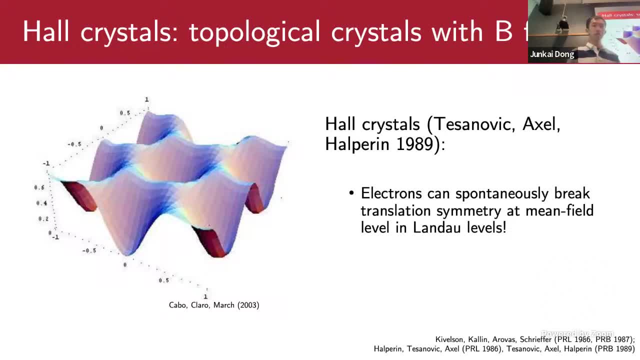 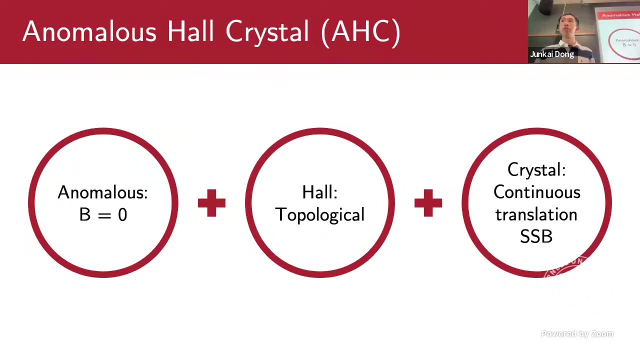 electrons will spontaneously break translation symmetry to form a state which is a crystal but also has a Hall response, And here the Hall response is really due to magnetic field that you have applied to the system. What we want today is the anomalous version of the Hall crystal. 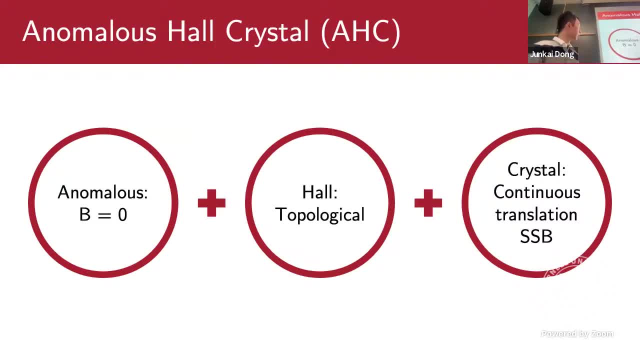 The anomalous Hall crystal refers to the following thing: It appears, It appears at zero magnetic field and it has continuous translation symmetry. However, it has a non-zero Hall response, meaning it has non-trivial Chern number and it spontaneously breaks continuous translation symmetry. 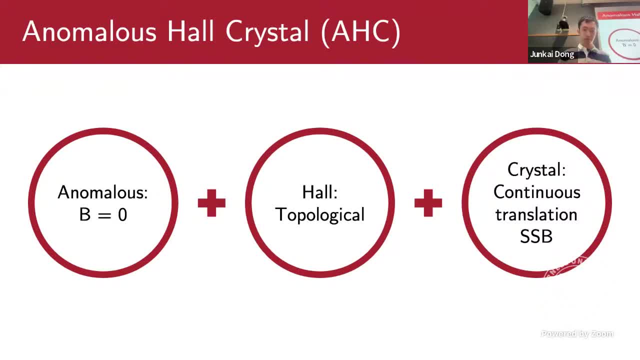 This state we will call the anomalous Hall crystal. Yes, How do you do this if you're undiluted to like a quantum Hall state using bubbles and plasma? All the quantum Halls actually both have the same state. 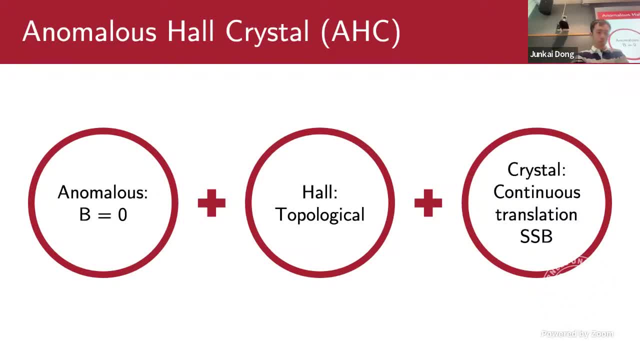 Very common. yeah, How does this work? This is a great question. So my understanding of it is the following: Quantum Hall stripes usually appear in higher lambda levels, For example, you know, at fillings, At fillings, for example, you know, three and a half. 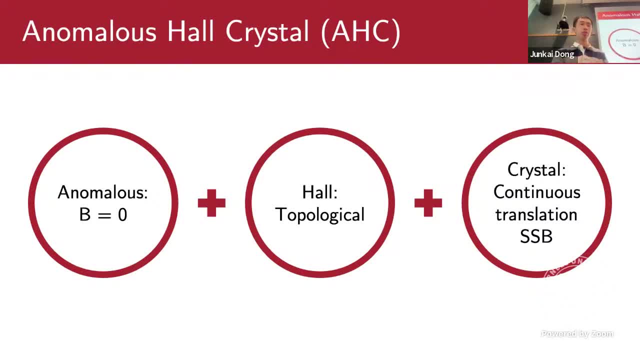 or you know five and a half, Then Then these stripes, stripes will form and if you just look at, for example, if we're talking about, you know, the, let's say, the fourth lambda level, you put half of the electrons into the fourth lambda level. 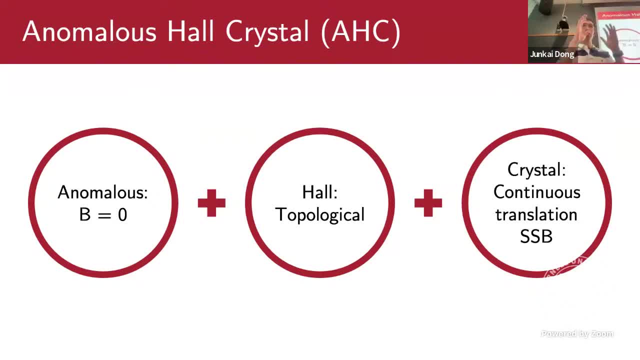 and you look at those electrons as a whole, they will form a Chern number zero charge density wave. So the charge, The charge density wave part, is topologically trivial and the rest of the electron in lower lambda levels will contribute a Hall response. 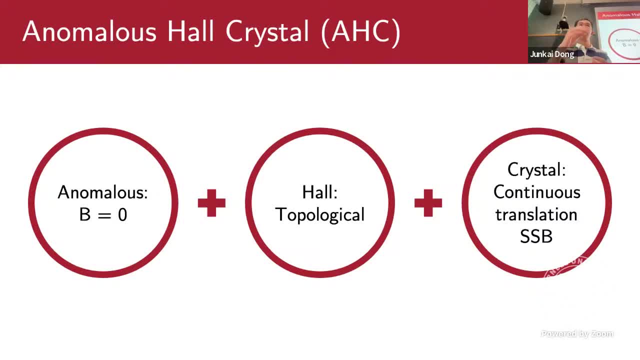 That's, That's what's different here. So in that case, for example in the Hall-Chrystal regime, you know you're really in very low lambda level index, You know you're really close to the zeroes lambda level. 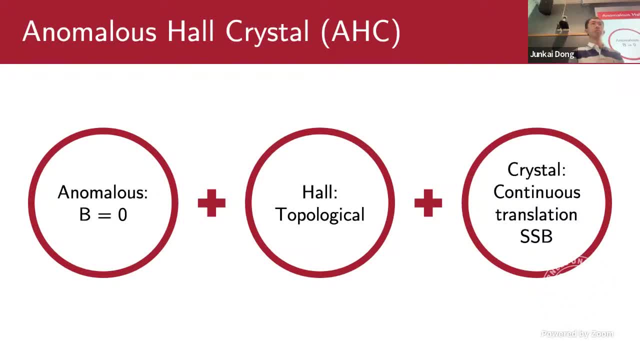 So from the observation point of view, from the symmetry point of view, they're different. From the symmetry point of view, they are indeed not different, you know. So you know, if you simply stack a A, If you simply stack a Wigner-Chrystal on top of a, 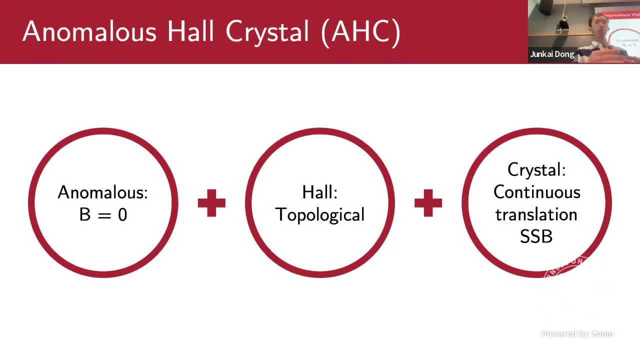 A. If you simply stack a Wigner-Chrystal on top of a A training slider, you will get something you know. if you package as a Hall something like an anonymous Hall-Chrystal, You're still bringing the whole structure. 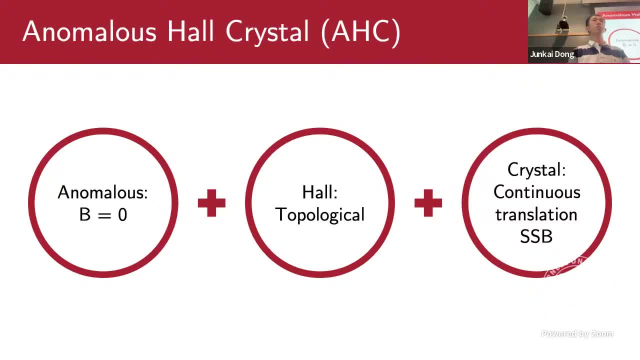 from objet level and then deal with the. Your lambda level is the lambda level. Yeah, yeah, yeah, yeah, yeah. So what those people did was not that bad. Well, you know, in the stripe business, the lower lander levels that contribute the Hall response. 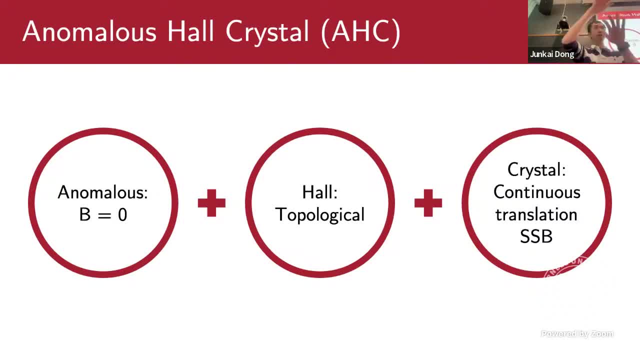 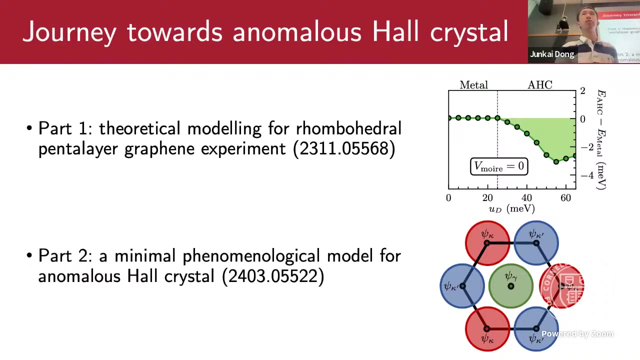 and the electrons that form stripes are really separate entities. OK, thank you. thank you, All right. so today we're going to take a journey towards the anomalous Hall crystal. I'm going to first discuss the very exciting experiment from Long-Juice group of rhombocytopenia. 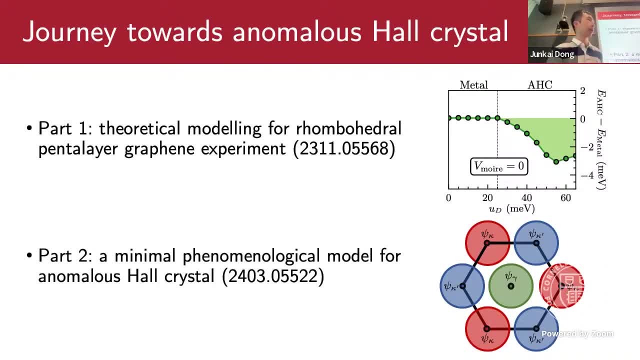 lyrography which motivated us to first think about the anomalous Hall crystal, And then, in part two, hopefully, I will convince you that we have constructed a very minimal phenomenological model for the anomalous Hall crystal state. All right, So. 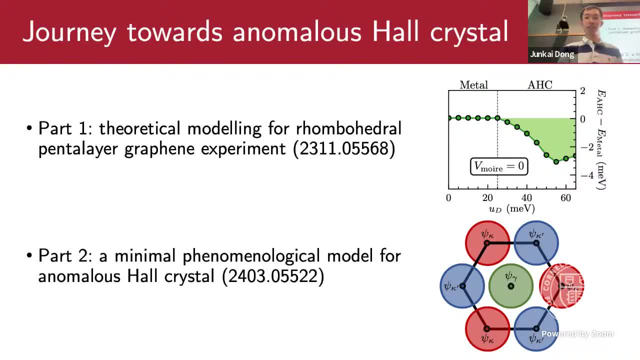 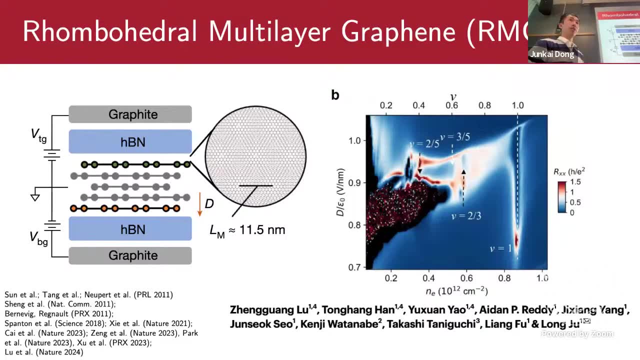 Given that Long-Juice has just come back a few days back, hopefully this part will be very straightforward. The experimental setup is the following complicated stack, But the main character is this material called rhombohedral pentalayer graphene. So by pentalayer I mean that there are five layers. 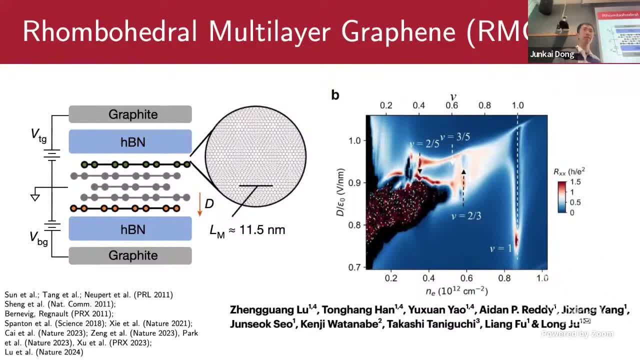 So each one of these layers is a layer of graphene, And they're stacked in this way, such that neighboring layers form staircases, And this stacking is called rhombohedral. Apart from that, they also encapsulate this rhombohedral multilayer graphene stack. 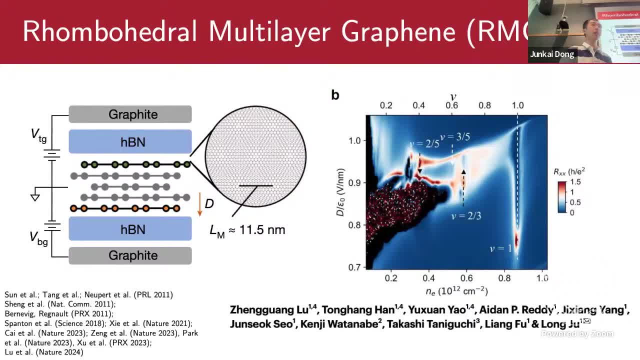 with two slabs of HPN. HPN crystals have a very similar lattice constant compared to graphene, So when the two crystals are closely aligned, they form a moiré pattern. Indeed, there is a moiré pattern. The moiré pattern forms by the top HPN, but not the bottom HPN. 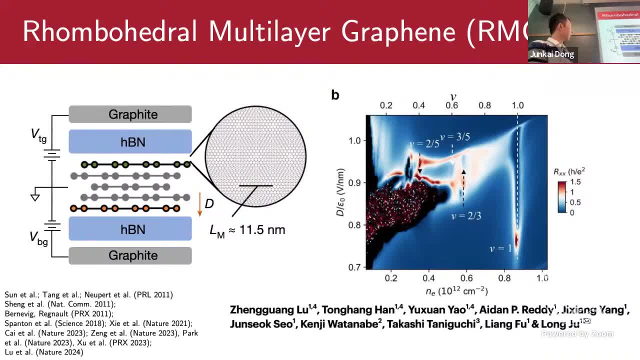 This is very important. Apart from that, they also have two gates, The top gate. both gates are made using graphite And by tuning the voltages of those two gates you can control the electronic density within the rhombohedral pentalayer graphene. 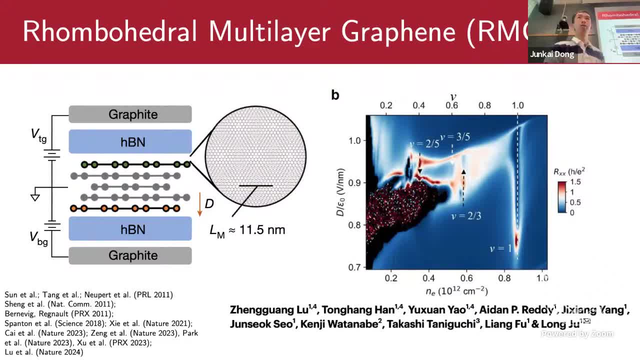 and a perpendicular electric field across the rhombohedral, pentalayer graphene, independently. This perpendicular electric field we'll call the displacement field. Your statement that there's no moiré on the bottom? that's because the twist is too large. Yes, 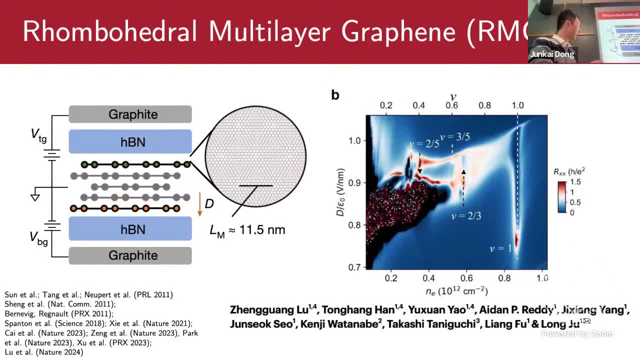 You know, it's completely unaligned. right, The top one is aligned, the bottom one is unaligned. Yes, Great. So here are the experimental observations at very high displacement fields. So this is something that we're going to talk about. 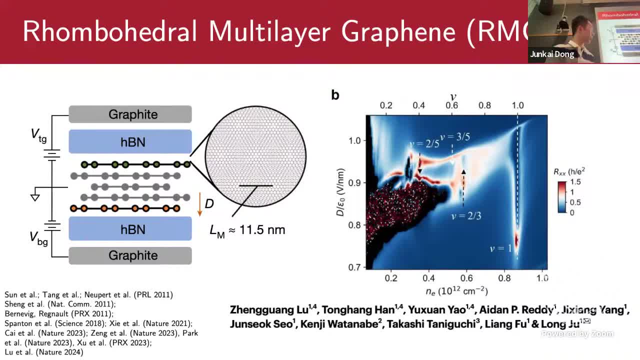 People have not previously attempted What they see at moiré. filling 1 is a train insulator, something that has rxx equals 0 and rxy equals to 1 in units of h over e squared. And what you see is that as you lower the electronic filling, 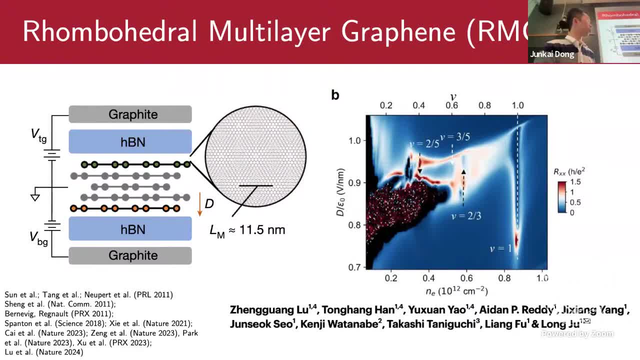 if you dope holes on top of the nu equals 1 state, you get fractional efflux. Yes, These are fractional states that are insulating with fractional Hall conductors. These fractional states are called fractional train insulators and they're analogs of fractional quantum Hall. 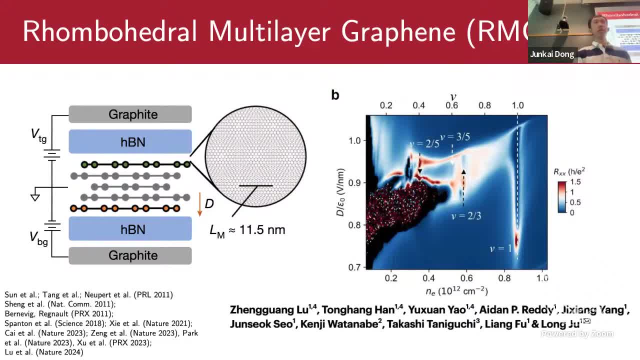 states in the absence of a magnetic field. They have been long sought for. In fact, this is only the second only platform to appear to host these states. The first platform was twisted MOTE2, which was studied by experiments. They were also studied by experimentalists. 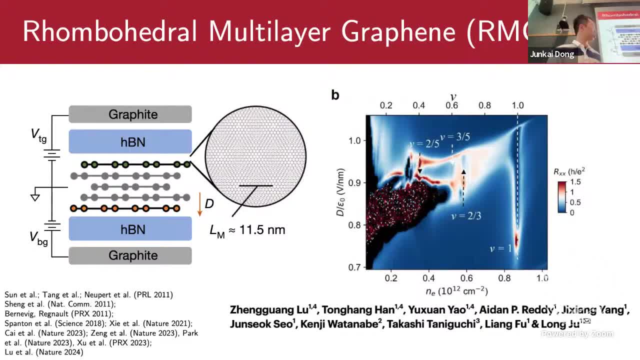 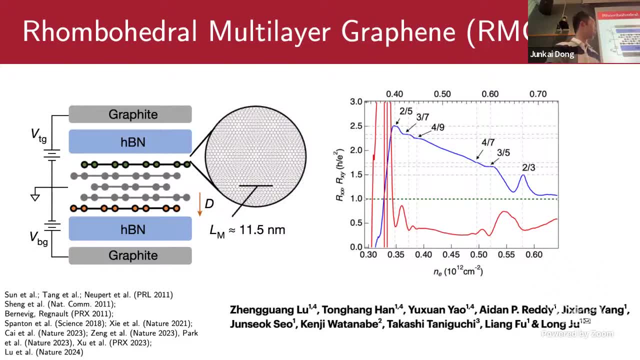 at the University of Washington, Kim Fai and Jie Shan here and Tingxin Li's group back in Shanghai JiaoTang University. So perhaps this line cut at a certain anti-displacement field is much more illuminating. You can see that there are a bunch of plateaus. 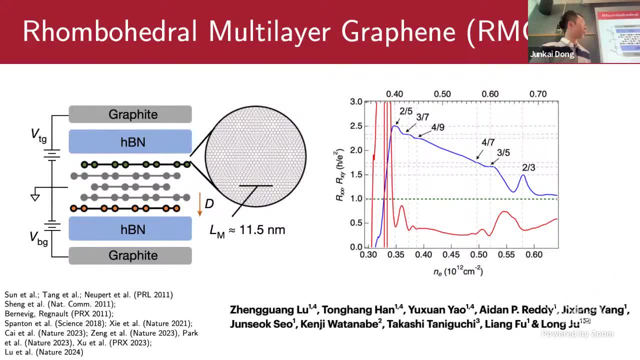 with fractions 2 fifths, 3 sevenths, 4 ninths, 4 sevenths, 3 fifths and 2 thirds. I would like to particularly highlight, you know, the fraction state which is 4 ninths, which has quite a large denominator. 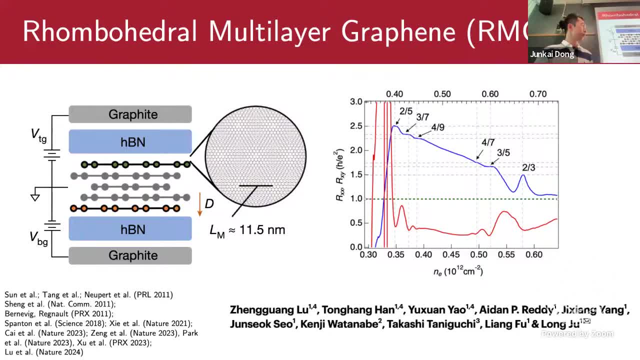 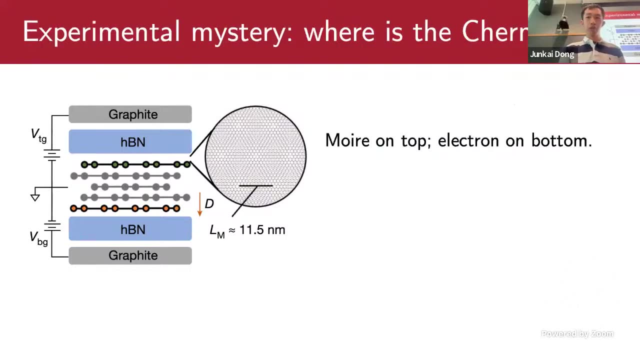 just illuminating the quality of the sample. OK, As theorists we're very interested in this material, you know, of course due to all the fractional states, But as it turns out, the integer state was already puzzling on its own right. 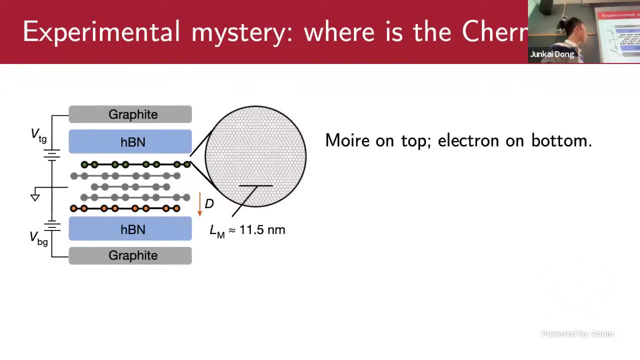 In fact, if you look at the setup, you immediately find a huge mystery. As I have alluded to before, the Moray potential really sits on the top layer right. The effect of the HBN alignment is really on the electrons on the several top layers. 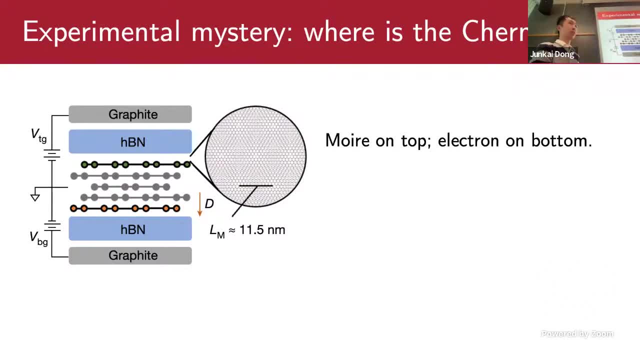 However, you apply a huge electric field and the electrons are going to get pushed down to the bottom layer So effectively. if you just look at those electrons, they should not feel available, Right Yeah, They should not have a very strong Moray potential at all. 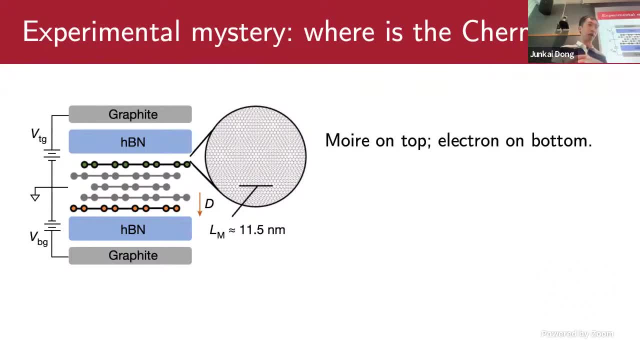 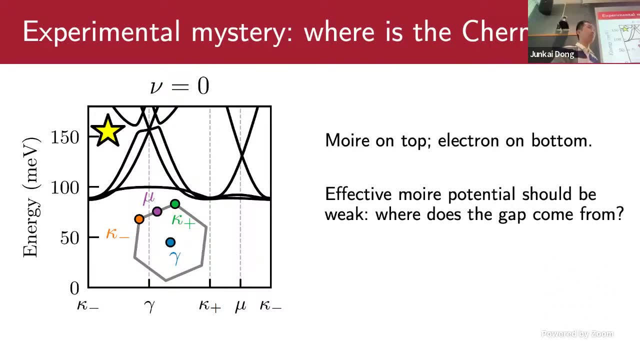 which means that they really have graphing scale or, in this case, continuous translation symmetry. This is confirmed by looking, just plotting the band structure, And what you can see is that you know there is no clear gap induced by the Moray potential. 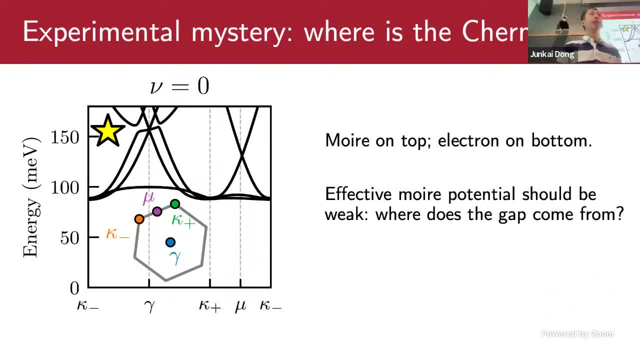 The effective Moray potential is very, very weak. Yes, If I choose, let's say numbers. what is the density of the difference between the top and the bottom layer? Something like, yeah, yeah, yeah, you know. something like 10%, you know 10%. 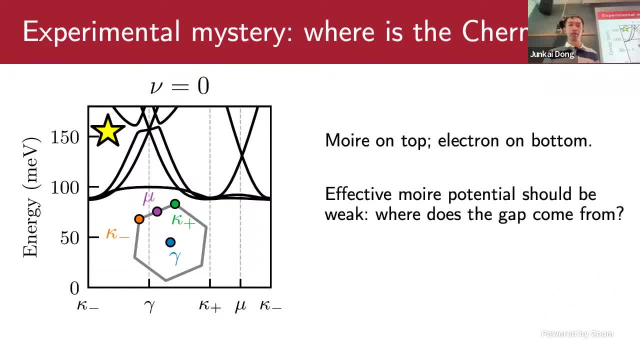 1 versus 10.. 1 versus 10, yeah, Something like that. Yes, If you did a different experiment where both of them were not giving Moray better, presumably then you would predict that they would still be the best OK. 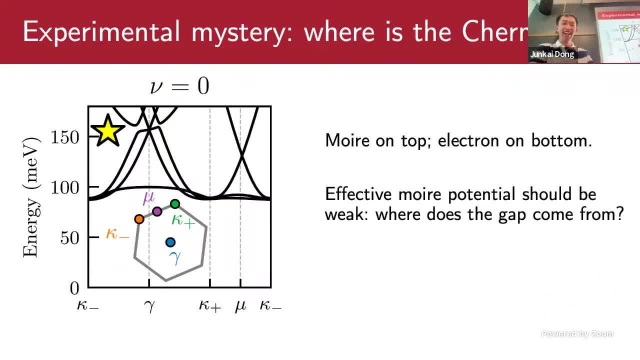 You're jumping. You're jumping Three slides ahead. Great, We'll touch on that very soon, Right? OK, And this immediately defies the current way that we understand these fractional translator states. Usually, the way we think about it is the following: 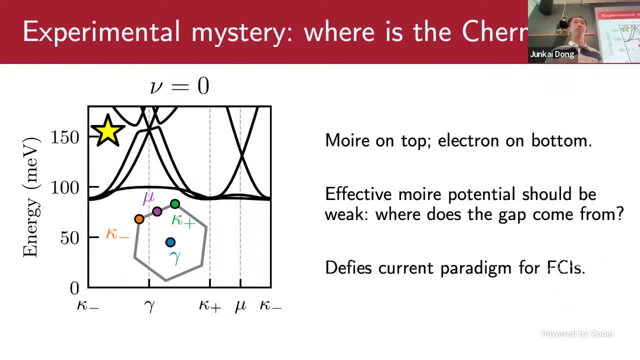 You take an isolated, very flat term band. You take it and you put some electrons into it, usually at a fractional filling, and those electrons will form some fractional states that are similar to lambda levels, and you are happy. However, here there isn't even an isolated term. 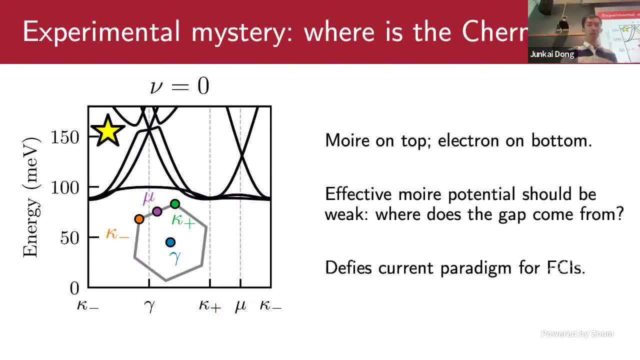 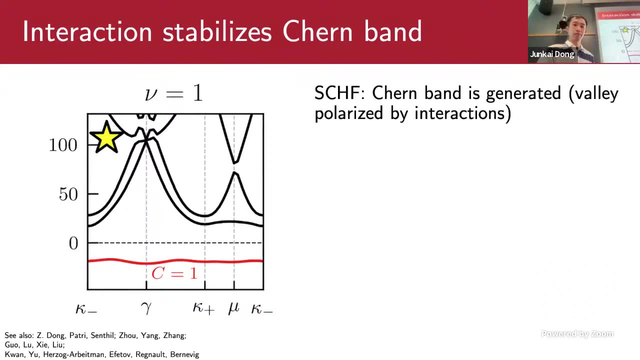 band to begin with, let alone talking about any of the fractional training layers. So the first step for us is to generate the term band. As it turns out, what happens is that the interaction will again stabilize a term band. This is self-consistent Hartree-Fock numerics. 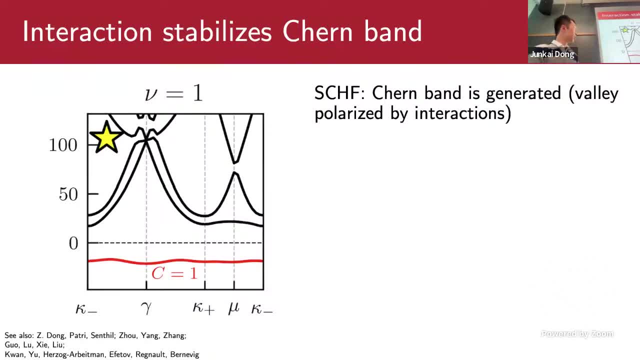 so completely mean field. What you see is that a term band gets separated out. This state breaks time reversal symmetry because all the electrons get polarized into one of the valleys due to the large density of states, So all electrons occupy this term band. 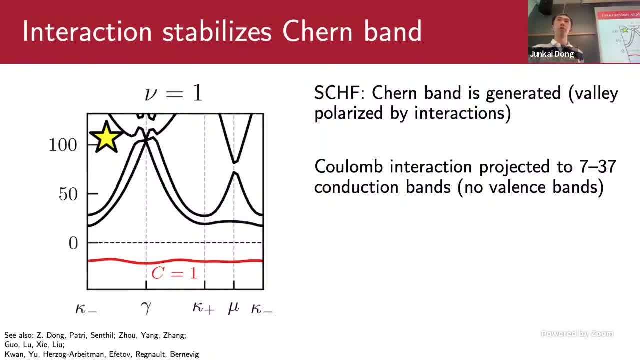 Just as an example- OK, Technical detail, this is Coulomb interaction projected to a large number of bands and we completely freeze the valence bands. So we assume that all the valence bands are completely filled and we only do numerics on the conduction bands alone. 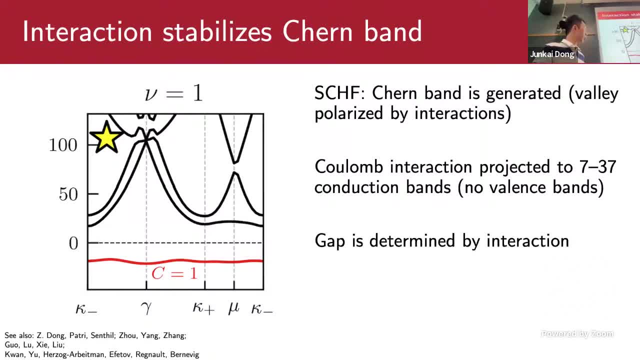 What is particularly interesting is that this single particle charge gap is determined by the interaction You can change. You can change all forms of your interaction, of your Moray potential to be. there has been debate about how the actual HPN creates the Moray potential. 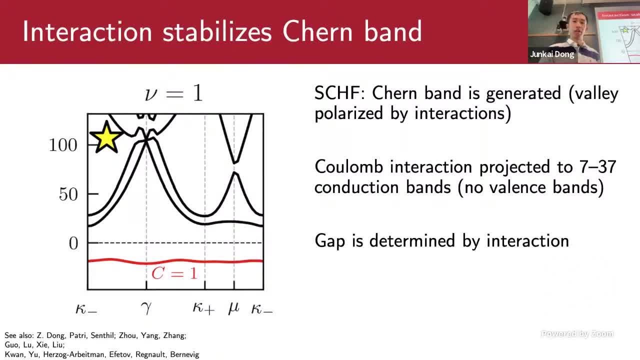 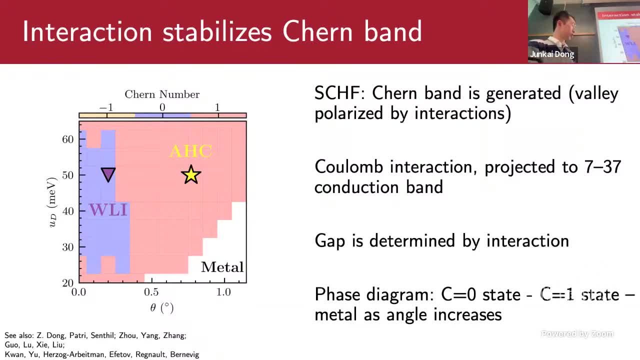 And in this calculation the gap is nearly unchanged. And if you can scan a bunch of parameters corresponding to different twist angles between the Rombaud-Hitler graphing and the top layer HPN And displacement field, what you see is that at low angles you get a turn number zero insulator. 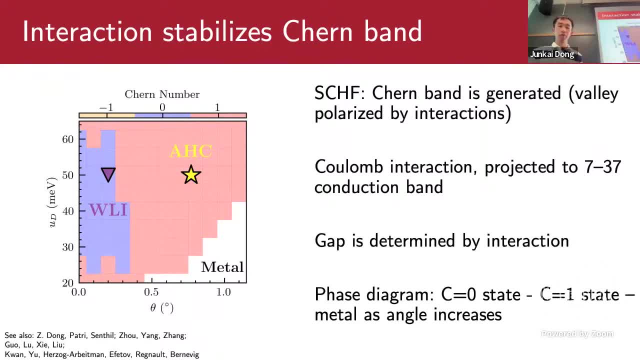 At large angles you get a metal, And in between them is this very broad phase of a turn number one insulator, which I will argue to be an anomalous Hall crystal in the next slide. Yes, Thank you. Thank you for the question. 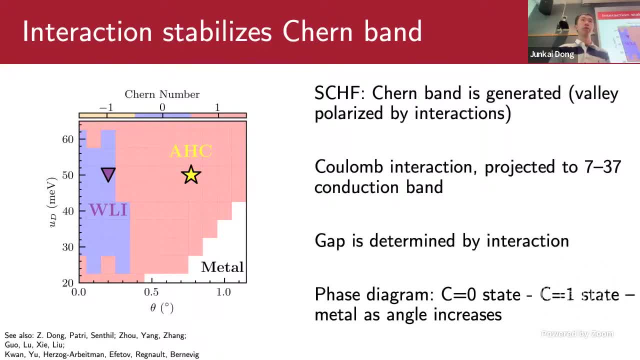 Well, what's the impact of the turn? What are you saying? Is it being polarized as well? Yeah, It is being polarized. yes, Also due to- yeah, also due to the same reason: large density of states, sonar, ferromagnetism. yeah, 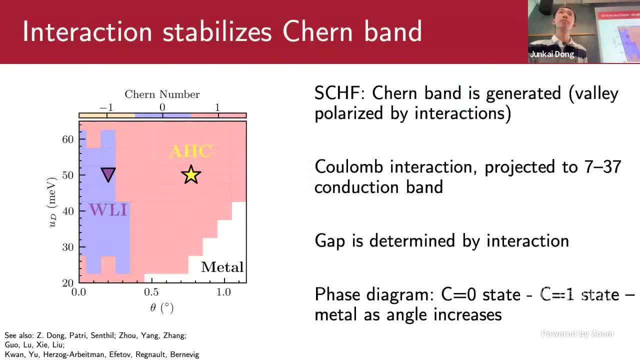 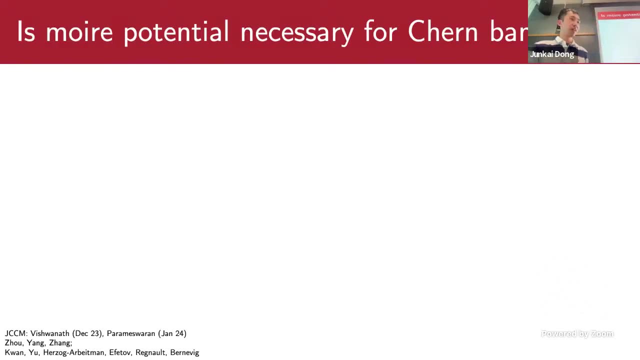 Great. So yes, You have said that this calculation is Moray in or not. This calculation Moray is in it. OK. Now, as very acutely pointed out by Chaoming and Jin, the question is: do we need even? 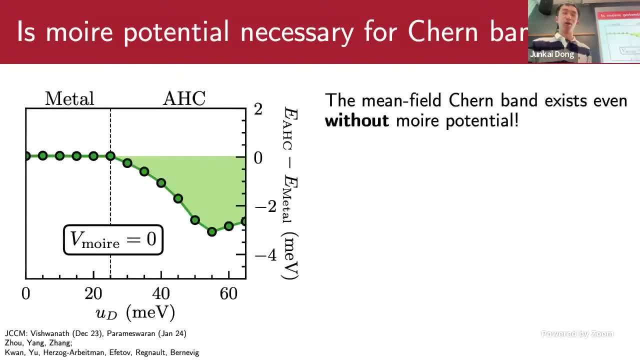 more in this in this case, And the answer is, of course, no. Now this calculation is done without Moray. Here, of course, we're still using a mean field approximation. We compare the energy of a translational symmetric metal versus the turn number one insulator right. 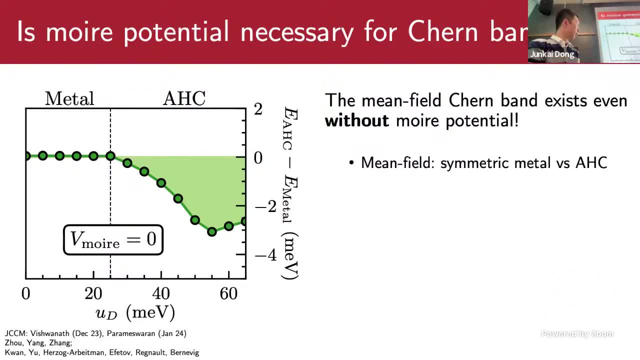 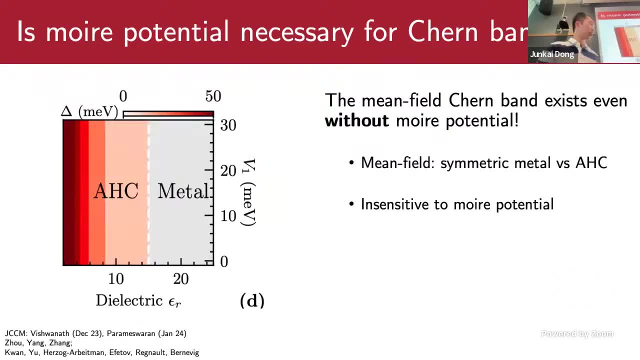 And what you'll find is that, you know, above a certain critical displacement field, the churn number one insulator wins. And of course, as I have said before, the charge gap is completely insensitive to the Moray potential. it's only a function of dielectric constant alone. This critical displacement field actually, 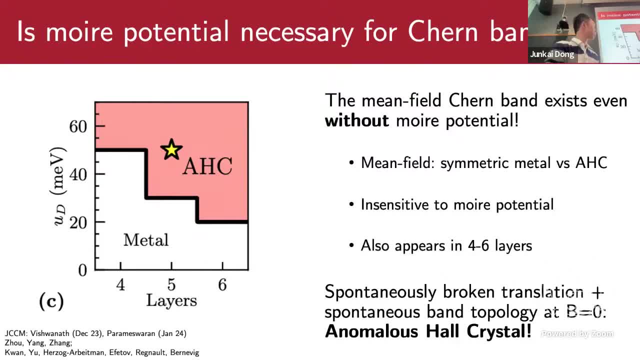 decreases as the number of layers, But the churn number one insulator still survives in different number of layers. So if there are any experimentalists listening to this talk, please make six layers And four. You can crank up the potential. So what I would like to argue? 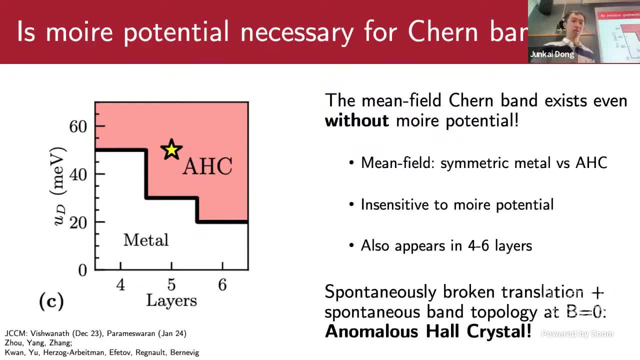 and at least in the current approximation, which is a very strong one in the mean field calculation, what we have found is that this state a churn number one insulator that spontaneously breaks translation and spontaneously breaks time reversal symmetry, And thus this is exactly. 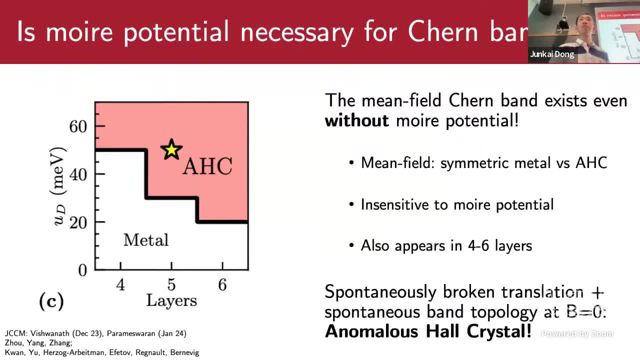 what we are trying to find. This is an anonymous Hall crystal. Yes, In this calculation, are you still assuming the band folding the Moray pattern is turning Moray potential to zero? Yes, So what we do is that we explicitly choose a free-wand zone. that fixes the way. 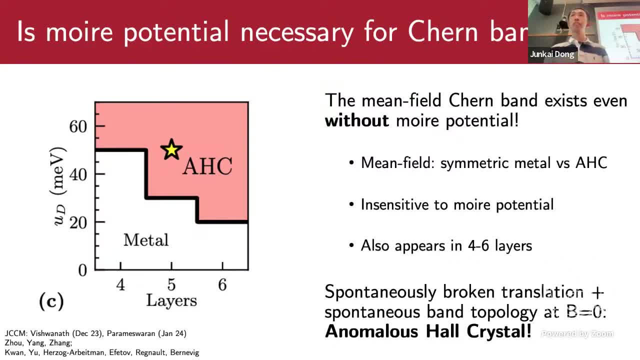 that the band is folded. So, yeah, So the spontaneously broken translations increase that insular. You can also try to optimize over different ways of breaking translations. That is also possible. Yeah, Related to phi, it sounds like you're, for example. 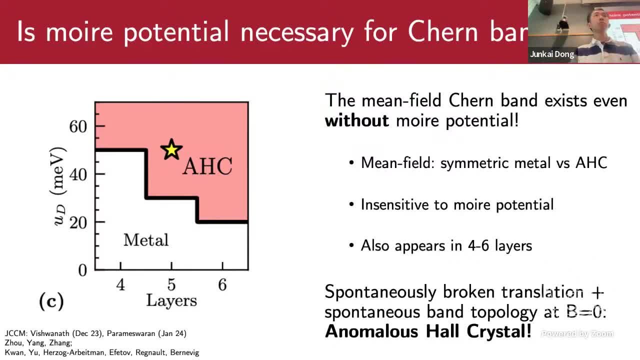 So it sounds like you're doing stoner paramagnetism, is it right? Which part? So is the mechanism large density of, say, stoner paramagnetism in some channel? The translation breaking is indeed induced in this way. yeah. 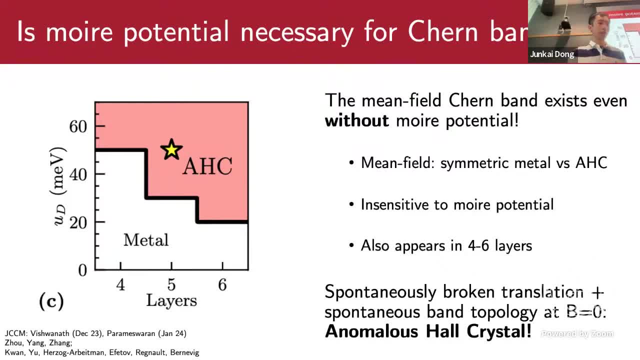 So basically, the band is very flat, right And OK. so the way I usually think about it is the following: If you have perfect nesting, then you know. of course you wouldn't be surprised that you know. translation is broken. 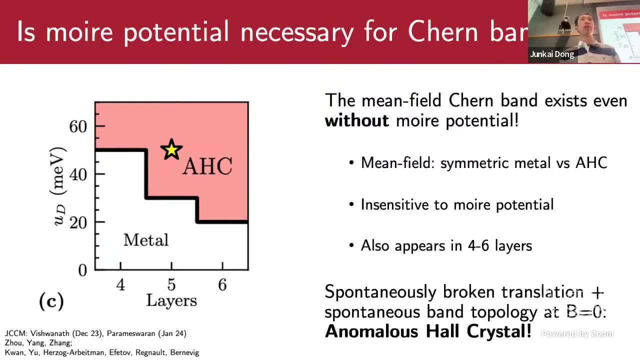 Then, if you know the band is flat enough, it does not cost a lot of kinetic energy to deform your Fermi surface into one that has perfect nesting And this gives you. You know, after the deformation of the Fermi surface it can gain interaction energy by breaking translations. 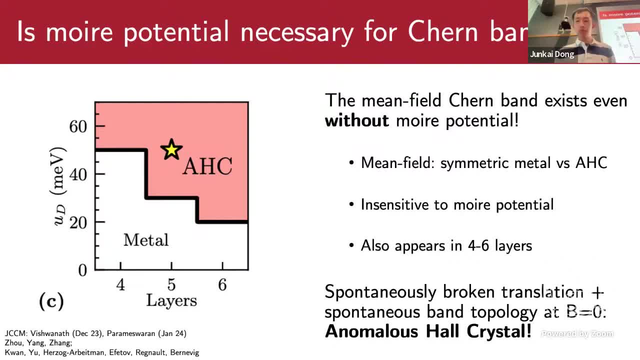 So you want to break two things. You want to break tangential and tangential, Yes, Yes So. and breaking transversal in stoner paramagnetism. So you want to break transversal in stoner paramagnetism: the density of the nesting effect. 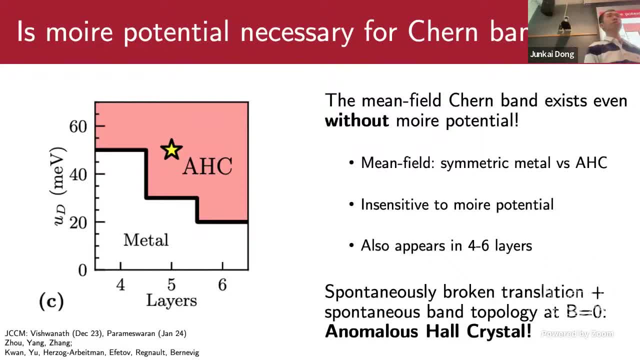 Yes And that, But that's not like orbital magnetism, or is it like? is there a spin on there, OK, so? So you're doing something like stoner paramagnetism, which could be either with real spin or with little spin. 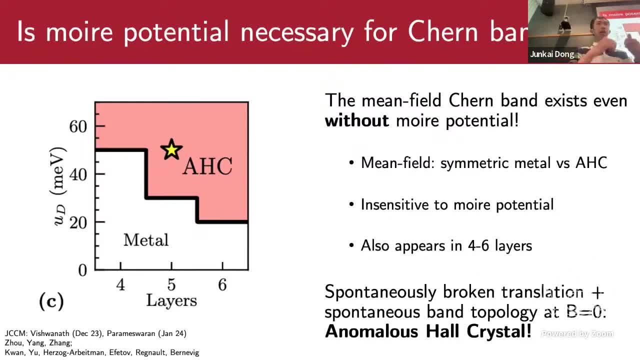 Yes, OK. So Why is the little spin negative, The k and k prime? So there are two valleys. Your valley break, Yes, yes, yes, yes, yes. So you're valley breaking, Your valley polarizing, And and you're getting translational symmetry breaking because it's less flat, or? 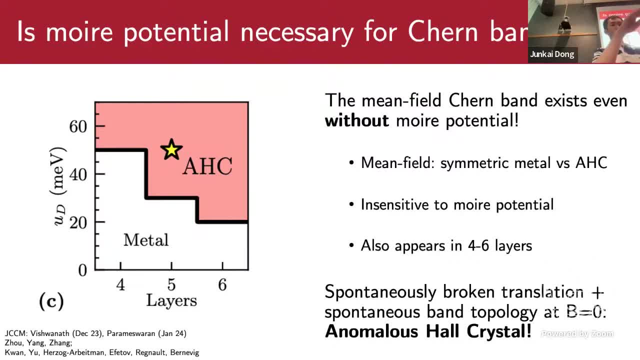 We're getting translational symmetry breaking because the band you know around the valleys. So, for example, if you look at, you know the band structure around the, the point k, then the band is very flat. That will give you. 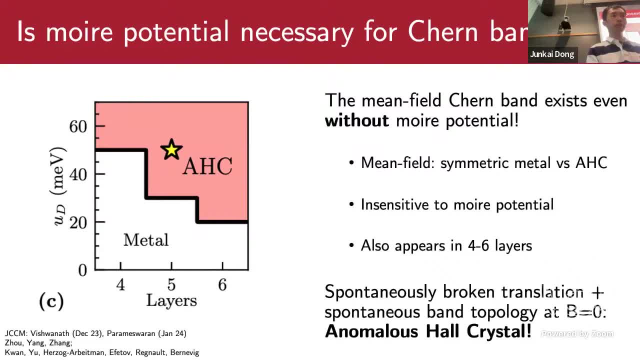 So what sets the periodicity? What sets the periodicity? The electronic density sets the periodicity. You're going to look at a Fermi surface and try to find something there. Is there a warping involved or Here I don't know what, what's the precise meaning of the warping? but you know, we do take into trigonal warping, which is 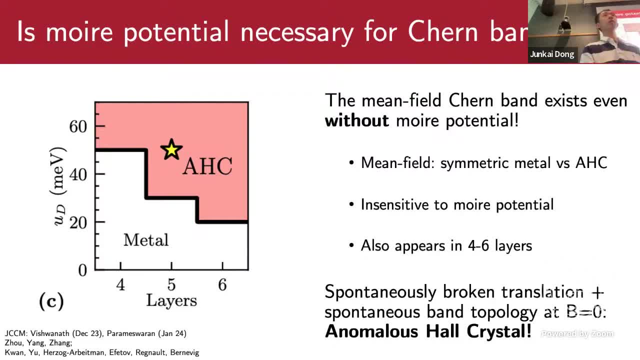 Yes, You need to somehow get the length scale out of something. Yeah, yeah, yeah, yeah, yeah. And why do they happen simultaneously? Why do they happen simultaneously? So You can break the valley. You can use CDW. 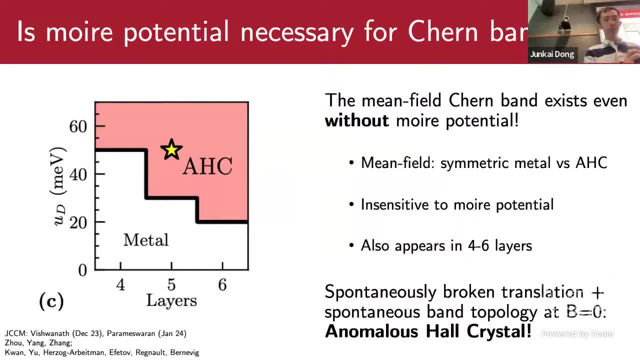 They don't have to happen simultaneously. Indeed, they do not have to happen simultaneously, And you know, as we have seen for for for many, many times, they do, in fact, most of the time, do not happen simultaneously. 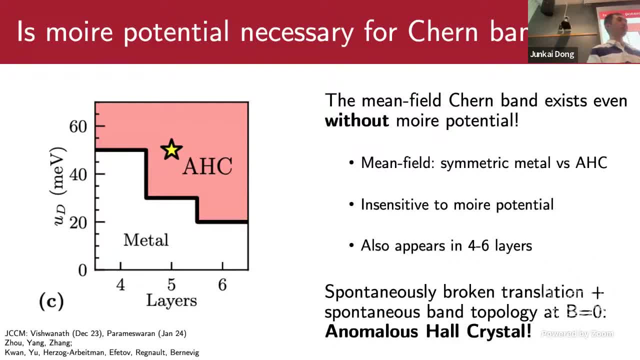 Why this happens simultaneously, probably. Yeah, I don't have a great answer for you at this moment, But the neurotic of the state is a valley-polarized identity, A valley-polarized, I would want to say, Wigner crystal, because charge-density wave almost implies that. you know, you will originally have a, have a lattice and you're just, you know, breaking discrete translation symmetry. 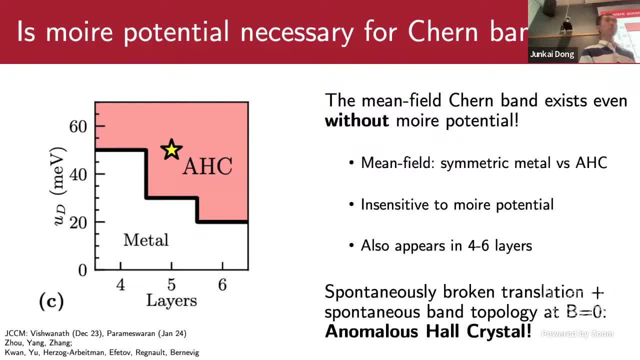 Here. you know it's really incommensurate. I just want to understand, in the symmetry sense, what is the state. In that sense, you know it's a. In that sense it's a, It's a valley-polarized. 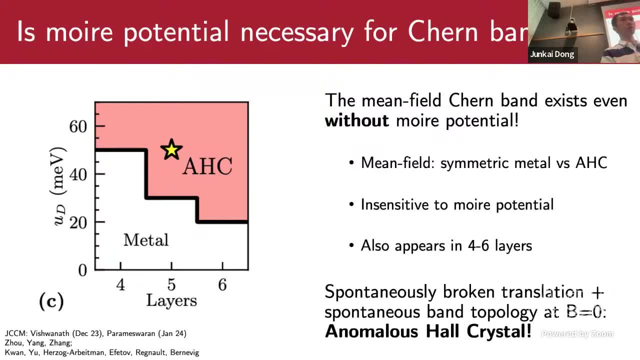 charge-density wave, But you're deriving it by density. Yeah, yeah, yeah, Something like that. Yeah, That, Yeah, that breaks continuous translation symmetry. and, yeah, topological balance. Great, Thank you. Thank you. One thing to return to. 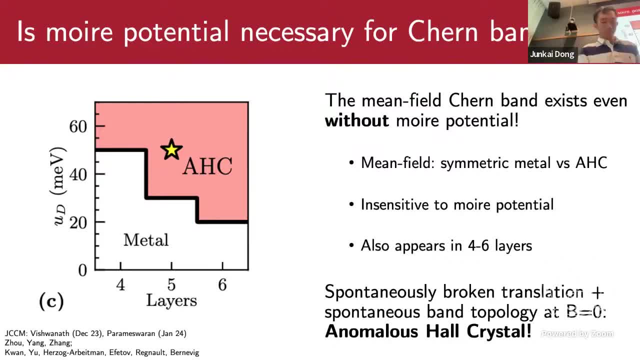 Yeah, It's actually related to this question. If this thing exists purely on the continuum, the density does not have to conform to whatever the Moiré scale gives you. Absolutely not. Principles make any refinement, Yes, But I suppose in the real system somehow they magically turn out to be in both same OR same number. 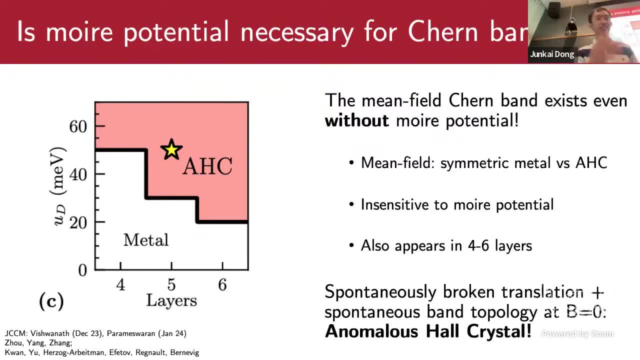 Three slides later. Okay, But yes, in, But no, indeed, indeed, they do turn out to be, you know, the same magic number that you know Basically, one way to think about this is, you know, the Moiré line scale gives you a Brillouin zone. 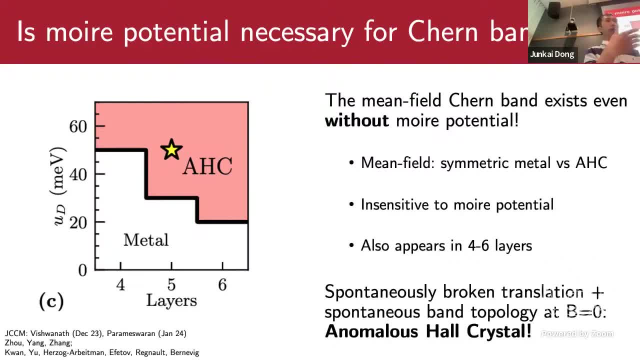 And the Brillouin zone. Within the Brillouin zone you can look at how flat your band is. You know the folded band. you know the bottom band of your folded band structure. If that folded band structure is very dispersive you're not going to get dispersion. 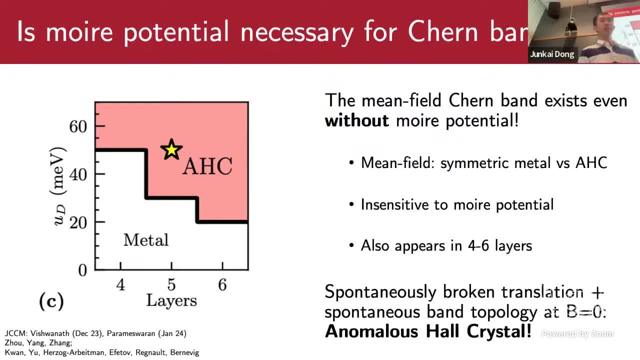 And it just happens that the electronic density and the Moiré potential just fit together such that the dispersion is very, very flat. Yeah, Why don't you get a state supremum? Why do I not? How to say this? So one, I don't really. 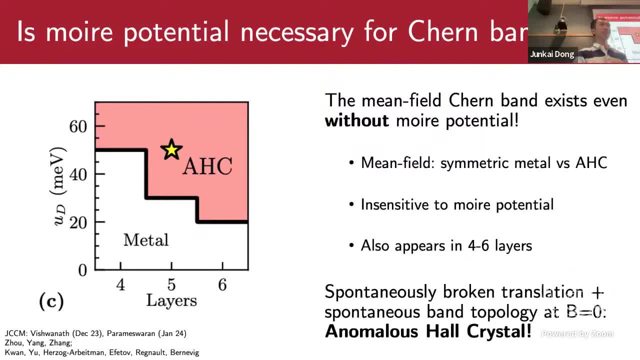 Okay, How to say this? So one. indeed, in lower number of rhombus hydrography, the superconductivity is seen Right, You know, for In my calculation I mean in this case I'm using repulsive interaction. 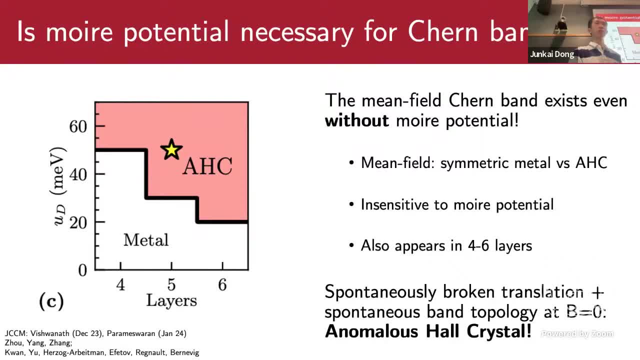 So I'm not sure where the attraction between electrons could come in here. I'm not sure what's the glue for the Coupe pairs. Do you think there's superconductivity out of the repulsive interaction That's, from SOC modes or something right? 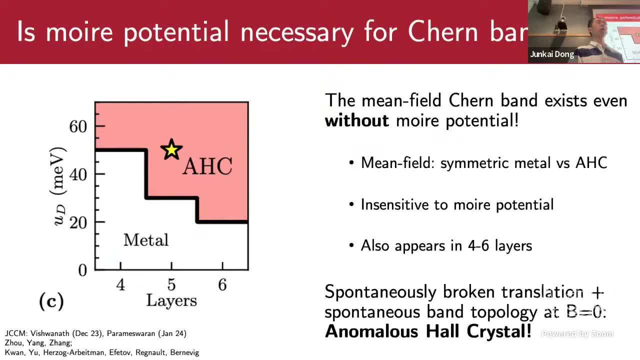 Or Can you do that again? Oh, I see, I see it. So within your GPL theory, you're doing repulsive interaction, which will only give you a bit of a ferromagnetism of Yes. Yes, We have not considered. 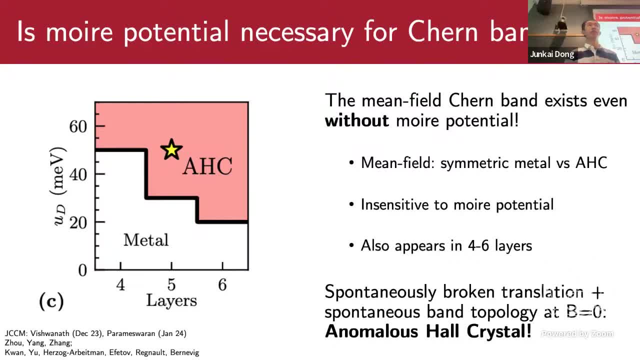 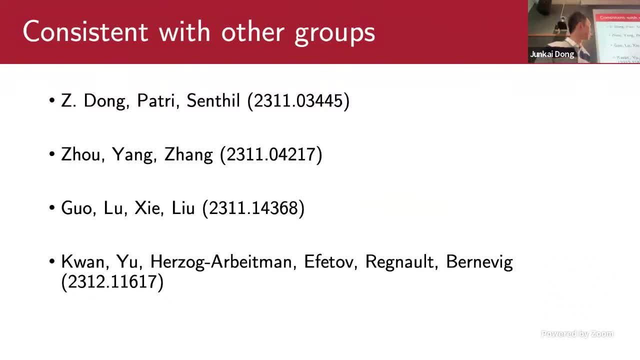 Yeah, Excellent. Okay, I guess everyone agrees that this is a cool state. I would like to also highlight some simultaneous works, a whole bunch of them from, you know, Central's group at MIT, Yahui's group, Jianfeng Liu's group and Andrei's group. 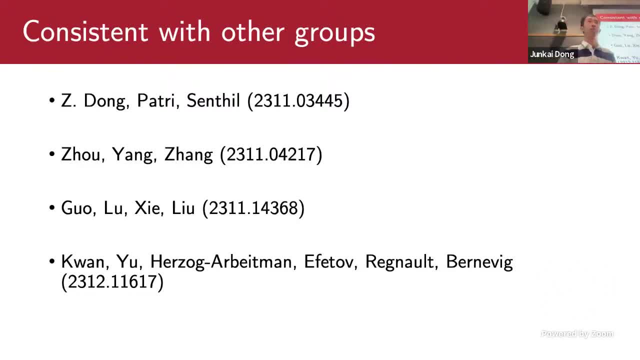 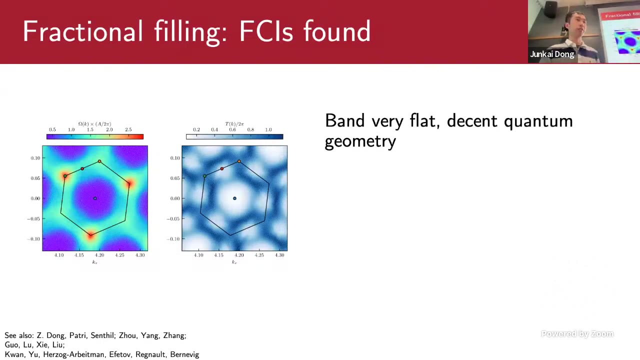 Particularly Yahui's group also found that the churning insulator in this setup could be interpreted in the framework of spontaneous translation: symmetry break And, of course, upon doping. on this band that was just formed you can find fractional churning insulators. 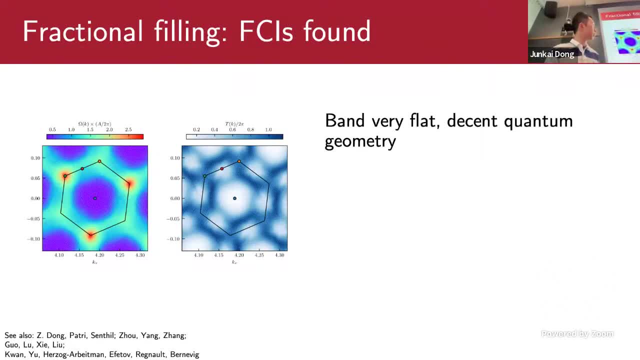 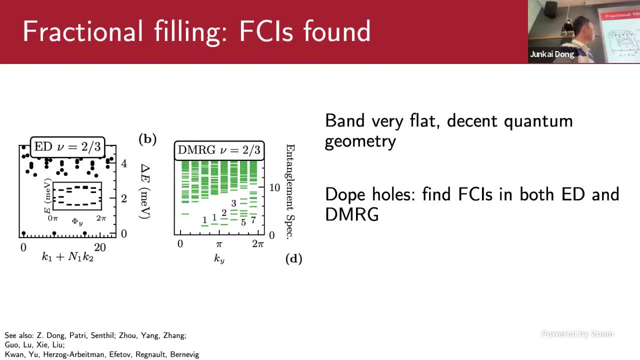 The band is quite flat And it has very decent quantum geometry. The trace condition violation is not very large And you know, when you put holes in them- to set nu equals two-thirds, you will find fractional churning insulators in both exact diagonalization through spectral flow and 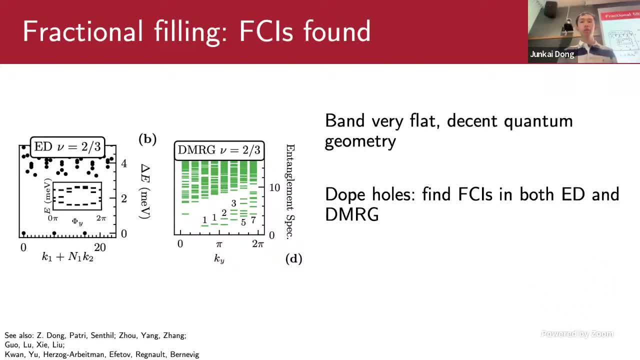 DMRG through entanglement spectrum. All right, There is a caveat that I would like to warn everyone against. These calculations are projected into the Hartree-Falk band structure that we have obtained, So we have restricted our effective Hilbert space to the orbitals that are forming the 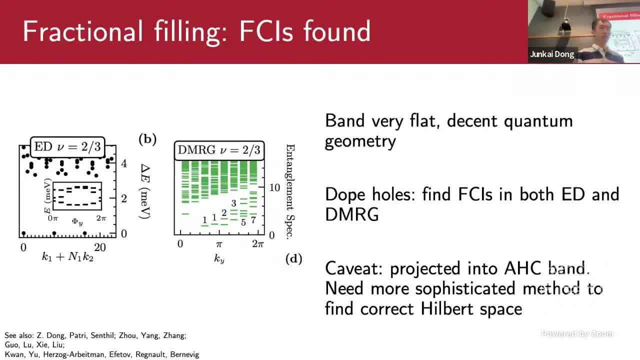 anomalous Hall crystal band. This is, of course, a quite uncontrolled approximation And we know that it would become false when the electronic filling is much, much less than one. For example, at nu equals, you know, 0.01,. the Hilbert space is definitely not correct. 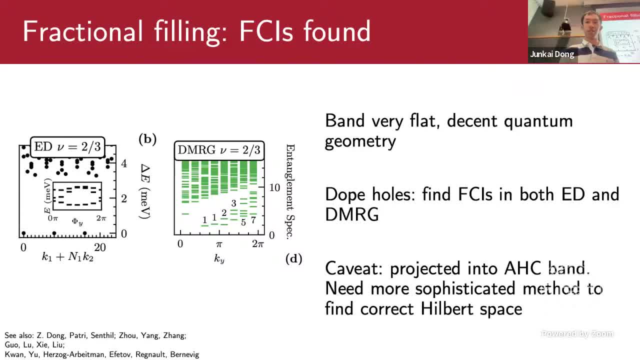 And in fact, you probably need a more sophisticated method to find the correct Hilbert space. Yes, So with your first d252 box, Yes, Yes, Are you double counting interactions somehow? Or, like, how do you make sure that you're not double counting interactions? 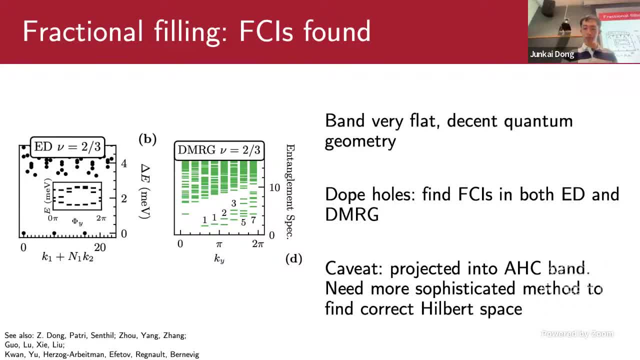 Good. So what we do is the following: After you perform your Hartree-Falk procedure, you get your filled states And you know you start from the normal ordered interaction with respect to charge neutrality and project into this Hilbert space. 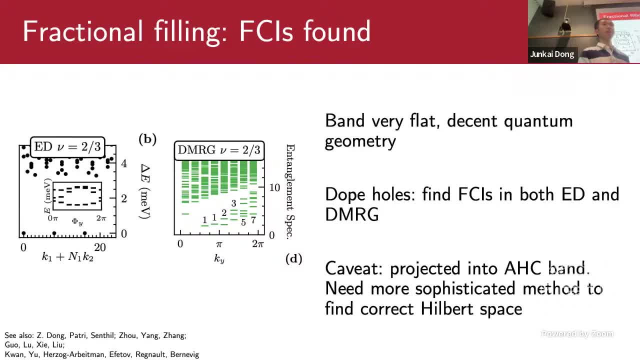 That is a completely legal procedure And in that sense, we're not double counting the interactions And yes, as you pointed out, there is a real danger of doing so. All right Now for the million-dollar question: is the experimental state a crystal? 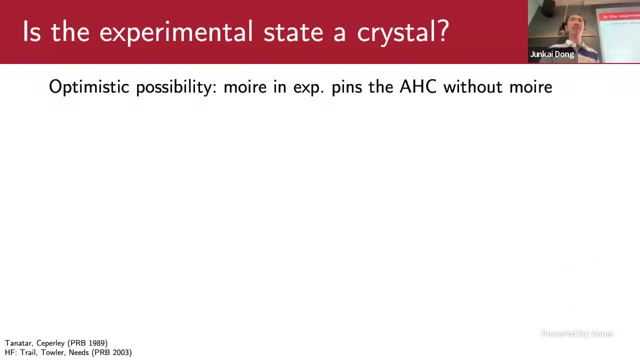 We want to be cautious here. right, There is indeed an optimistic possibility that you know the experimental state. if you, completely you know, don't have moray potentials on the top layer and the bottom layer, the system is completely translationally symmetric. it might be a crystal. 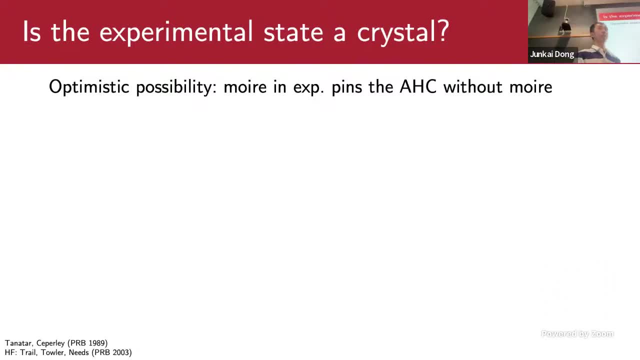 And what the actual experiment that Long has performed shows is that, you know, the moray potential actually pins the translation breaking pattern to a certain you know lattice. There is a less optimistic scenario, which is also likely, Yes, Which is that you know. maybe the brown state, in the absence of a moray potential, is actually translation symmetric. 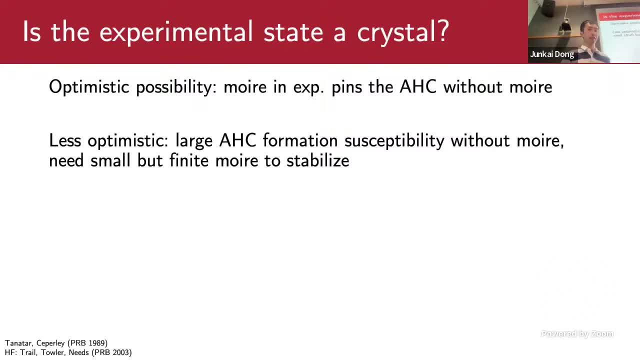 It's not a crystal. However, this state has a very large susceptibility without a moray potential. So you need a very small but still finite moray potential to get an anomalous Hall crystal state stabilized? Yes, But your susceptibility to…. But your susceptibility to will be determined by your furnace surface. 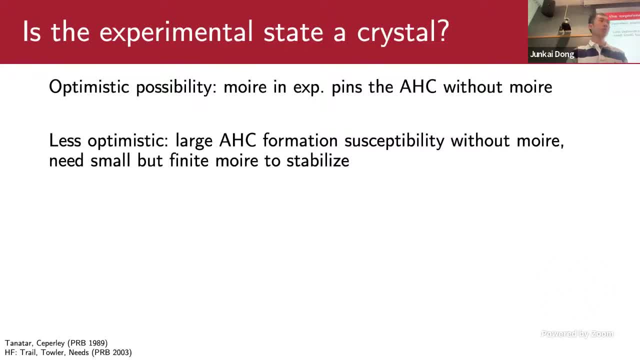 And that does not have to be in any relationship with the moray surface. I guess that would definitely…. Well, right, Right. So, indeed, if you applied a moray potential, that is, whose wave factors are completely off from you know, your KF and whatnot, then the crystal will not form right. 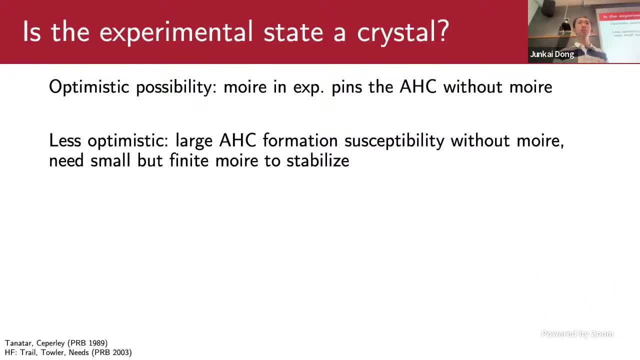 So these are speculations. Do I know the KF? You know, actually, you know, if you just look at the non-interacting band structure, the Fermi surface for the band structure I have plotted is quite complicated In the sense that it actually has a Mexican hat shape. 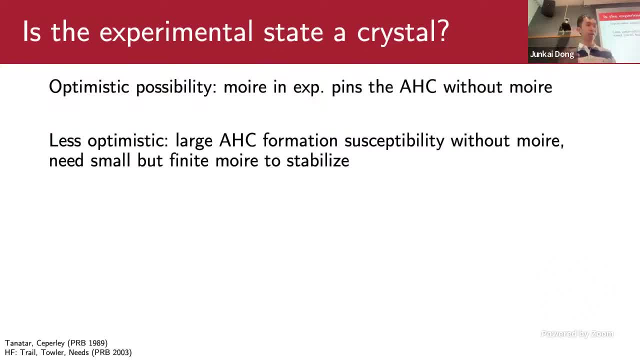 And thus, if you just very, very, very naively- you know form… Fill the lowest energy orbitals, you will get an annular Fermi surface And in that sense, I don't know if we should use the inner one, you should use the other one, you should use, you know, the average, something like this: 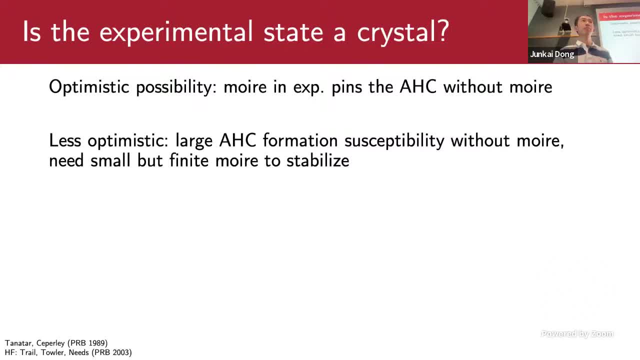 But yeah, Anyway. So I would also like to highlight the danger of claiming victory with Hartree-Fock, which is the tendency to… To form crystals, is way, way overestimated, if you just do mean field theory, because Hartree-Fock cannot capture the energies of gapless states very well. 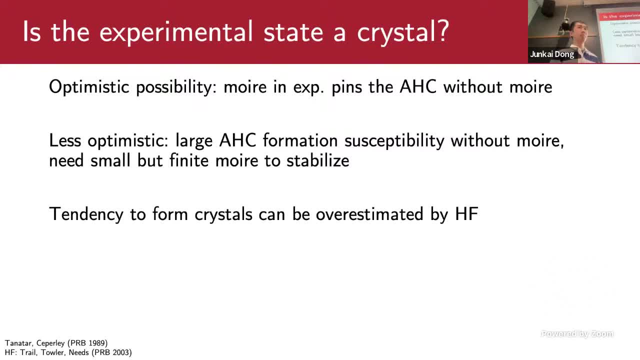 In fact, for the Wigner crystal, it overestimates the tendency to crystallize by a factor of 15 in interaction strengths or in RS. So we're by no means claiming that the state is definitely a crystal. Okay, There is of course also a question of you know what is actually the moray potential in the experiment, right? 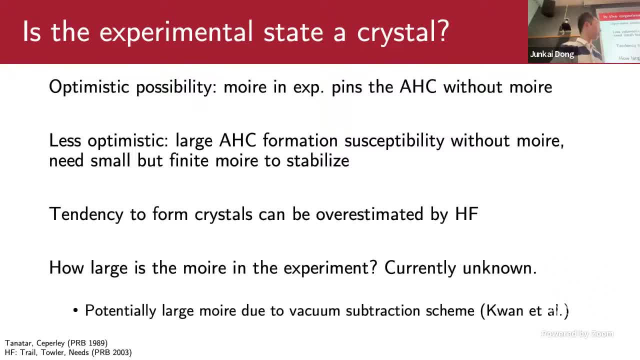 Because of modeling difficulties and whatnot. this is actually quite complicated and needs potentially more work from both theoretical and experimental fronts. What I would like to highlight is that, as pointed out by the paper from Andre's group, there is a potential enhancement of moray effects by the interactions due to different vacuum subtraction schemes. 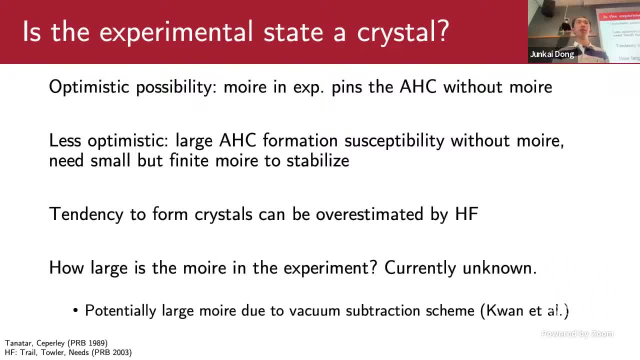 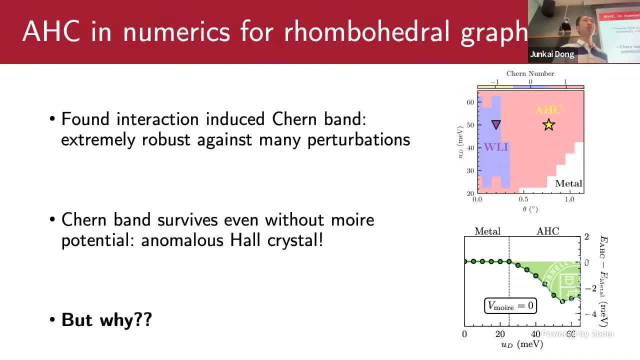 basically how you choose your charge neutrality, the state which represents your charge neutrality point. So difficult problems, Okay. So this concludes the first part of the talk During the process of modeling on this very exciting experiment of rhombohedral pentaliography. 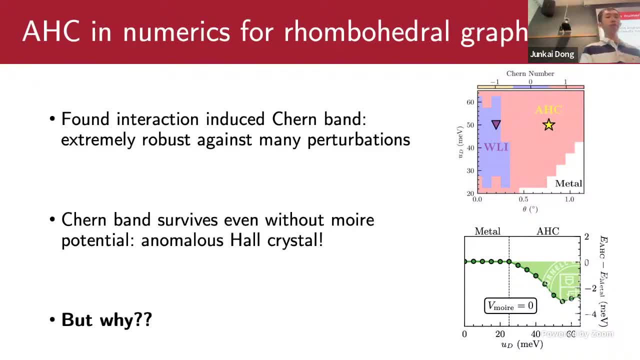 we found an interaction-induced churn band that is surprisingly robust against many, many perturbations, and this even survives without a moray potential, And thus at mean field level. we claim that this state is an anonymous Hall crystal. So so far I have presented you with just numerical observations. 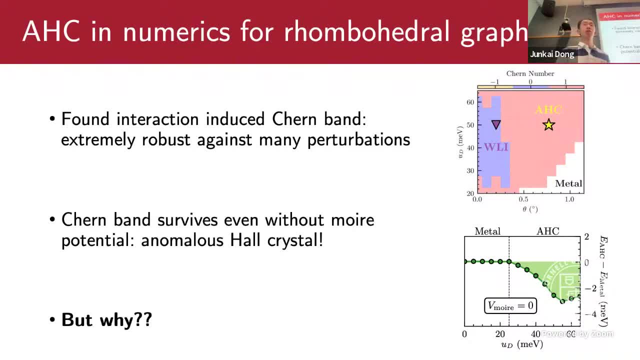 No physics is discussed In the second part of my talk. hopefully I will you know. I will talk about this minimal model that we have constructed to explain what we have observed numerically. Yes, Within the current setting. would you explain why the change of sign of the electric fieldwork is so important? 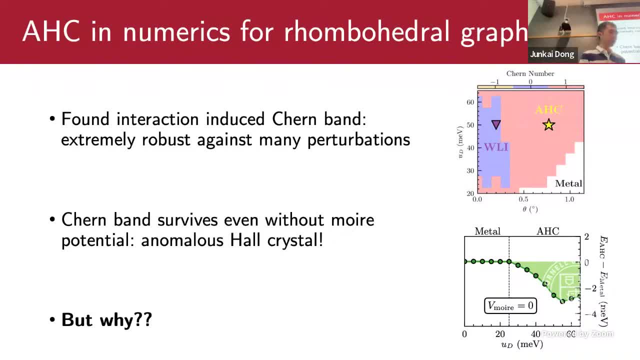 We do, we do, we do, And so, in fact, there is a very simple understanding. If you, if you just polarize electrons to the side where a moray is present, the moray potential will localize the electrons, You know. 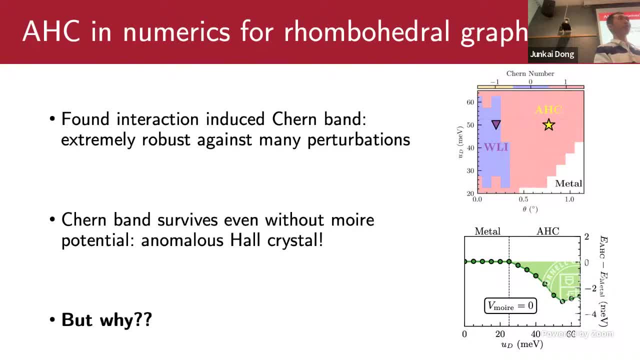 Well, you know, I wouldn't call it a Wigner crystal, It's a trivial insulator, right, Yeah, An equal one. you know, you, you, you, you have, Yeah, Exactly, Exactly, A fully filled, topologically trivial band. 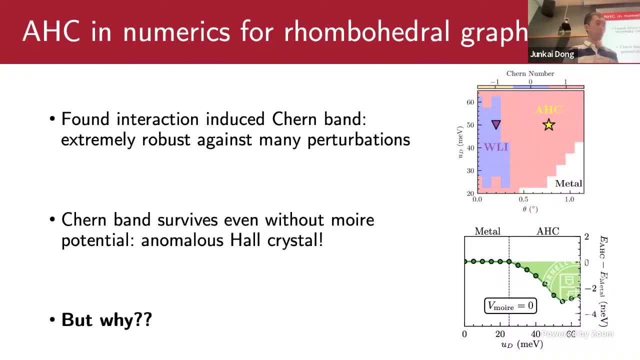 Yes, Yeah. So. however, however, there are also debates along that front, because you know, you don't actually know what's the form of the HPM potential. You have to choose. You don't know how strong it is. 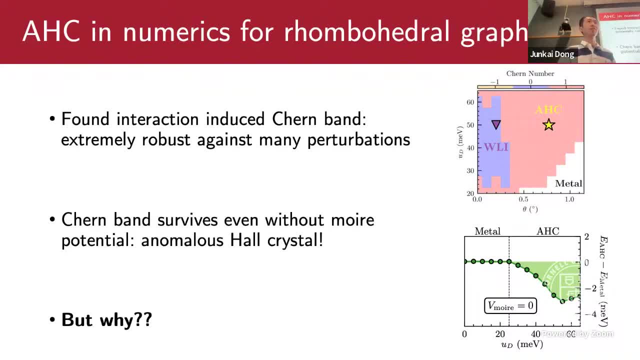 Well, yeah, Difficult problems. Who should have just gone? aligning, You know you would, you would, you would think, you would think not aligning things are are are not not very difficult, But I, I, I guess making examples are also very difficult. 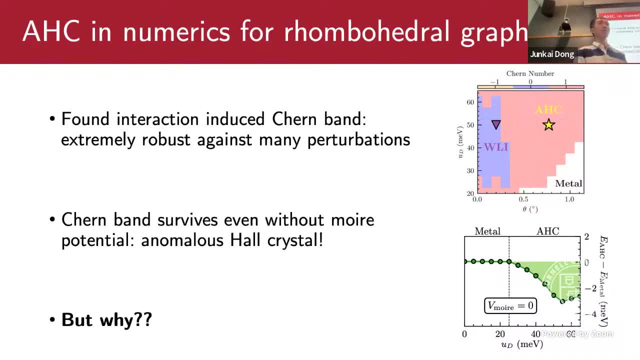 You know, rhombochedral stacking is not the most stable. stable stacking. Yeah, All right, Moving on to the second part. So to understand why the anomalous Hall crystal state even appears in our numerics, we have to understand the properties of the anomalous Hall crystal state a little bit better. 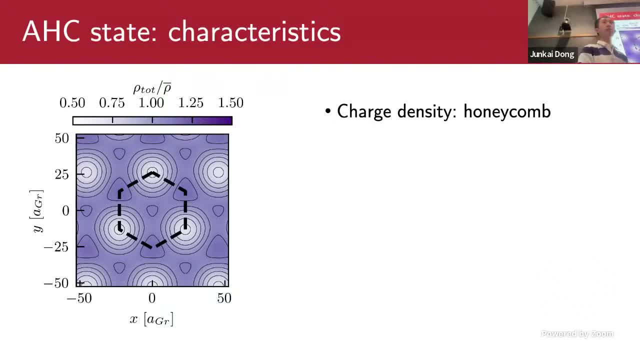 First of all, we can look at its charge density. Its charge density has nothing like the Wigner crystal which are, you know, triangular lattice shaped. This actually has a honeycomb shape in which you can see that there are two, you know. 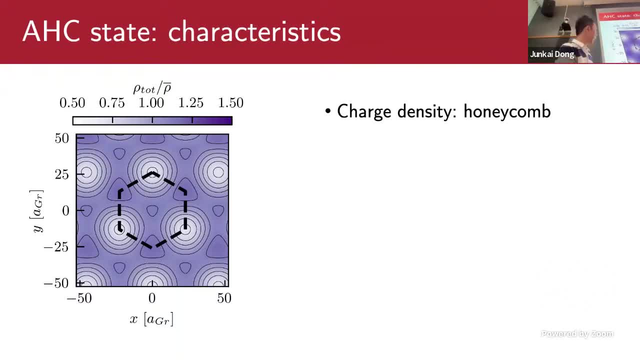 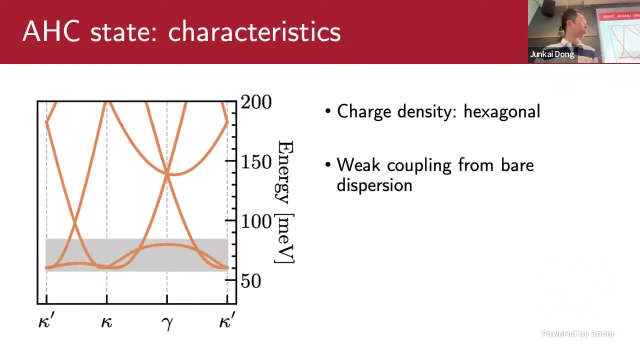 you can see that there are two peaks in the Brillouin cell and one dip Right. Wigner crystals are usually strongly coupled but the the anomalous Hall crystal state that we have found is actually very weakly coupled. Here on on orange lines I'm plotting the dispersion of the system which gives rise to the anomalous Hall crystal. 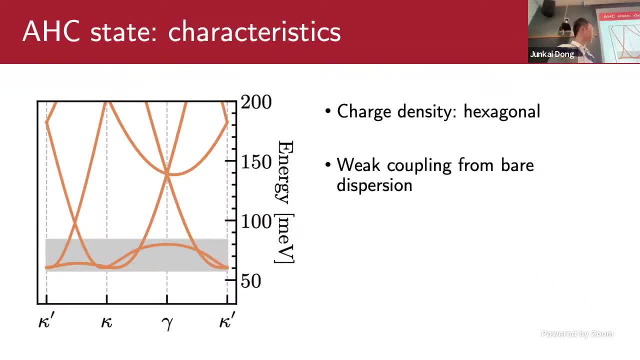 And in this gray shading I'm plotting the interaction strength. What you can see is that interaction cannot completely rearrange the band structure. Right, For example, you know, the state at gamma here cannot be strongly mixed with states up there, simply due to the interaction not being strong enough. 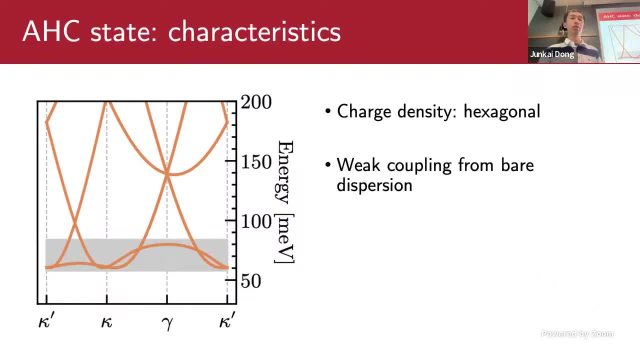 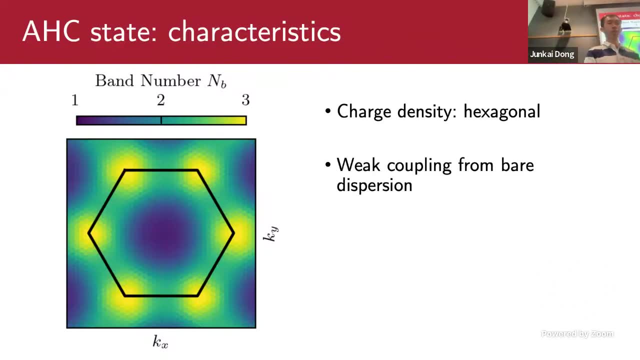 This weakly coupled nature is also shown in the following quantity, called the band number. Basically, what I do is that I take a field orbital from the anomalous Hall crystal state And I calculate how many non-interacting bands does it live on? At gamma point in the middle, the band number is one, which means that it corresponds to simply living on one non-interacting orbital. 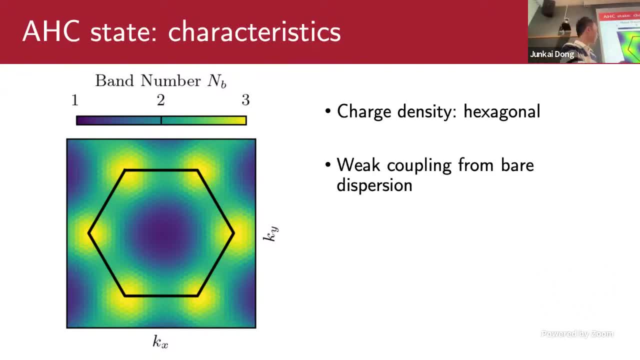 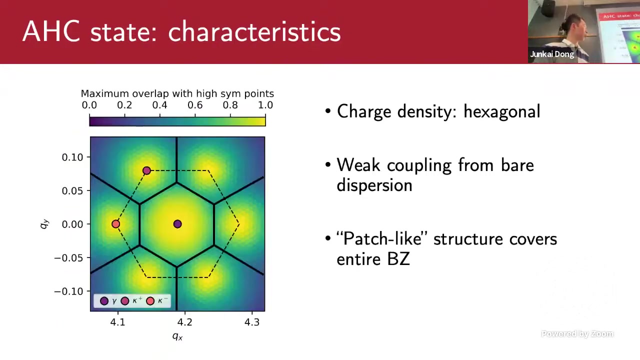 Whereas if I look at the kappa and the kappa prime points, the band number is three, which means that the the the anomalous Hall crystal orbital is basically a linear superposition of three Non-interacting orbitals. What's probably most surprising about the anomalous Hall crystal is its patch-like structure. 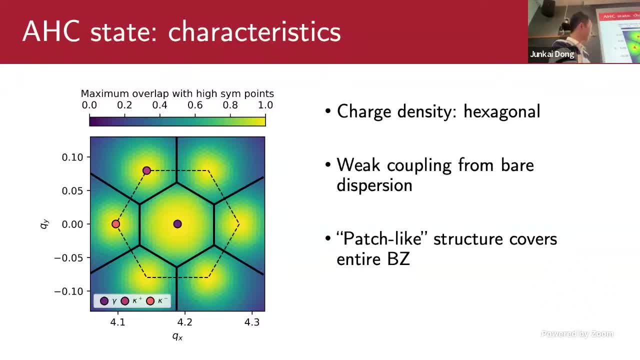 What I'm plotting here is the following: I take an arbitrary momentum Q, take the field orbital and I overlap it with high symmetry point orbitals such as gamma, kappa and kappa prime, And then I take the maximum of those overlaps. 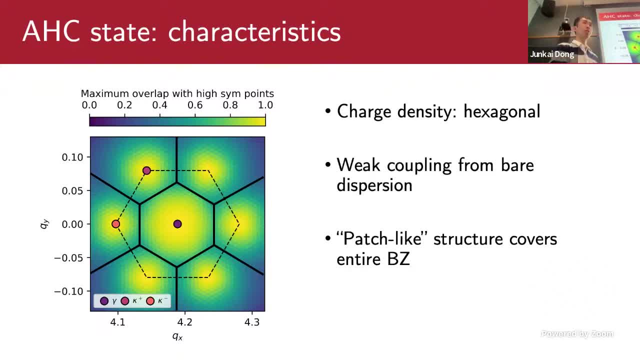 And you can see that at most of the, in most of the regions, the overlap is rather large. What this tells you is that, for example, orbitals around gamma, but not exactly at gamma, behave almost like they are, like the gamma electrons. 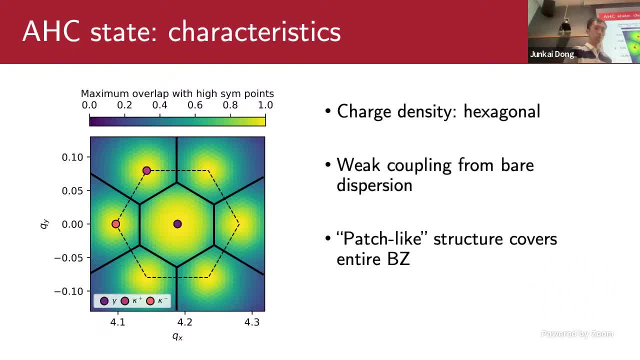 And electrons which are close to the kappa point behave very, very similarly to the kappa point electrons, and similarly for the kappa prime electrons. Yes, So should I be surprised by this? I don't have a good intuition here. Should you be surprised by this? 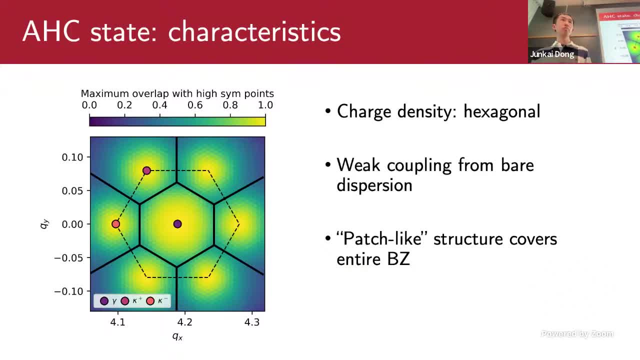 I guess so. so I guess there is the. there's also the statement that the wave functions at the different symmetry points are resolved to each other. Of course, you know, in rhombohedral pentalayer graphing, because you know, you have, you have many, many, many, many different atoms. 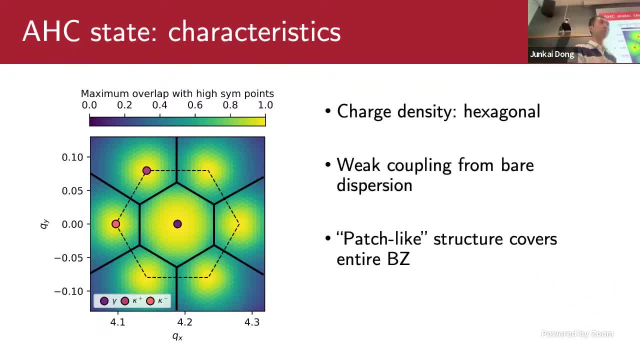 They will correspond to different. they will give you a spinner structure in the orbitals And you know the spinners at this point, and this point, indeed, look quite different. So is there? you know, if I had a different model or something different, would I expect, instead of getting these big patches, these small regions, or is this? 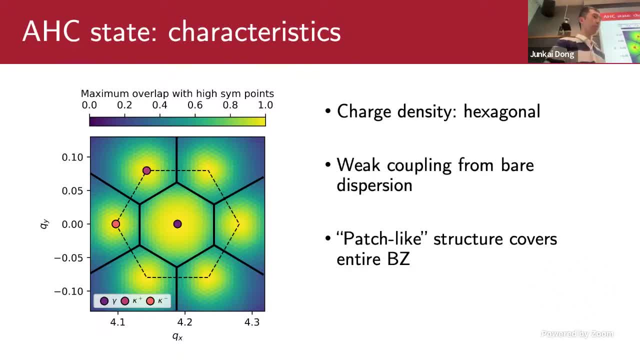 This depends. I think the intuition is that this depends on how fast the spinners move. The spinners change, right? If you know here this spinner is very different from the kappa point spinner, then you surely wouldn't expect this to occur. 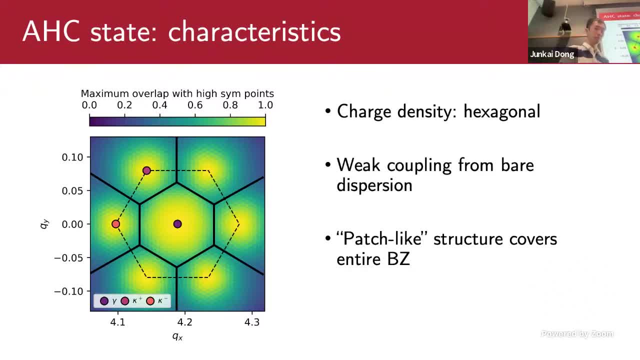 And it's actually the fork. I think our understanding is the fork interaction really tries to align the spinners from the kappa point and you know nearby points, And because fork interaction wants spinners to point in the same way, they create patches. 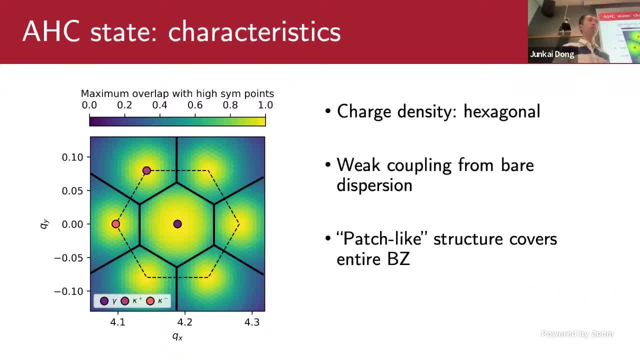 So to enhance the fork interaction, you want the spinners to look very similar to each other. Yes, Oh no, that's, that's me enhancing the visual visualization of the patches. Yes, Thankfully those aren't. yeah, it's not, it's not so discontinuous. 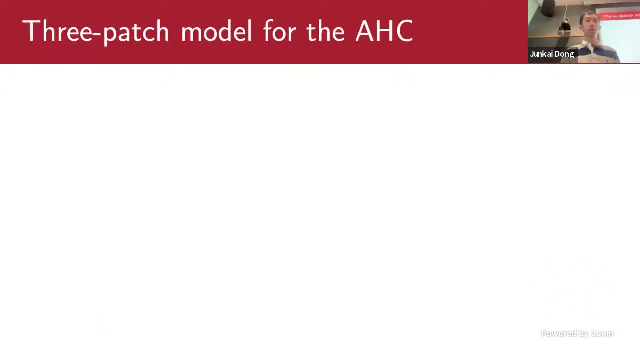 So this feature actually motivated us to construct a minimal model called the three-patch model. And the goal of the three-patch model is to explain why is this churn number one crystal even favored against, you know, churn number zero crystals such as the Wigner crystal. 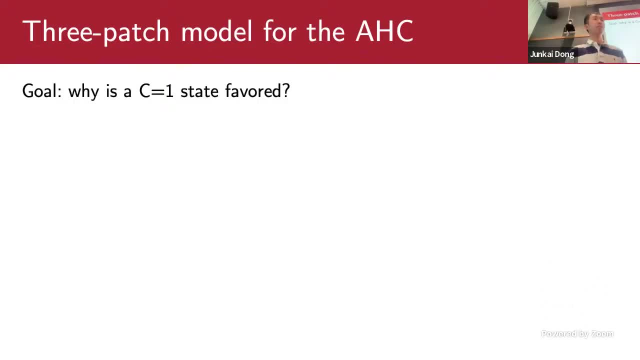 What we're going to do is to impose some assumptions, Some of which might not be, you know, a priori justified from from, from, from you know controlled approximations, But in the end you will see that this model works very well. 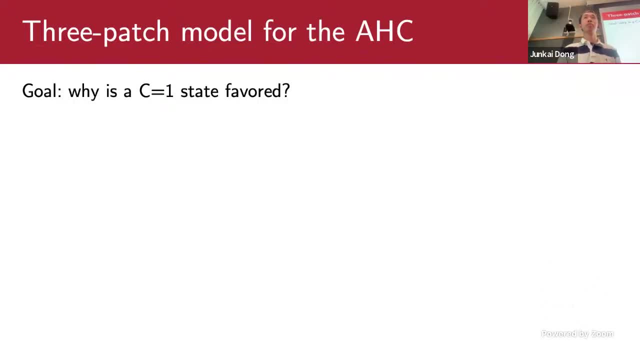 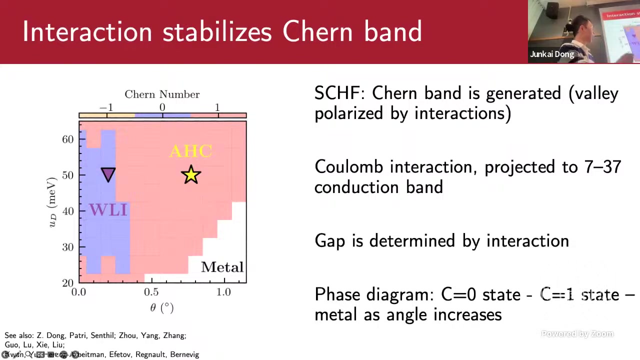 Yes, The value polarization. value polarization, that is right. But okay, how do you say this: No, no, no, no, no, no, So. so that is actually not the problem, right? So, for example, you know, if I go back to this slide- right, maybe, maybe a little bit even further back right, if I go to this slide- all of these electrons are value spin, polarized. 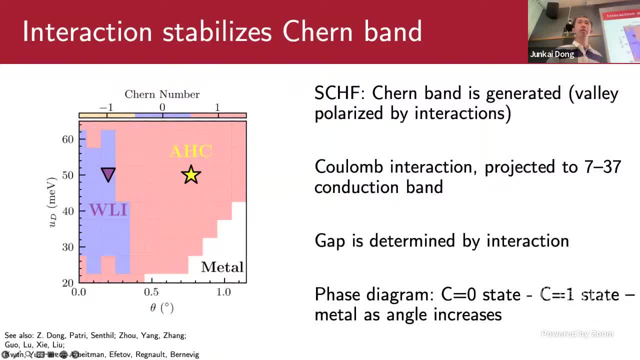 However, some of them still give rise to churn number zero, you know, in this case crystals, right? So there is a question to be asked, Which is: you know, why aren't all of these regions, which presumably the electron crystallizes, going to a crystal, which is, we are familiar with, the Wigner crystal? 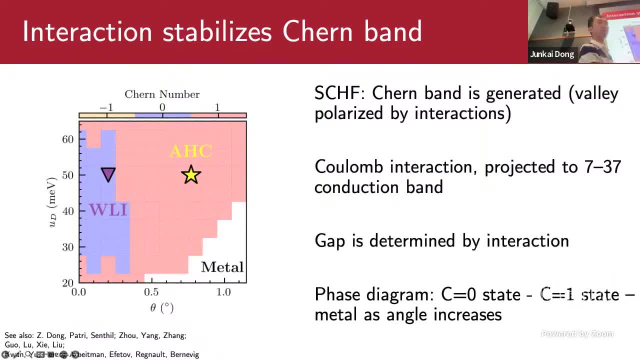 Why aren't all of these the Wigner crystal? Why do you get something which for which the churn number is not not zero? That's the question, Indeed right. So the time-revealed symmetry gives you the possibility for for for non-zero churn number, but it does not guarantee that it's going to be non-zero. 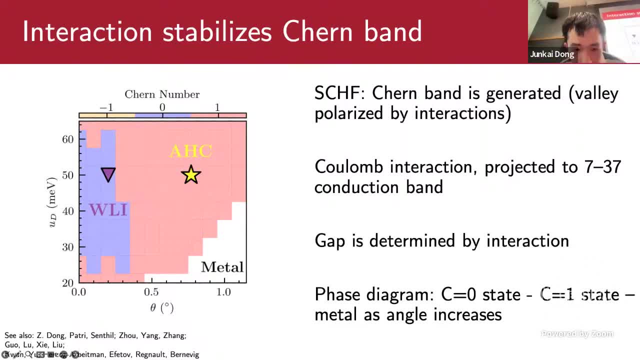 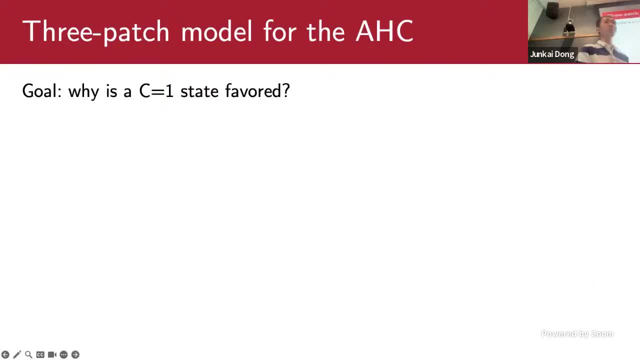 Yeah, Thank you, Right Going back. So what we want to understand is: why is? why does it choose the churn number one state right. So we're going to impose some assumptions. We're going to assume value polarization from the beginning. 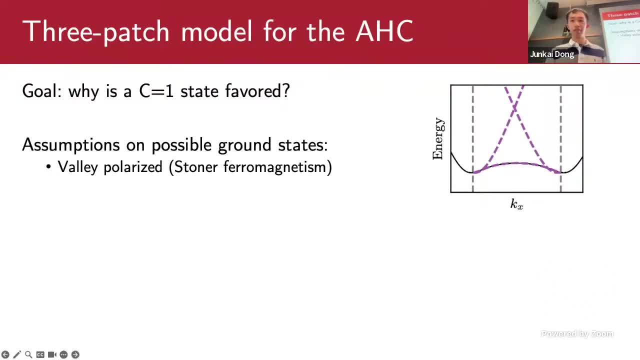 We're going to assume the figure of the ferromagnetism from a very large density of states, from the far, far bottom. We're going to do meanfield approximation and you know, just to make progress. And we're going to assume that the states are going to be translation breaking. 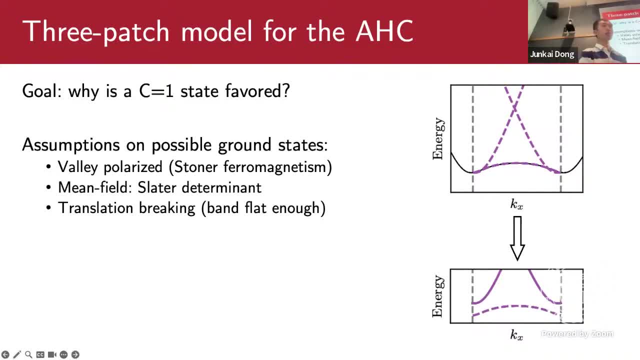 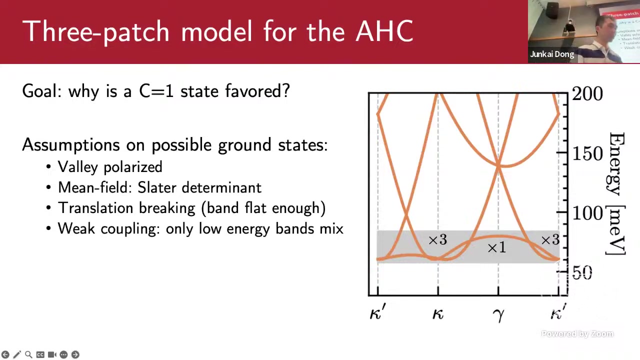 So this excludes the possibility of the competition with metals from our model. So if we do mean-joke calculations, we're not going to be responsibly taking into account correlations for the metals Anyway, and furthermore we're going to assume that a state is weakly coupled due to relations. 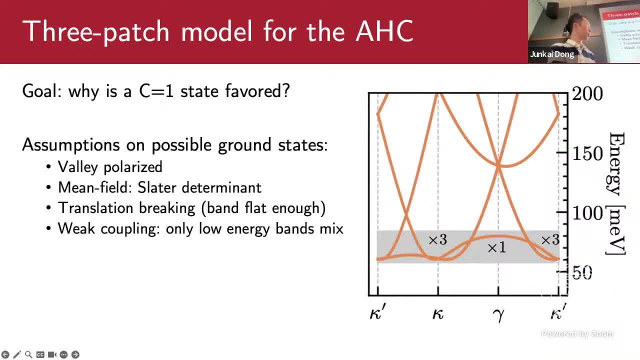 that we have alluded to above. Interactions are only going to mix low-energy orbitals, For example, this 3-fold degeneracy at Kappa point, 1-fold single band at the gamma point, and et cetera. 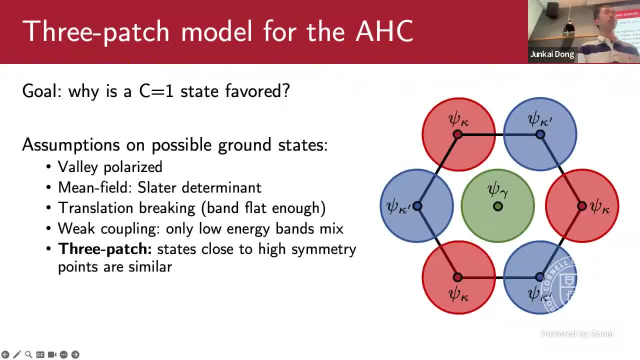 The most important approximation that we're going to make is this three-patch approximation, which basically says that states which are close to the high symmetry points look almost exactly like the high symmetry point wave functions. What this enables you to do is that you can basically delete 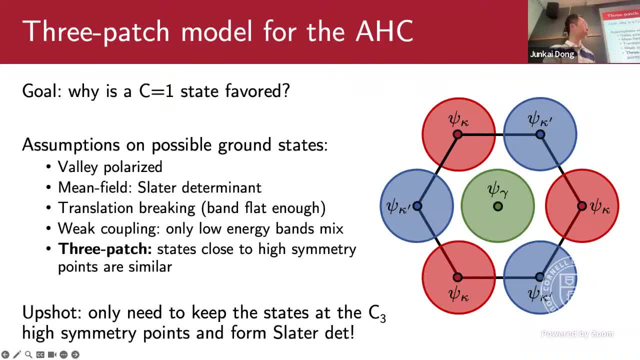 all the electrons in the Brillouin zone which are not at the high symmetry points, They get absorbed. This is like a very coarse-graining block spin approximation: All the electrons around the high symmetry points gets absorbed into the electron at the high symmetry points. 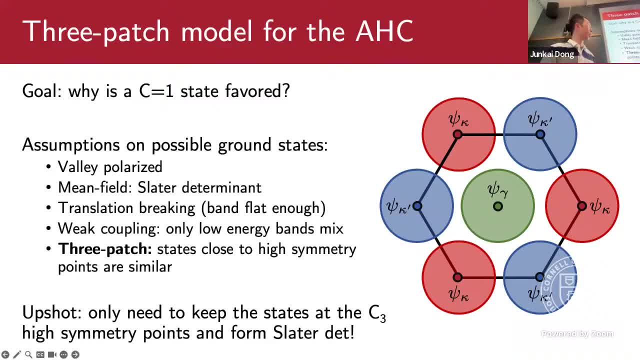 So how many electrons are there? There are only three electrons in states: One at gamma, one at Kappa, one at Kappa prime, and that's it. To make the discussion more explicit, we're going to construct the three-patch states. 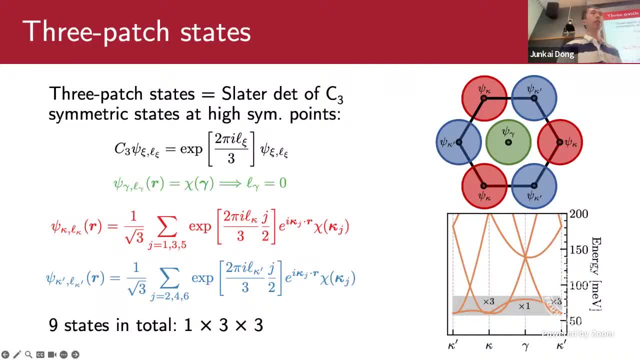 Given that we're filling electrons at the high symmetry points, particularly here, at the C3 high symmetry points, the occupied orbitals must be a mass form, representation of C3. These three which are labeled by the angular momentum L, So is the one at gamma, essentially. 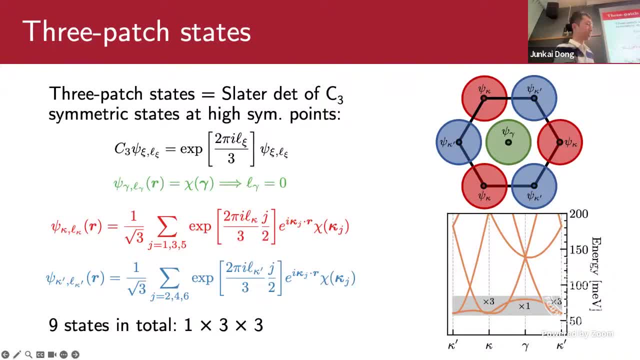 No, no. So, as you can see, the gamma point, in fact, is completely fixed among all of these three-patch states And we will explicitly show that gamma point wouldn't matter at all And we can use this property that the gamma point doesn't. 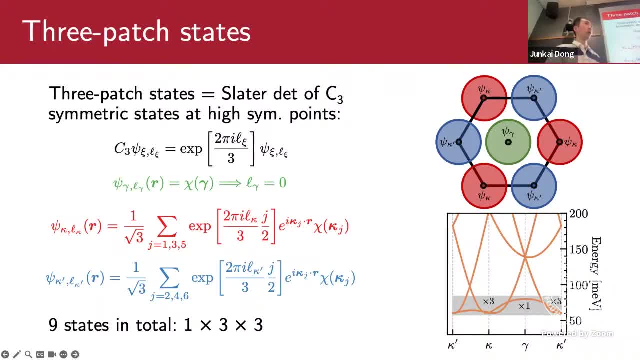 break translation symmetry to fix the C3 action such that the angular momentum at the gamma point is 0.. The Kappa and Kappa prime points are slightly more complicated. For example, for the Kappa point it can form a linear superposition of orbitals here. 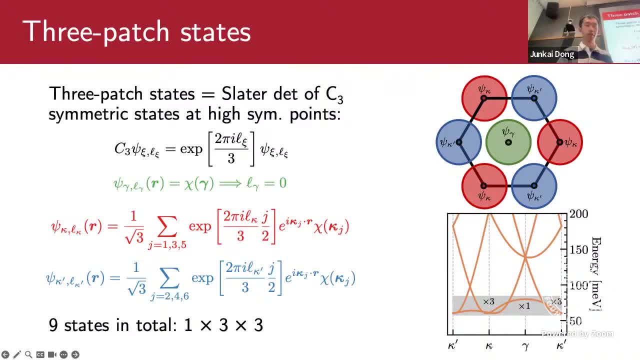 here and here corresponding to different spinner structures. These electronic orbitals are guaranteed to be degenerate in the single particle spectrum due to C3 symmetry. So, as you can see, the linear superposition takes this form, which means that these angular momentum 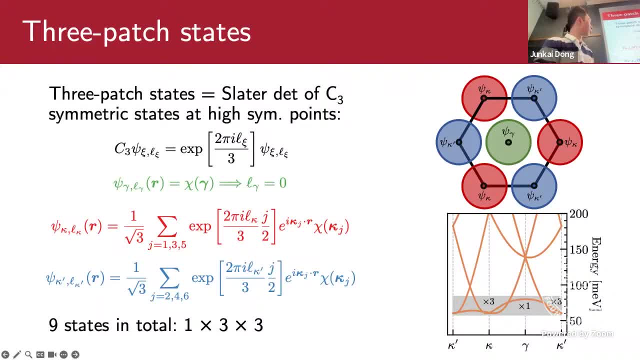 are really well-defined mod 3.. So for Kappa point, there are three choices that you can take: angular momentum minus 1,, 0, and 1, and three choices for the Kappa prime point as well. Thus there are nine states, in total one. 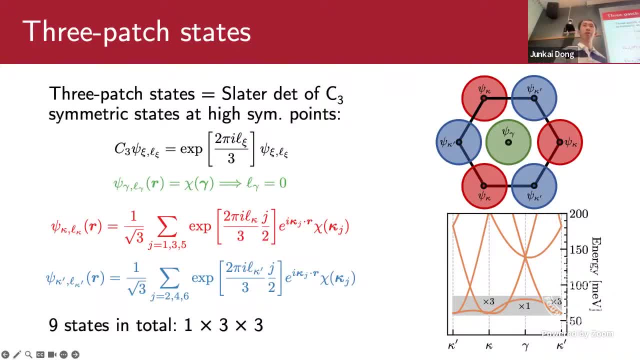 from the one choice from the gamma point. three from Kappa, three from Kappa prime. What? Yes, Here's a double question. This Kappa, what is the? It's the edge, It's the vertex of the Bruandau. 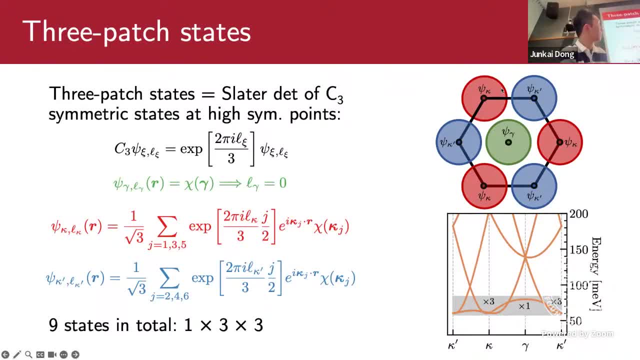 So Bruandau looks like this Right And the way of the Moray Bruandau, Moray, Bruandau. Very good. So this, what we do, is that we explicitly choose, we choose a Bruandau such that in each unit cell, 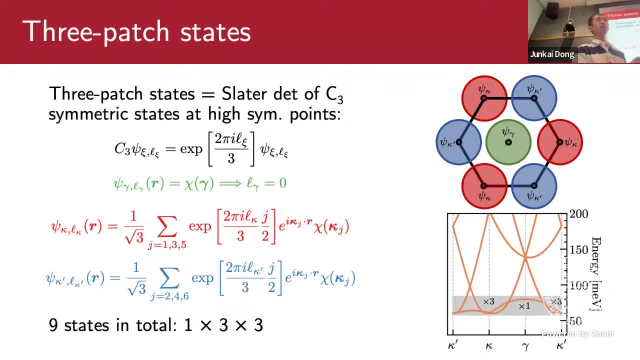 there is one electron. This will fix the size of the Bruandau. Yes, Sorry, In this phenomenological model the Moray does matter. In this phenomenological model the electronic density matters. So If you use the one electron per graph of the Kappa layer, Moray, 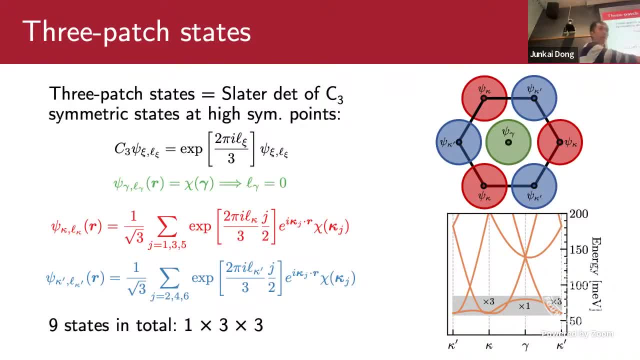 pattern. OK, So all of these calculations, You should think you know there is no Moray what so ever. Yes, What you do ask is what about that whole Moray pattern you're trying? Are there lots of electrons per unit cell of that Moray pattern? 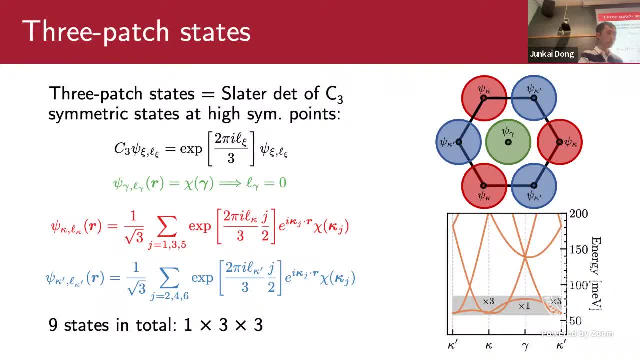 Are there a few electrons? Are they equal? This is a great question. In fact, you know we don't assume that those things will be commensurate in this case. Are they far apart? Are two of these? Can we know that this pattern has nothing to do with that one? 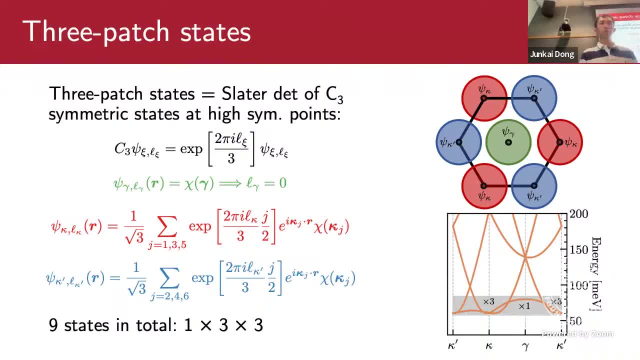 because it's so much different than that. This is a great question, In fact. so what I want to say is that I don't know the answer, because we have not. We have just completely thrown away all Moray effects in this model. 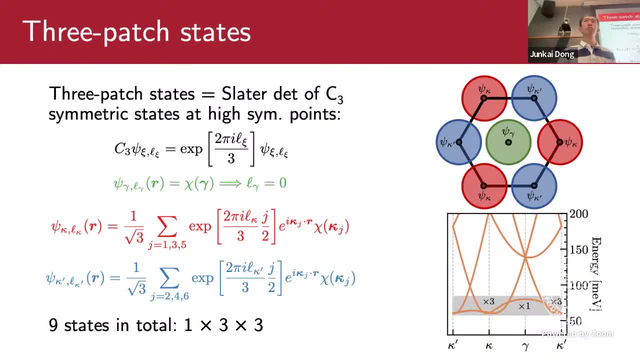 I mean to presume the experiment. How might they have? Oh, in the experimental setup, you know, those are very much, They're very much on the same order, They're, assuming Almost exactly the same. So at so the 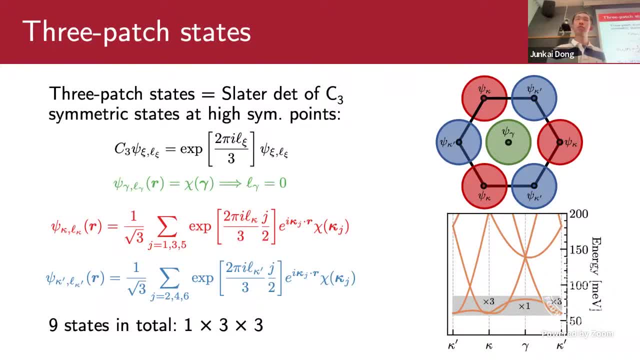 It's less of a push to the bottom, but the number is that kind of Moray. Oh, no, no. The number you can tune by hand. The number of electrons within the graphing stack, you can tune by hand by controlling the voltages. 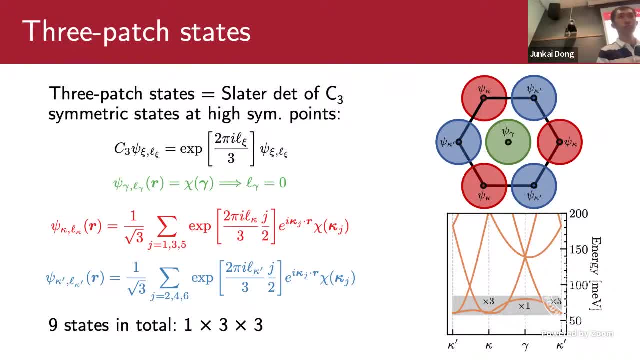 And then they've seen When they're near the density of the Moray pattern. Yes, Even though the Moray thread doesn't match. That's what we are saying. yes, Because? But can you agree with this? I completely agree, which is what we have said before. 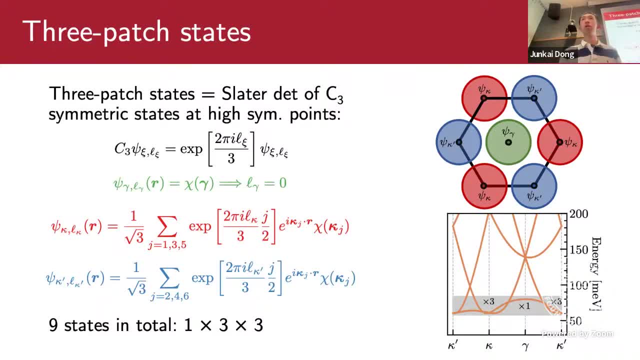 So in those cases there is a competition between the length scale. When they are far, They're far apart. There is a competition between the Moray. The Moray wants to impose one translation breaking pattern: The electrons by themselves probably. 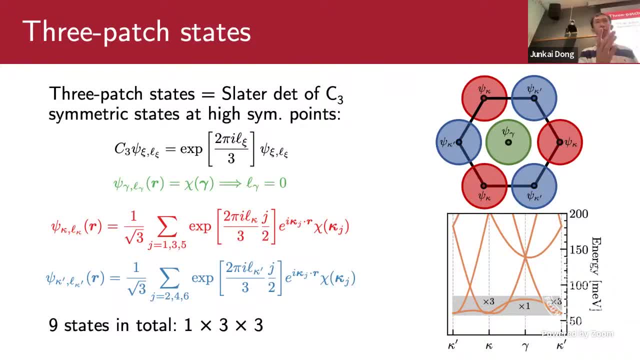 want to impose another translation breaking pattern And this competition we have not studied before And the experiment, if they didn't, to be this far away from the Moray length. it doesn't behave the same way, Or they just want to, because that's. 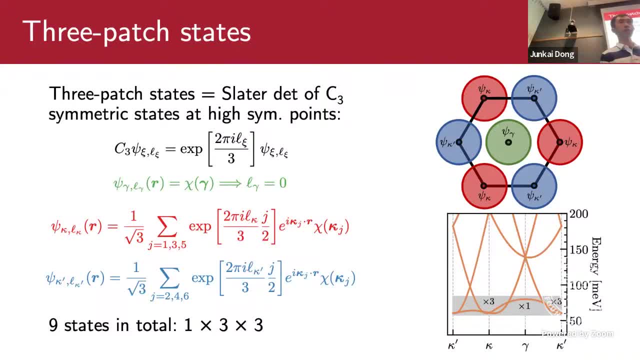 why they thought it would be. You know, if the electronic densities are very, very far more So if the electronic densities are very, very large, the other effects are going to come in. For example, the dispersion is going to become super large. 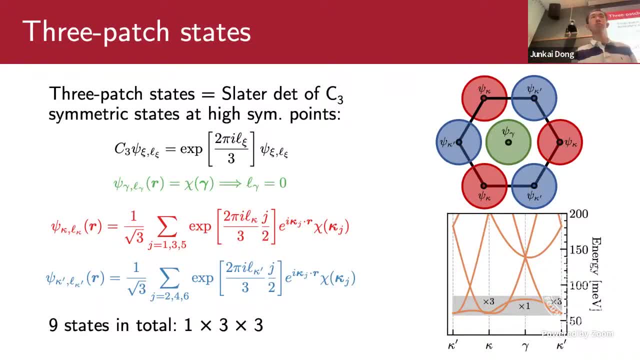 quite different, but not crazy At one half, you know. so if you lower Right At that point, I think the claim is that they form a composite Fermi liquid whose translation breaking pattern is still set by the Moray. 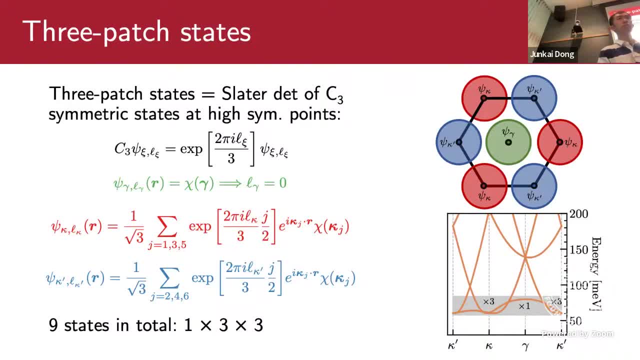 Was all of this motivated by the tall plateau and fractional building? Was all of this motivated by No? What was motivated by this? The motivation of all this was to even get to just understand the possibility Of getting a Wigner crystal. that is topologically non-trivial. 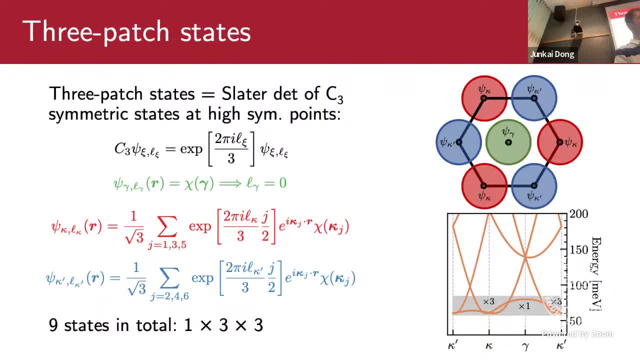 Oh, so this part has nothing to do with any experiment. No, no, no, no, no, no, no, I might have, I might have. What was the experiment that motivated this? that must have a feeling. The wait, sorry, sorry. 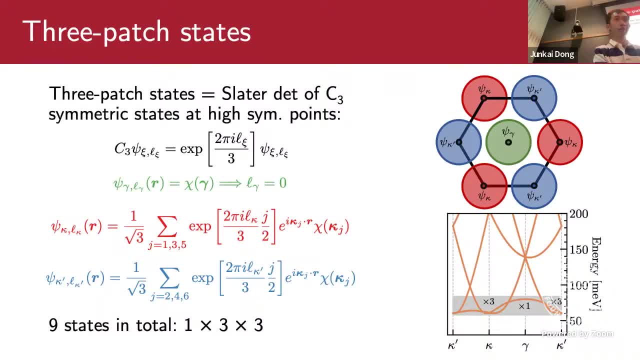 The experiment motivated the first part of the numerics. This part, Yes, The first part of the numerics motivated the second part of the molecule. What was the feeling in the experiment? Was it some fractional, commensurate, fractional building of Moray? 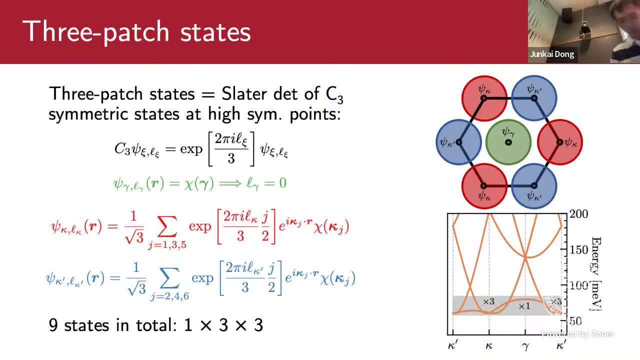 Right. so let me try to understand the question, because I assume that I have incurred some confusion right here. So you're asking: when does the turn insulator, the integer turn insulator, occur in the Moray experiment? Is that the right question to answer? 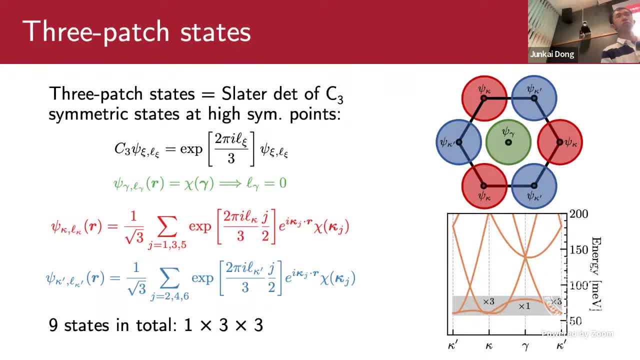 It just sounds like there's a lot of debate about whether it's your periodic, whatever your periodicity, that you're assuming here that you have one electron per some periodicity. Yes, What is the relationship between that and the Moray you could get? 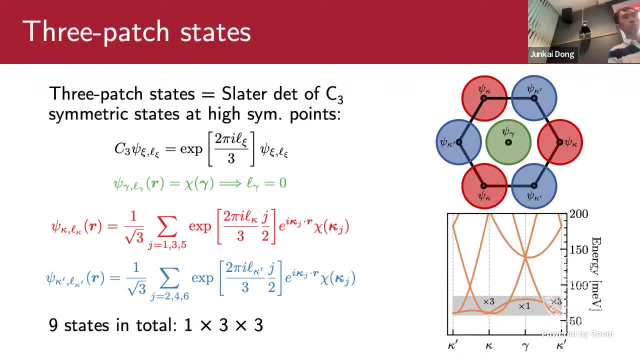 There is some confusion about that, Right. So I want to know, in the experiment that motivated all this adventure, what was experimentalist's note of feeling? And there was something incompressible, classical-like or something sharp Right In the experiment that motivated a lot. 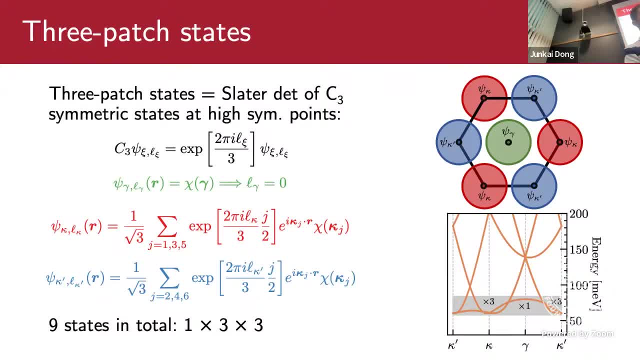 of theoretical investigation. I just want to know what the feeling was. Oh no, That feeling is one, That feeling is exactly one. Yeah, Oh Yes, One electron per Moray. Yes, Yes, OK, So why do you want to insist that this periodicity that? 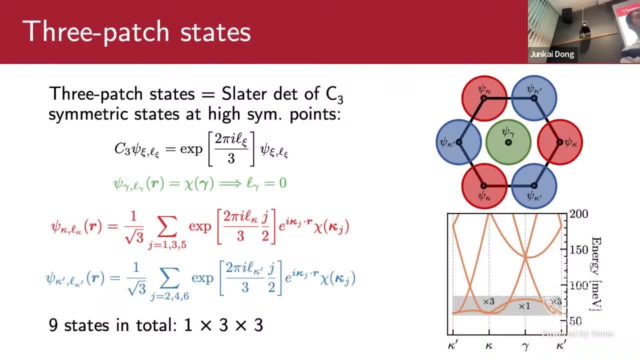 is exactly the same as Moray. periodicity has nothing to do with Moray. You know how to say this. Moray, as we have said, right, You know, Realistically realistic consideration is one thing, Right, Realistically, this system might just. 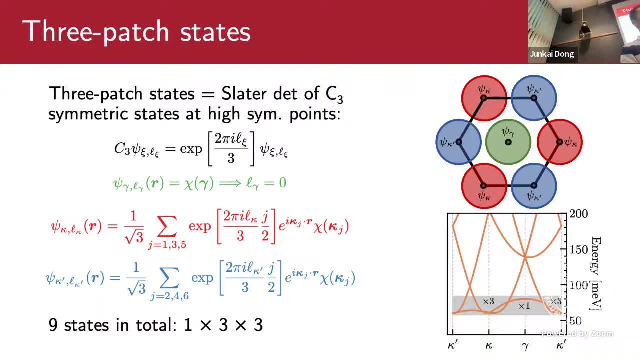 need a Moray to form a chain insulator which we can debate on. On the other hand, the urge to understand why we can even see something like this without Moray in numerics is something that we are trying to address. Yes, 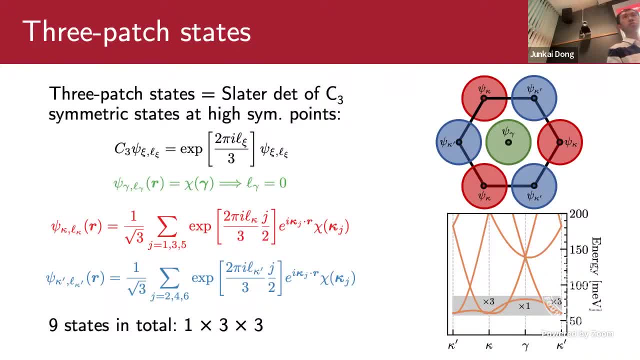 There is a thing. OK, So you're. So you're saying that the theory using this Hartree clock and things like that gave you Moray even without a. It gave you this insulating state Even without a Moray pattern. Yes, 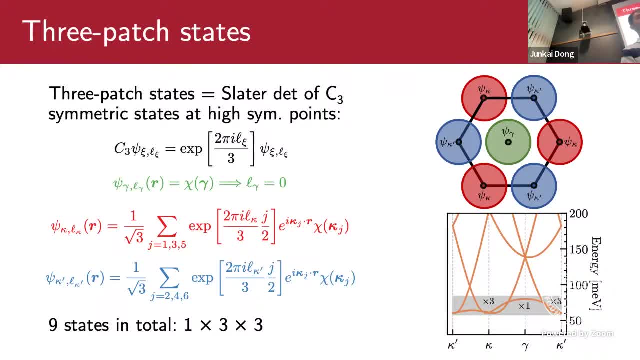 And now you're trying to understand why your Hartree clock gave you this answer Yes, And this is the reason the Hartree clock is giving you that answer Yes. And if Yes, The experiment also made use of the Moray. good for it. 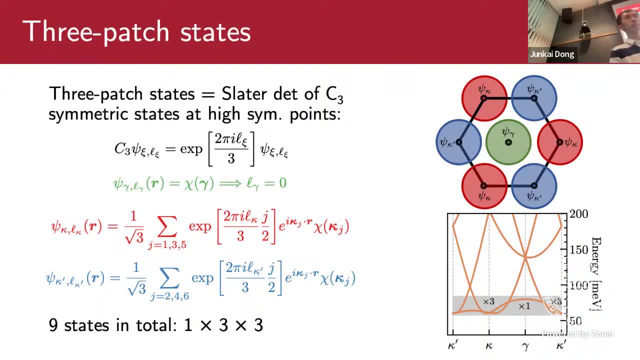 But it doesn't matter. Yes, But the problem is in Hartree clock. the periodicity that we can get has no reason to have any relation to the Moray periodicity. No, Not at all. Not at all. Completely agree. 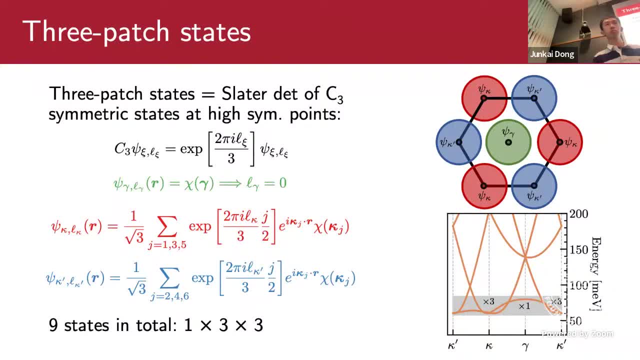 So the experiment was just some inspiration. You shouldn't try to relate this to the experiment. Yes, Almost exactly. No, Yeah, You know, If the experiments does have Something to do with this, Then we are going to be ecstatic. 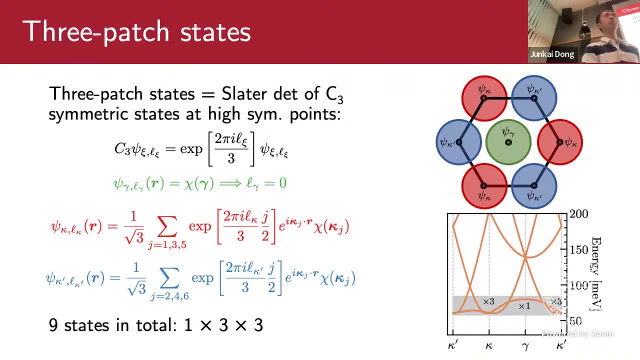 Yeah, Yes. Well, Actually, About this Hartree, Yes, Yes, Yes, Great, All right, So on with explaining why the translator appears in our numerics Right. What this simple modeling? This simple modeling might seem very minimalistic. 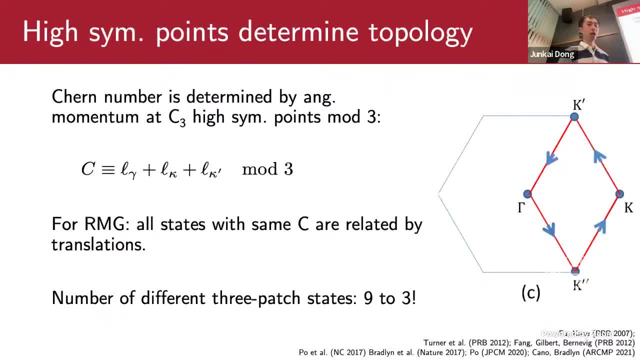 But it does not lose all the flavors of. It does not lose track of all the global data. In fact, there is a perspective called symmetry indicators. Basically, when you have some symmetry, such as C3,, you can only look at orbitals occupied. 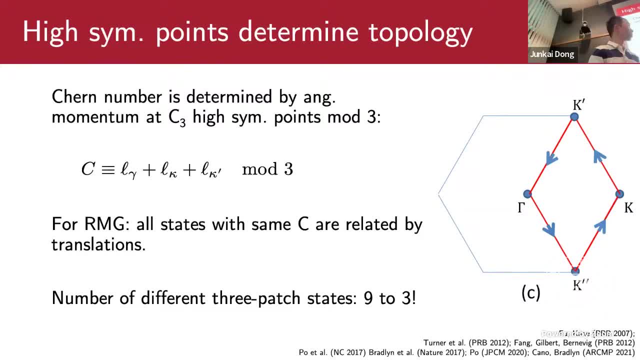 at those high symmetry points- gamma, kappa and kappa prime. And what Bernevik and folks have proven is that if you add Those angular momentum together, you're going to get turn number mod three. And for the model that we are considering, what's going to happen is that all the states 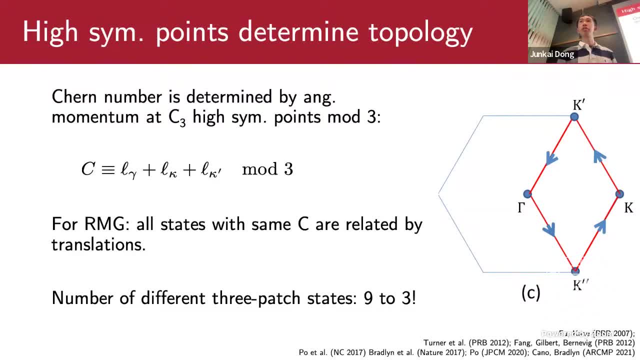 with the same turn number can be related with different translations And this will reduce the number of different three patch states from the previous slide of nine to three, corresponding to the three turn numbers. C equals minus one, zero, one mod three, So yeah, 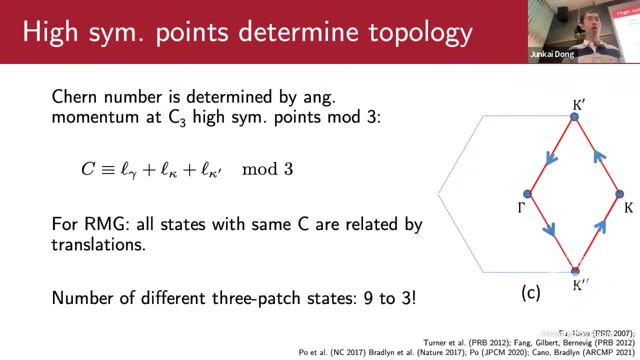 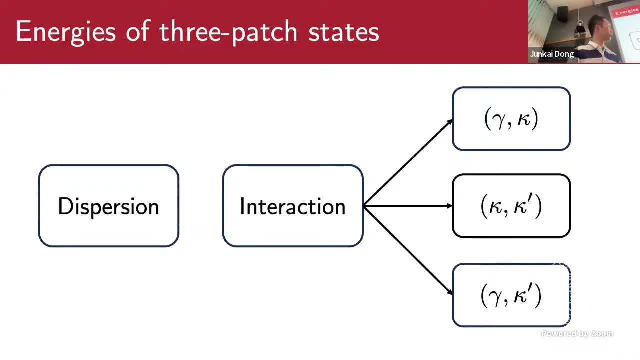 Now we're going to evaluate different energies of three patch states of different turn numbers. There are two parts to this. There is a dispersion and interactions corresponding to different electronic pairs, But not all of these care about the turn number. In fact, there is only one term that cares about the turn number, which is the interaction between: 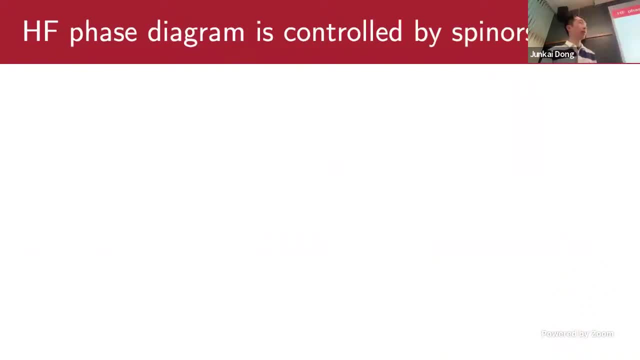 kappa and kappa prime. What's going to happen is the following: We're going to evaluate the interaction between the kappa electron and the kappa prime electron using the Hartree-Fock approximation. So the Hartree-Fock approximation breaks the energy into two terms: the Hartree term and 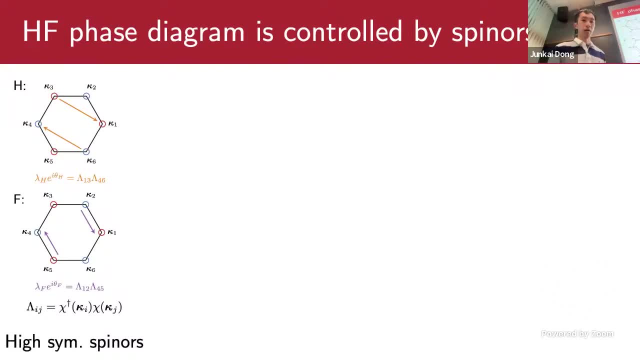 the Fock terms. Each of these, the turn number dependent part of the Hartree and Fock, are controlled by two scattering processes only. So scattering process from kappa three to kappa one and kappa six to kappa four, And there is a similar one for Fock. 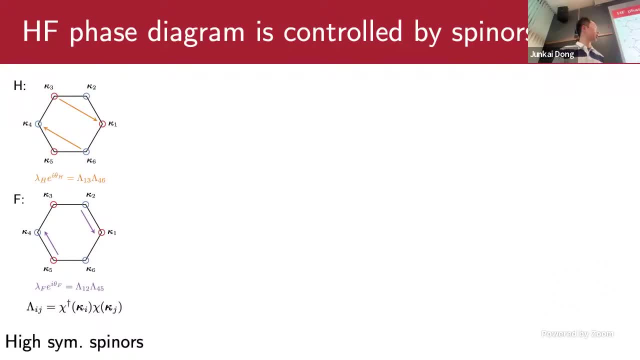 What's particularly important about these scattering processes is their amplitude, Basically a combination of form factor. When you calculate the amplitude of this process, you have to overlap the spinner at kappa three to a spinner at kappa one, and you know six to four. 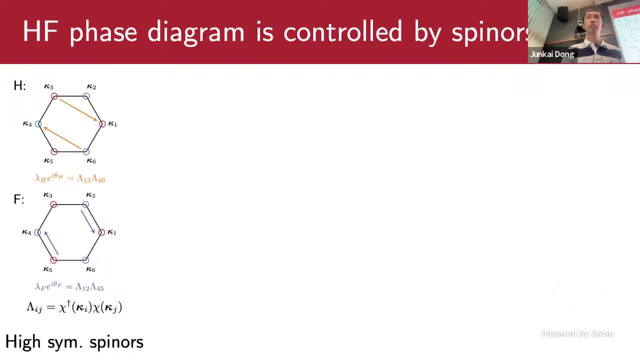 And you multiply them together, I'm not sure I really understand the weak to strong transition between. That's right, That's right, But I'm not sure I have enough knowledge to make that comparison. Yeah, Yeah, Yeah, That would be really cool. 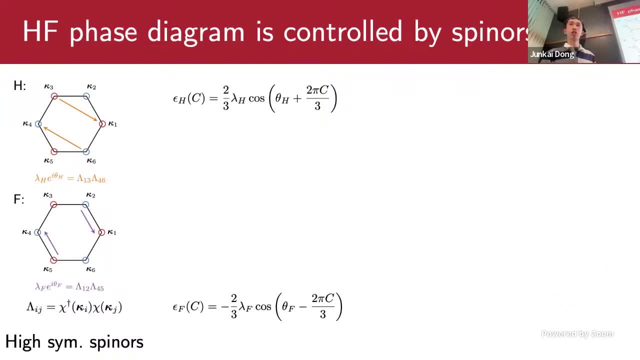 On the other hand. so what's going to happen is that, if you just look at Hartree and Fock terms alone, that it's really the angle of these scattering amplitudes that determine what turn numbers that they favor. So Hartree favors one turn number due to one angle, theta H. Fock favors another turn number. 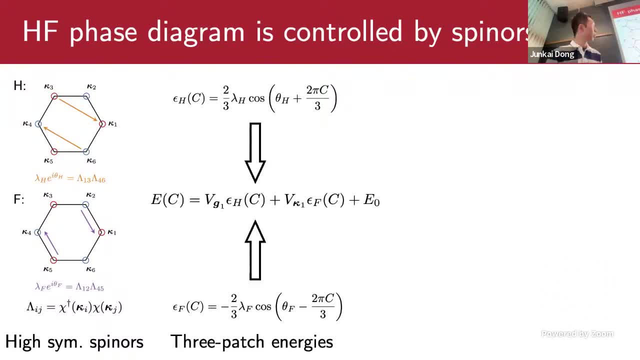 due to this factor. This phase factor is theta F, But in reality, the energy of the three patch states is going to be a weighted sum of those two plus a turn number, independent turn. However, what's going to happen is that in the phase diagram, as a function of theta H, 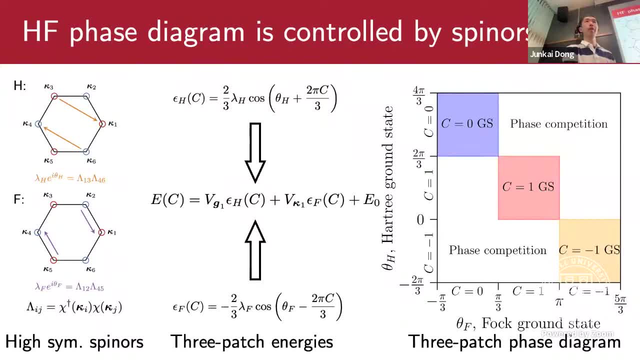 and theta F. sometimes you can get frustration-free regions in which both the Hartree and the Fock favor the same turn number, At which time you can guarantee that your state has a certain turn number. So for example, for Hartree, between 0 and 2, pi over 3,- all of these regions favor turn. 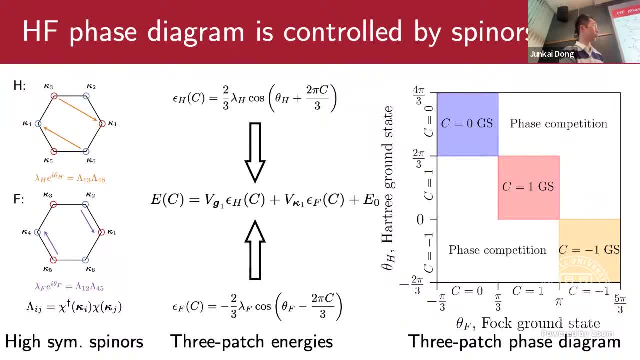 number 1 for Hartree, And when theta F is between pi over 3 and pi. all of these regions also favor turn number for Fock, So when they overlap you can guarantee that the ground state is turn number 1.. Hopefully at this point we have convinced you that you know the same thing is true. 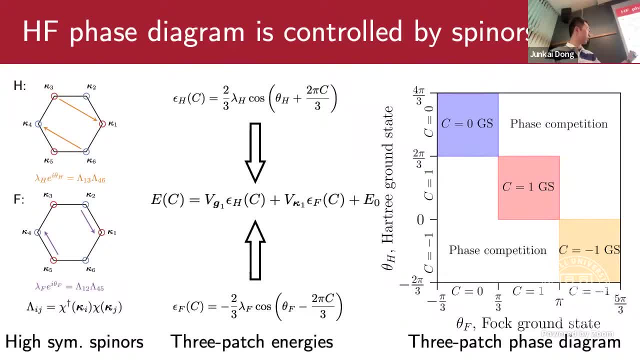 here. The spinors determine the form factors. The form factor determine the scattering amplitudes. Scattering amplitudes determine energetics. So the spinors are quite important. Given the time, let's try to do this very quickly. 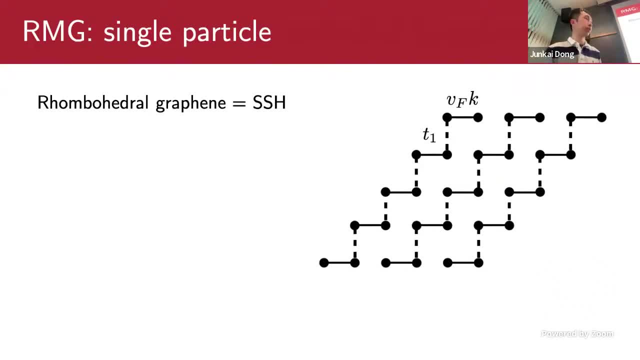 We need to find out the spinors for rhombohedral multilayer graphing. Rhombohedral multilayer graphing is basically an SSA chain with Hoppings, Vfk in plain and T1 out of plain, And SSA chain has a chain. 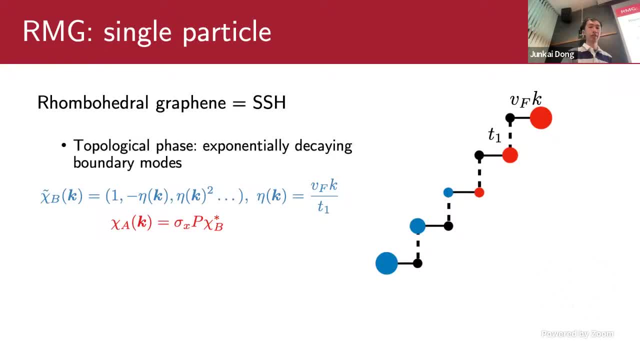 As a topological phase, when Vfk is less than T1, and you have exponentially decaying boundary modes living on the two sublattices, one on the B sublattice living on bottom and one living on the A sublattice on the top. 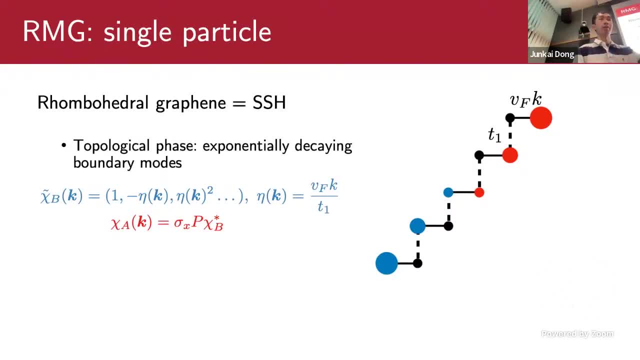 And they're going to be mixed together if there is no displacement field separating, which gaps them out. However, once you apply a displacement field, you're going to find that the spinner content of, for example, the conduction band is basically described by this spinner alone. 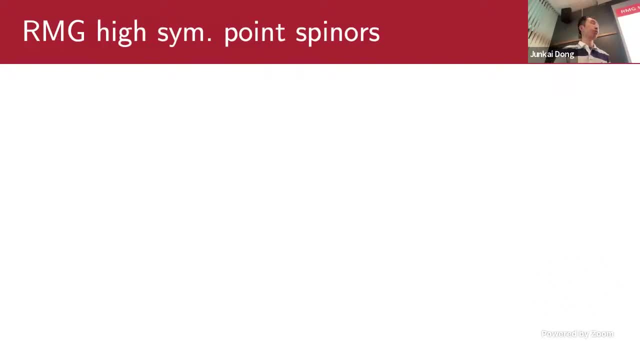 Well, now we're going to produce these spinors. We're going to choose a Brillouin zone corresponding to one electron per unit cell, And what you're going to find is that the spinors at all the high symmetry points is constructed. 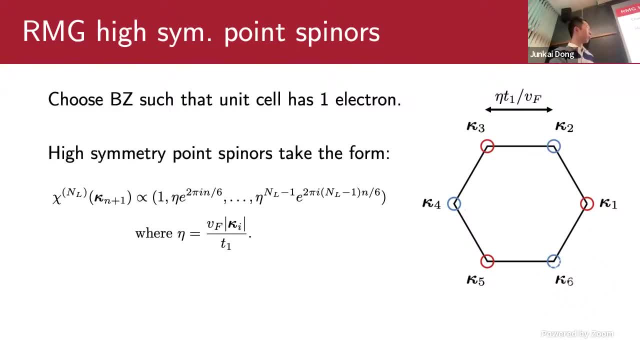 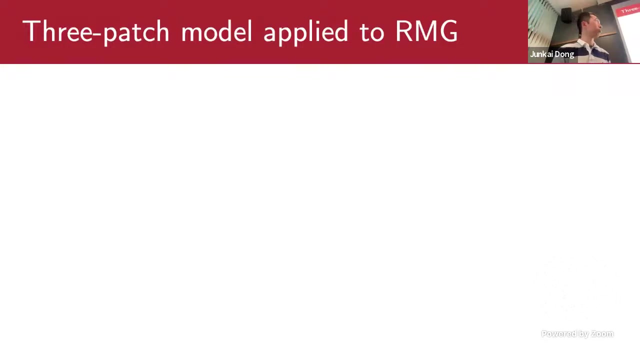 It's controlled by this number called eta. Eta basically describes how large the Brillouin zone is. So eta basically is how long this separation is And physically it can be tied to the square root of the electronic densities. Now we're going to apply the three-patch model to Rambler-Keter multilayer graphing and 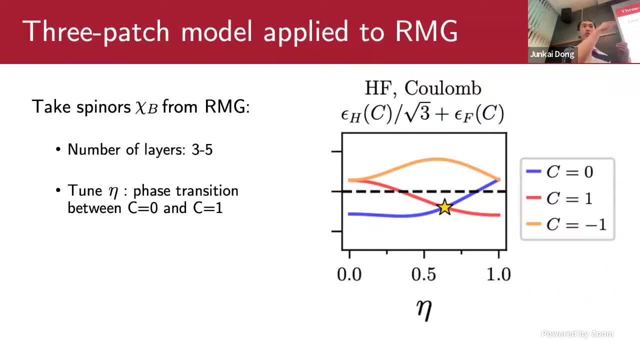 you take a certain number of layers, By which I mean that you take the exponentially decaying spinner and you cut it off at certain components. What you're going to see, the phase diagram, is very, very similar for three and five. So this is three layers. 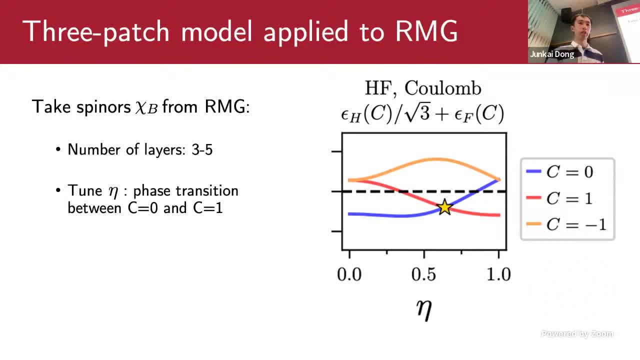 You tune eta, which physically corresponds to your tuned density, And there will be a phase transition between the sequence zero state, below eta at 0.6 or something, and above 0.6.. It's basically turn number one. Let's skip this. 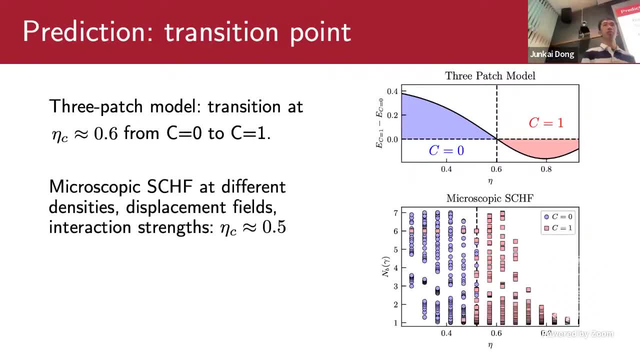 So, given this transition, you can also compare it to the Hartree-Fock numerics that we have run. So this is the apex of the argument. We run self-consistent Hartree-Fock at different electronic densities and different displacement fields, different interaction strengths, to see what is actually the parameter that drives. 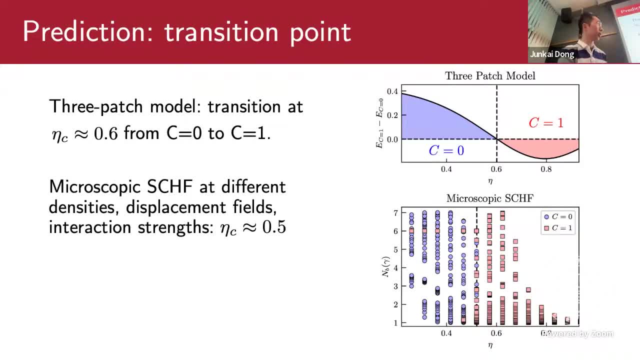 this transition And what you can see is that there is a pretty clean phase diagram as a function of eta. above, eta equals 0.5, or something like that. All the insulators that you get are turn number one, below which most of the insulators have. 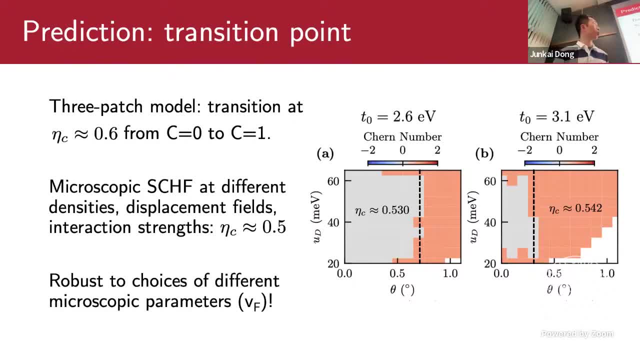 turn number zero. You can also tune. you know you can also tune microscopic parameters, such as you know the hoppings. You can tune hoppings by like 0.6.. You can also tune microscopic parameters, such as you know the hoppings. 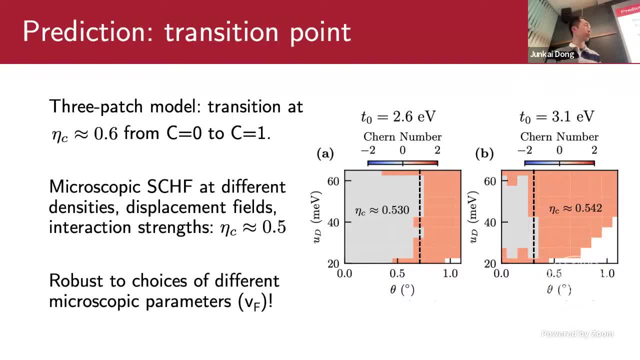 You can tune hoppings by like 0.6.. By 20%, And if you convert the phase boundaries to eta you find that it only moves on something like 2%. So I think what the three-patch model has identified is this crucial tuning parameter. 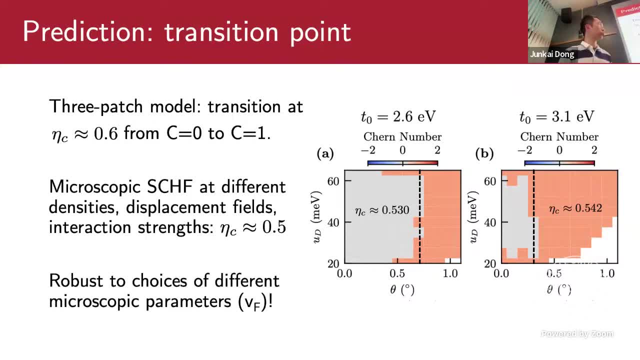 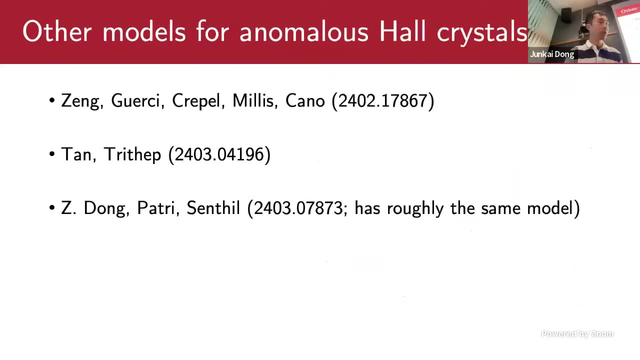 called eta, and this has been revealed to be true in microscopic numerics as well. So by this, I think we claim victory over explaining our own numerics with this very simplified model with three exact fonts. I'd also like to highlight some other models that 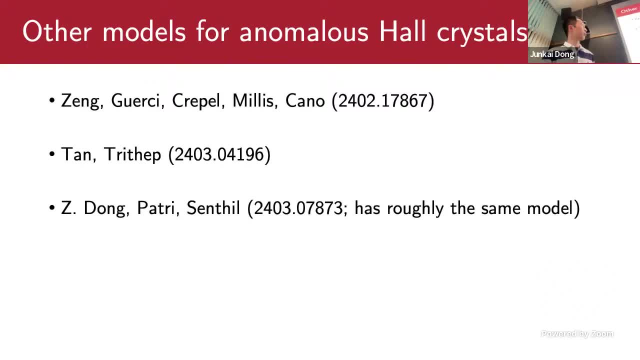 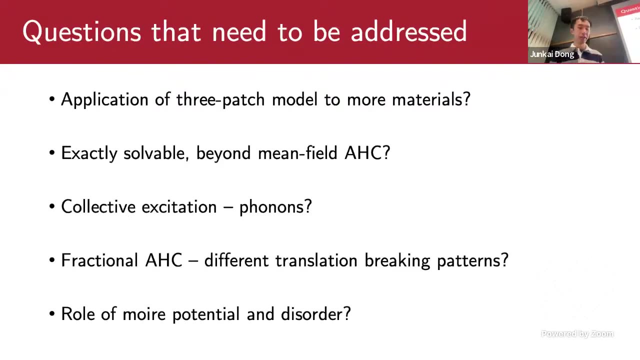 also have models for anomalous Hall crystals. There's one paper from Jennifer Cano's group, there's one paper from Fritz's group and again our old friends at Central came to almost exactly the same model as us. Given this development in anomalous Hall crystals, there are many questions. 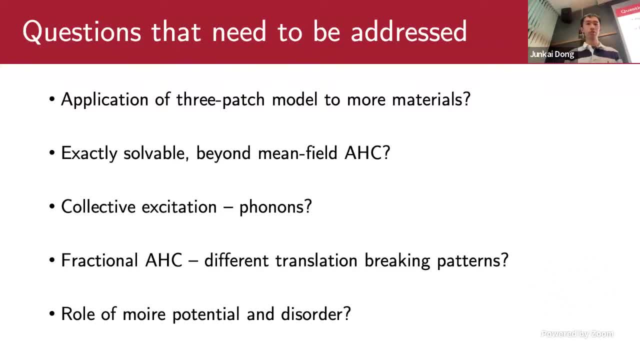 to be addressed? Can we apply this three-patch model to more materials? Can we do something beyond mean field that is exactly solvable or most likely analytically solvable? And what about the phonons in this topological crystal? Is there a possibility for fractional anomalous Hall? 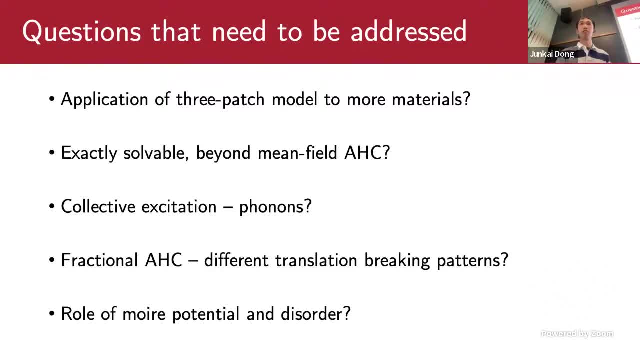 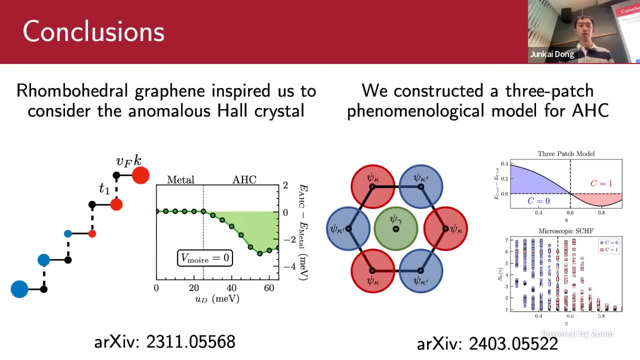 crystals and what is the role of Moray potential and disorder? With that I would like to conclude. the modeling of this very exciting experiment in rhombohydrography has inspired us to think about the state of anomalous Hall crystals and we have built a three-patch model, a three-patch phenomenological. 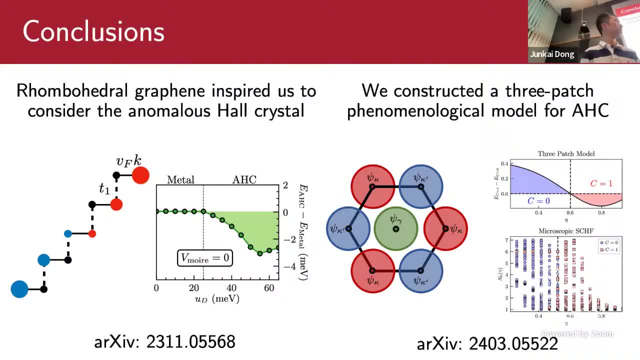 model for the anomalous Hall crystal that we have found in our numerics and it is decently successful With that. thank you very much. Questions Answers- Any questions about the model. Questions Answers: Questions, Answers, Answers. 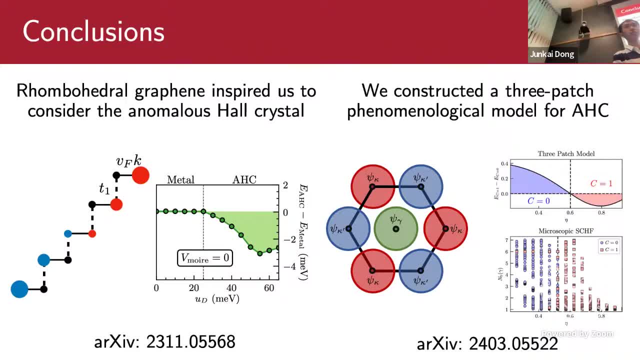 Questions, Answers, Answers, Answers, Answers you just make I'm not going to do this, Whatever, yeah, Yeah, When it just seems to move density to the ring: No, so this is Sometimes why you have to break that. 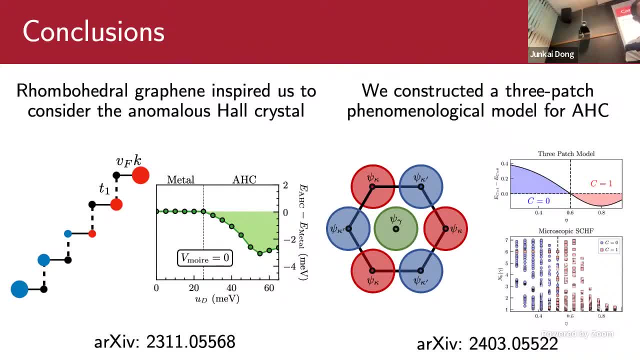 is to get a right piece, Right, right, right, No, no, no. this is a fantastic point in which this is: you know, we want to study this, but you know this question in particular, but I have not found a very good way to phrase. 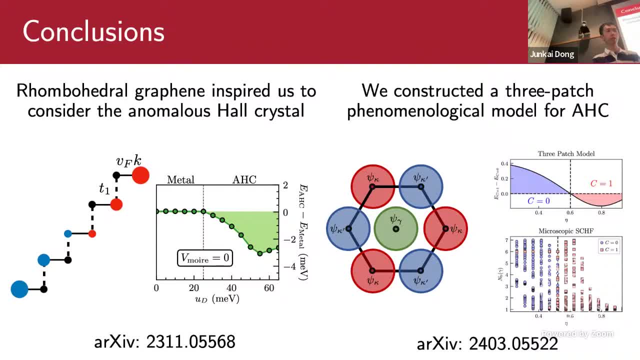 to probe the problem. So probably one way to say this is the following: right, You know, let's say you have some particular electronic density and you know at which you get the anonymous Hall crystal, Then you dope it, dope holes. 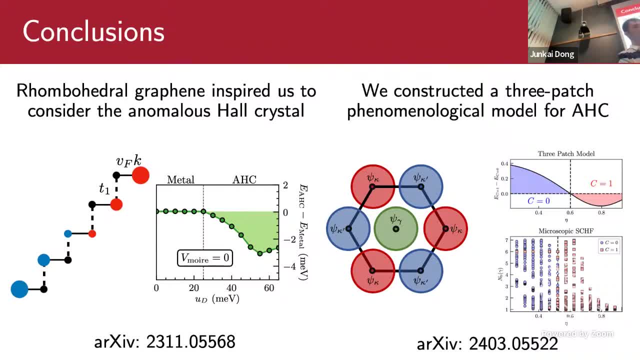 you decrease your electronic density At, for example, filling, you know, one third, let's say, Let's say one third. there are two possibilities. One: you keep the density, the translation breaking pattern, unchanged and you form a fractional state, most likely. 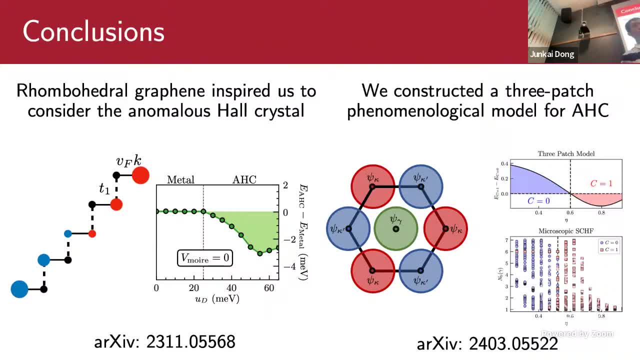 And the fact that you know you can just expand your unit cell and form an integer filled state. There is non-trivial competition between those states. So, But if the only thing that's setting the data is the identity of a lexon? 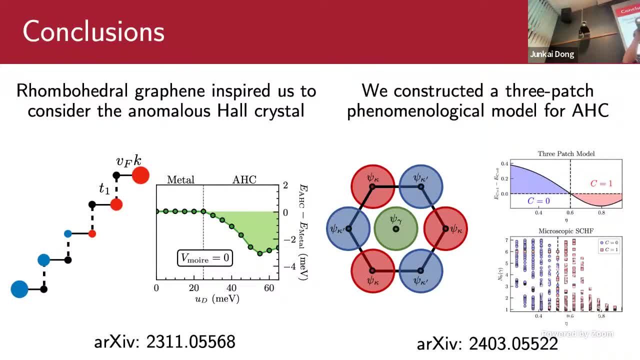 Yeah, If the identity of a lexon, how can a student ever fractionally build? That's what vegan crystal is supposed to be. Vegan crystal's purity is the only set by the density. If you really want it, it's this one name. 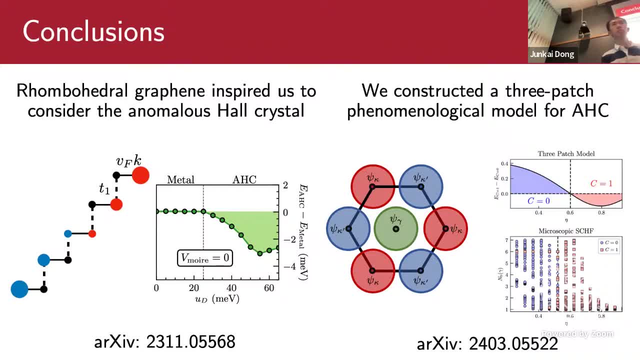 But that's semantic And if, as far as I can tell, what you have is, you know value and density are very, very, very important. So it's very, very important: valley polarized charge density wave state which the valley polarized state on by valley polarizing. 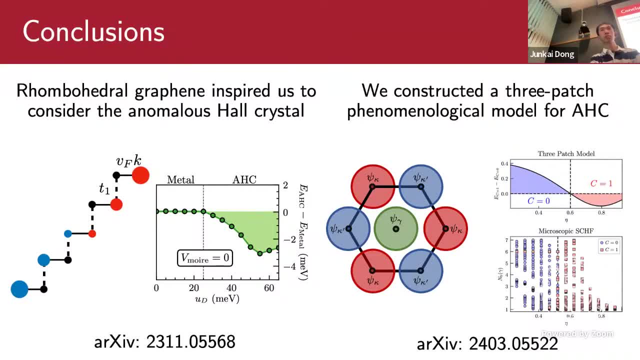 side can or may or may not have turn number right. yes, and. but you, in your second paper, you indeed treated translation of symmetry breaking totally separately from the turn number to fix, yes, yes. so as far as your chart of translation of symmetry breaking is concerned, you're getting it. 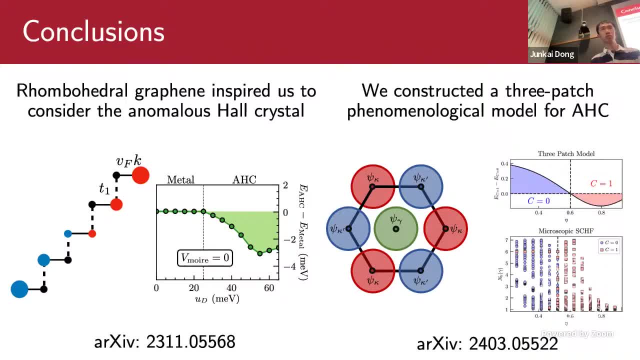 out of higher sensibility of nesting, which is what turns into basically yeah, yeah, no. going back to the question, it's, you know i don't. although i agree with the sentiment, i do not know if there is a is. if there is a precise argument for which, you know, one can argue. 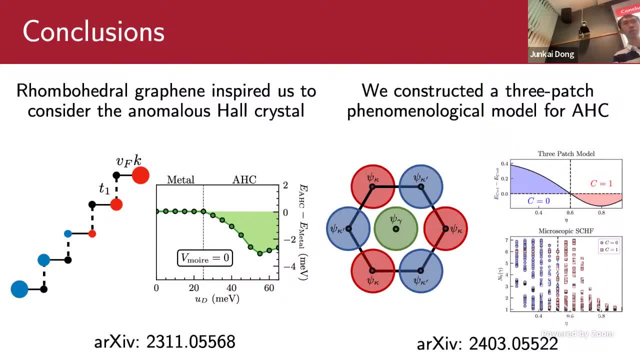 that it's always going to be the integer state rather than the fractional state. um, in fact, we have been looking for this argument for a very long time, um, without success. so, yeah, if there is no way to set the, uh, yes, you have to define the periodicity as the lattice. 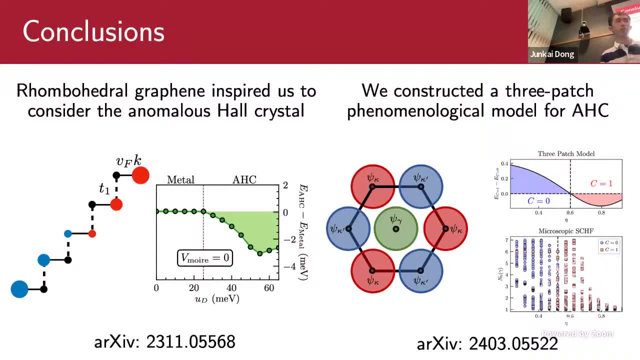 i agree, i agree. so, basically, my question is right. you know, at a particular, at a particular electronic density, there are two possible states: one fractional, the other integer. right, you cannot talk about that, right. so right. so electrons will spontaneously break translation symmetry to form a lattice, and the lattice, you know if. 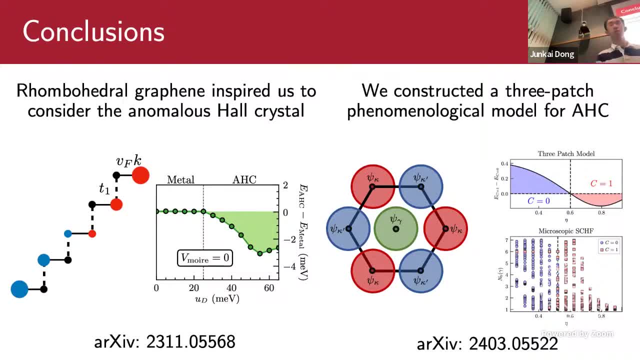 you calculate the electronic density, electron number within each unit cell of that lattice born by electrons is fractional. that's what i mean by fraction. i mean, shown by your- uh, original calculations, new calculations, that that there is a tendency, uh, there's this enhanced susceptibility, to take it forward. 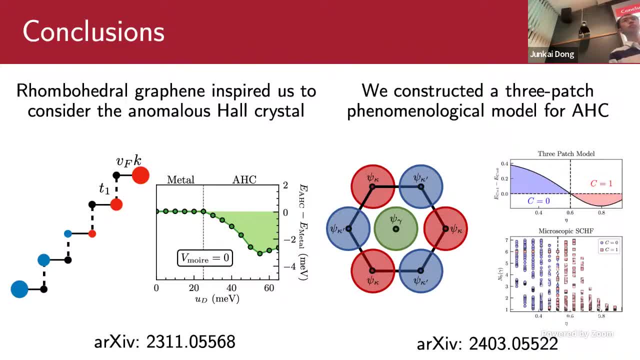 for a uh, for a 10 like state: uh uh, uh. with the periodicity of the form that maybe the experiment is making use of by adding a very unique uh uh previous that would be yeah, and then the experiment might launch into a practice: killed that state and 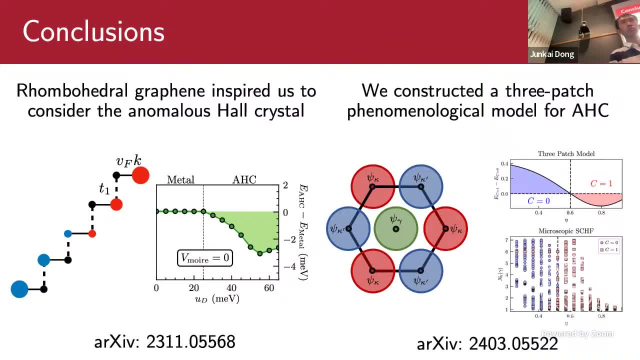 your mechanism would cross that. the fact that you need an enhanced susceptibility to the moray state is is allowing the system to do this, and if you try to put a third as many electrons or half as many electrons, then it's losing the advantage that your mechanism is providing. 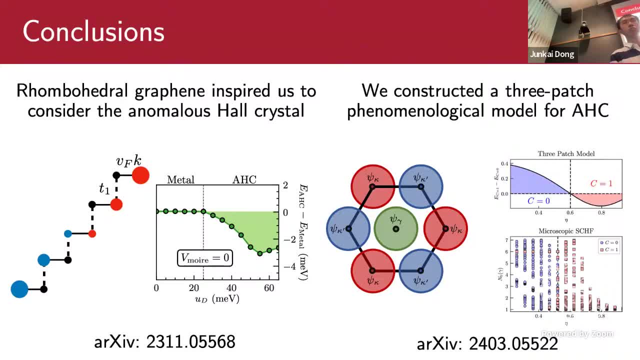 and it's now having to work much harder to form a fraction. I agree with the sentiment that maybe wouldn't it be so nice like: okay, how do you say this right? rvb is not, it's probably not the ground state for cuprates, and yet people have studied rvbs. 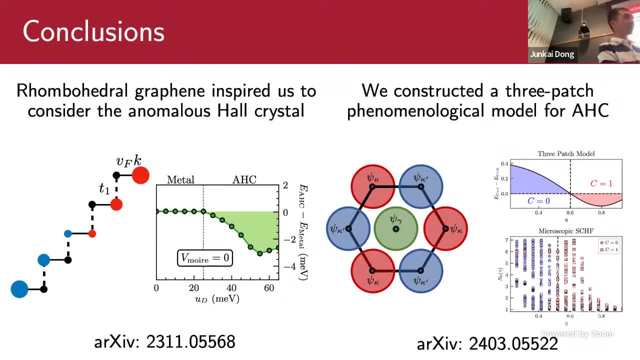 this is by no means rvb, but theoretically I think it is still worth pursuing. yes, Yes, Wigner-Crystal When, for example, one seven. indeed, I do get a Wigner-Crystal state, but I'm not sure you get sigma xy proportional to the density. 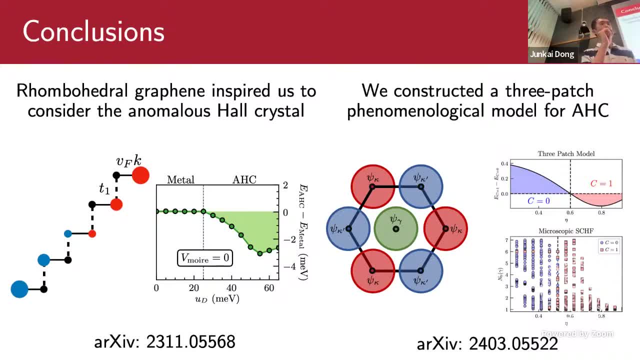 Oh, I see. Okay, let me say this Probably: what you're thinking of is the translationally invariant case. Translationally invariant, the Strata formula is slightly difficult there. In the completely clean case, the Wigner-Crystal is not an insulator because you can expand. 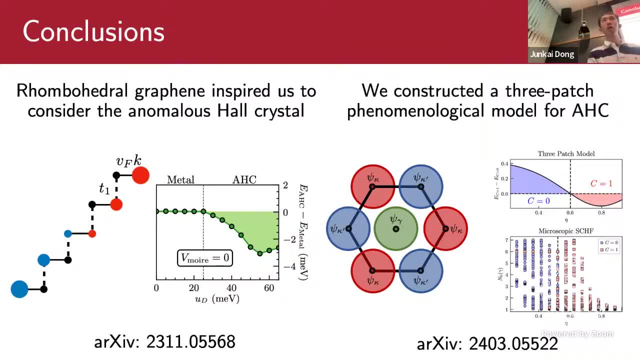 First of all, it can slide, so the sigma xx is non-zero. Two, you can dope into it by shrinking the lattice constant, so it's by no means an insulator. So Strata's formula doesn't need to hold that limit. If you read Burr's paper, Burr's paper in 1989 is actually called: 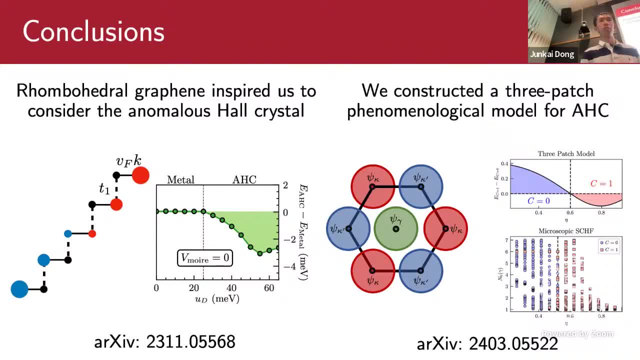 Hall-Crystal versus Wigner-Crystal And I think in the reference somewhere in the reference he has a discussion on the Strata formula. Basically, if the charge density can be, Is the charge density pinned by the magnetic field, or you know. 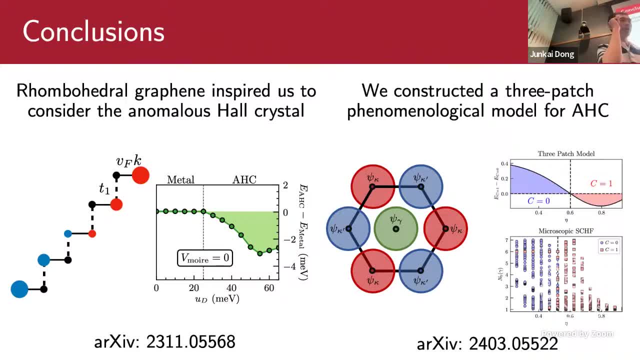 or something else. he says the Strata or the sigma xy. he says the Strata formula can only be used if the Wigner-Crystal is pinned, meaning it becomes a true insulator. It can slide right. The Wigner-Crystal can slide like this if there is no disorder or potential pinning it. 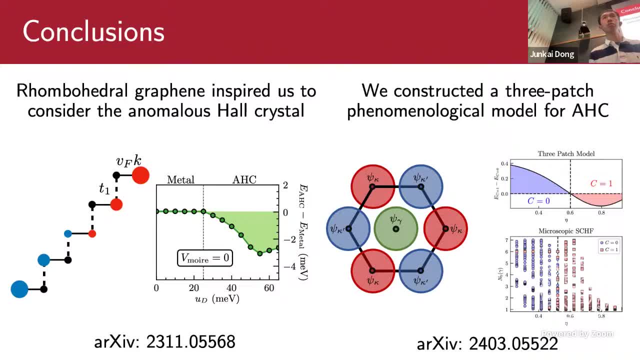 No, I mean what you're saying is correct. What you're saying is correct. In the clean limit I agree that the sigma xy is proportional to the density. However, in experiments- I'm not sure the experiments at mu- equals a seventh- it has sigma xy non-zero. 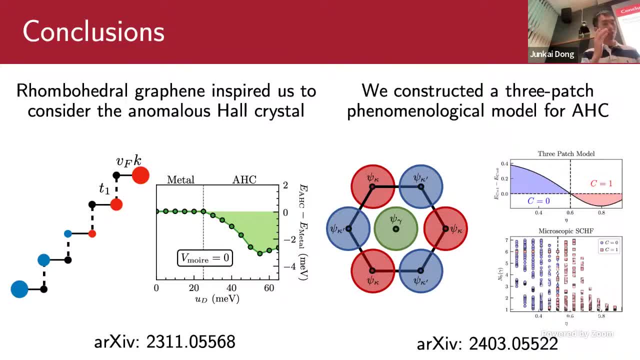 That's what I? Yeah, yeah, That's not the clean limit. Yes, yes, sorry, yes, I should have made a that clear. yes, You need pinning. You need a pinning to make sure that this is an insulator, Otherwise, 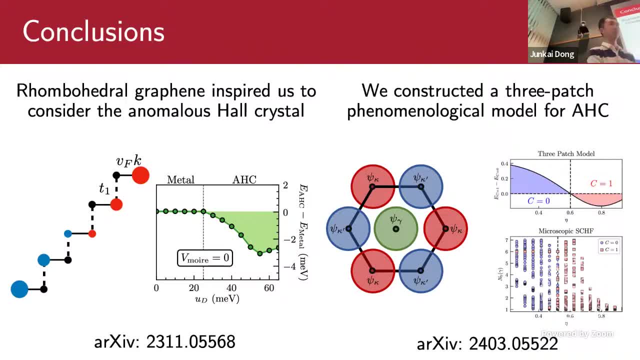 I don't even know how to think about that. Yeah, think about that, But once you add a little bit pinning, which means that you are necessarily away from the clean limit, then sigma xy is pinned to one, which I agree. 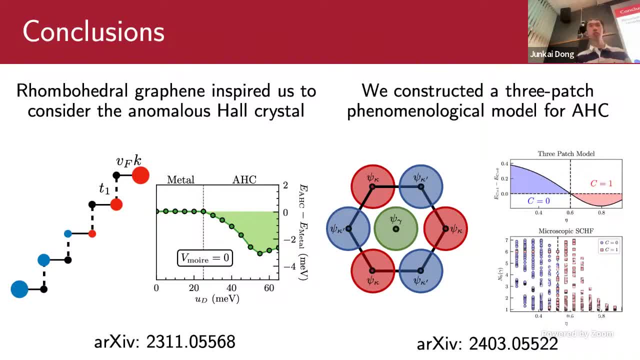 I agree. No, no, no, no. I have continuous translation symmetry. right, I have a continuous translation symmetry, which means that my slendering is Yes, yes, yes. It means that my slendering is growing, that my state can slide and expand. So it's exactly the same as the as the Wigner crystal. 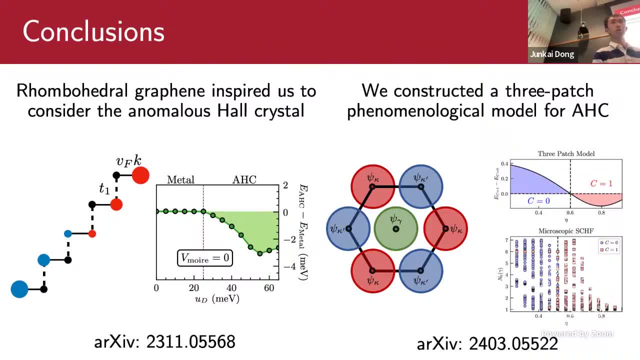 without pinning. The Wigner crystal without pinning is not an insulator, But I thought you were getting nesting ribbon tartan fluid in your mid-heel wheel. Uh yeah, That gives you a tricentrifugal surface. It won't have any fluid surrounding it. 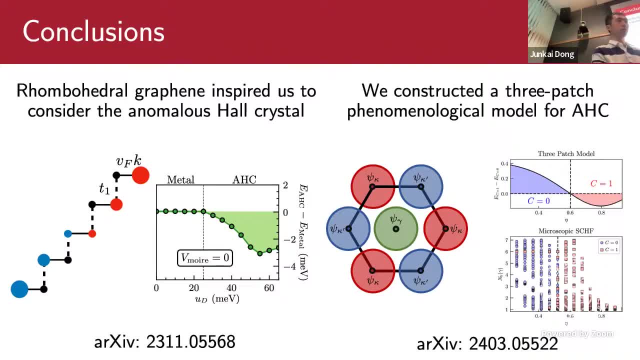 That okay, that I can probably agree with, But translation like given continuous translation symmetry, right? Well, I think I'm really lost, Because you're very conservative and to talk about filling the needs, that is deserted. So I didn't hear. why are you in a history model? 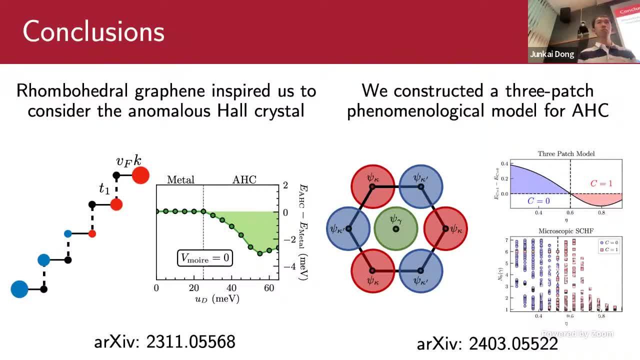 Continuous translation. I know what. I know what tricentrifugal is And the statement that you want to make by associating to Wigner crystal is seems to be a philosophy, not something that comes out. I'm not sure I agree, Because the calculation at the level of your calculation. 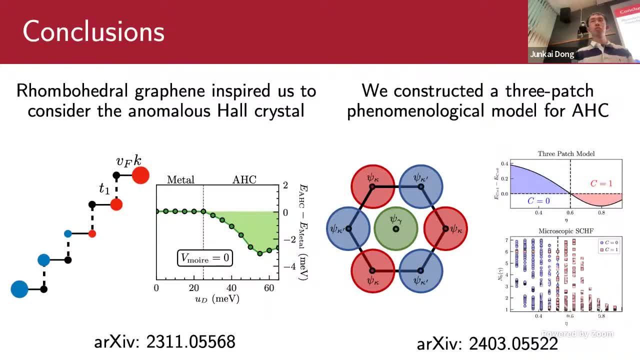 the electric ball is the same as all once on all electric balls. The difference is you're breaking values in a tree and in that value state as it is, you may or may not have 100.. But as far as sixth-stageろう symmetry breaking out of Hartree-Bollin-Mil��� field, 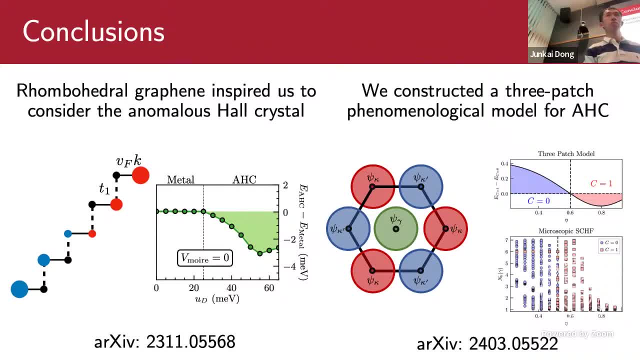 that's actually the same as quantum all stripes and quantum all bubbles, And they didn't say what they had is some zero-threads separation, Although they started with tricentrifugal. No, Okay, so so I agree. I agree that it's a tricentrifugal structure, right? I mean it's, you know. that kind of. you know you can even find a tricentrifugal area in a deep stream, Like if you thing about a total mass of tricentrifugal area. you can't call it tricentrifugal. 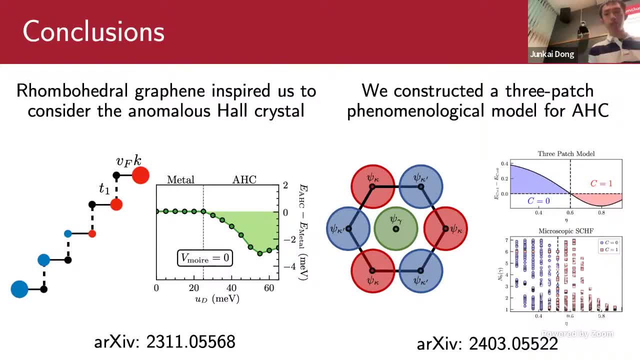 So I agree. I agree that I can agree with the fact that you know you can choose to call it a charge density wave. However, what I'm not sure is that the physical response will be significantly different. So do you think it is charge density wave or do you think the physical response will be different from the charge density wave? 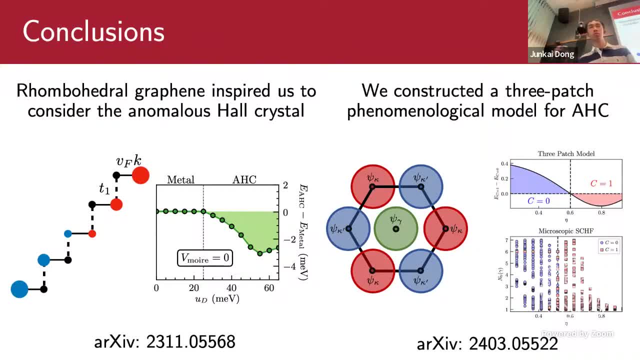 For example, what response are you considering? I think the CW in the clean limit. So CW, even though it drifts, even though it, even though it drifts, do you still think that it is an insulator When it's being pinned? then we're all, I think. I think that's the limit in which we can agree. 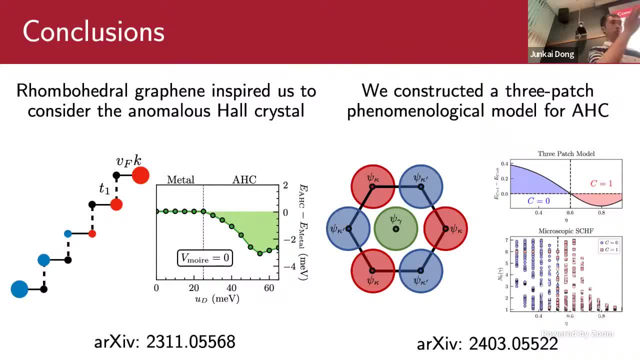 You know it. When, when, the, when the crystal cannot move, When the crystal cannot move, then you know everything is clear. It's a good insulator. You know Rxy is, you know Rxy is, is whatever value that the trend number is. 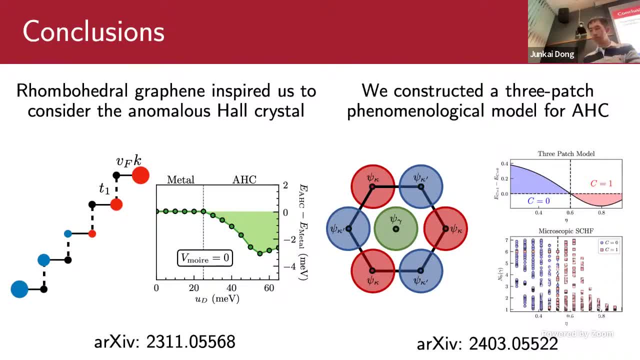 I'm sorry, but I just think I listen to the adjunct call and also I was really really confused. So it looks like. Do I understand this correctly? Calculation is the same as that of charge density wave, What? what is the observation will be the same as charge density wave. 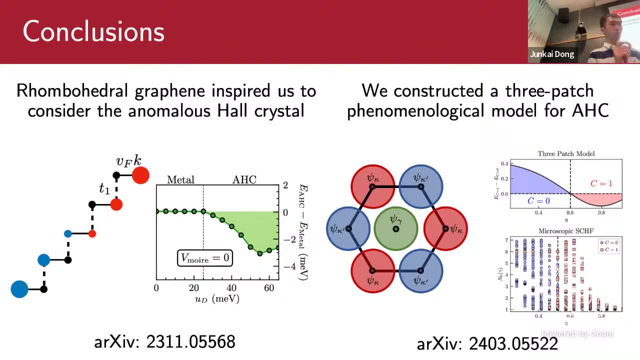 But you want to think about it from a different perspective. I'm not sure I understand either of the two claims that has been made. One: the calculation is exactly the same as charge density wave. As far as the translational sensitivity rate measurement that is used to access your heart rate volume field theory. 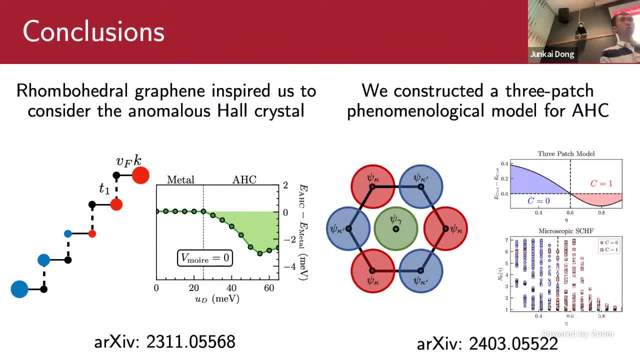 The following: The following: Well land, the level doesn't have a Fermi surface, So the heart People have patients of. Start from that They can get different levels And they don't have to fall And they get a translation. 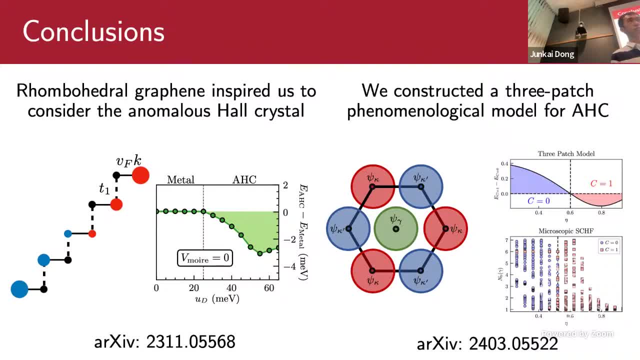 Completely agree. Yes, that's exactly what. That's okay. That's one way to interpret what we're doing. Indeed, we both use hard to talk. We both find translations He symmetry. We both find translation symmetry breaking. Yes. 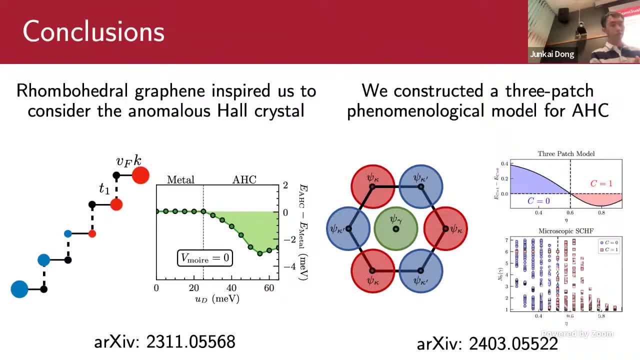 You didn't start with. I indeed did not start from Landau levels. Well, you know that that's. He was also starting with nothing. That's why it was important by getting started. Oh, you're true, My band was. 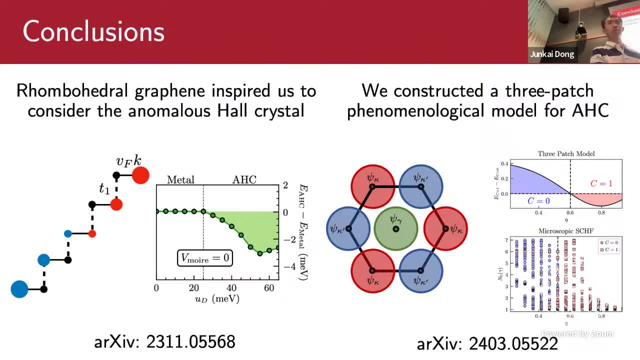 My band was Was. Was Was the service versus Okay. Whatever, Consider it, The positive interaction You can't get. Sounds good, Sounds good, Agreed, Agreed, Okay, Sorry, Is the computer resolved or not resolved? 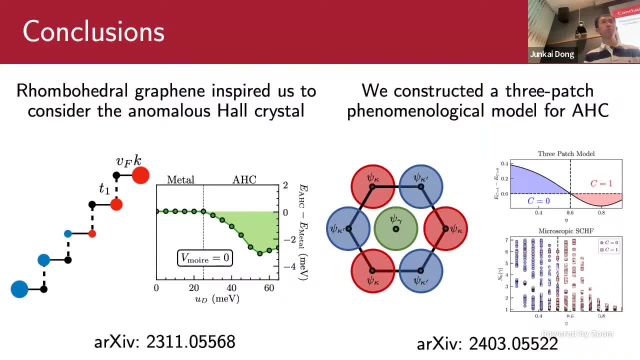 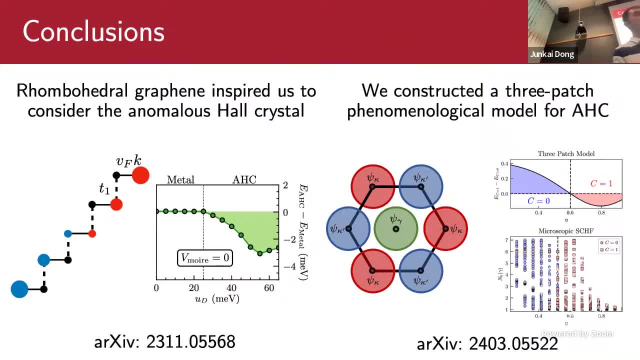 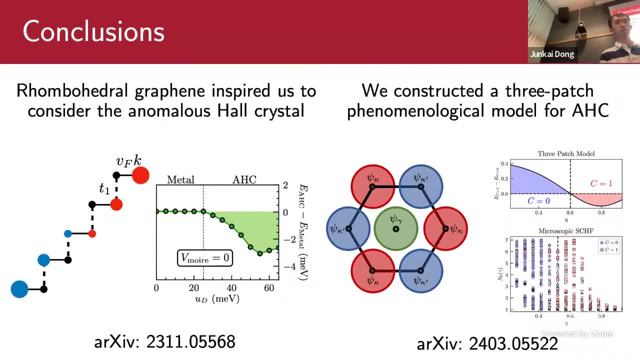 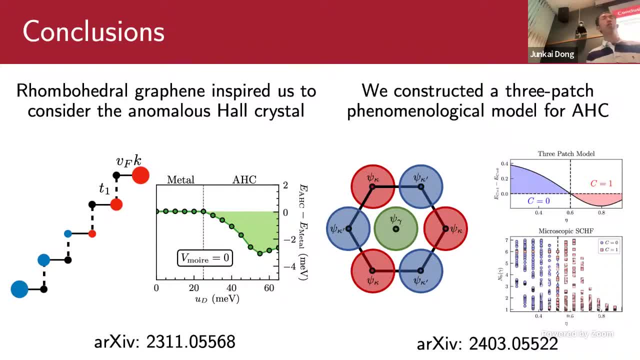 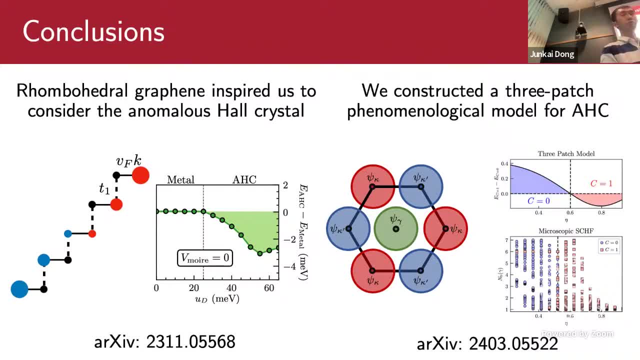 There's no such scale in the setup that we have considered The virtue not applied. A moment ago you were saying maybe I can get fractions. Now I'm saying the lattice got to the set by the density Indeed. okay, probably. that is another thing. 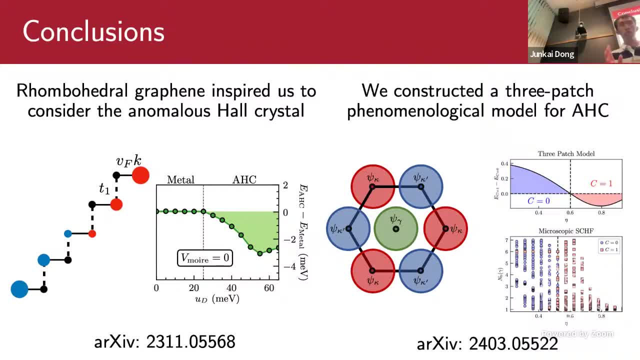 to be considered. here We are by. okay, let me make this very clear: We have never, in our calculations, claimed to say that we have obtained a crystal with fractional, a crystal with, you know, fractionalization. We have never said that. 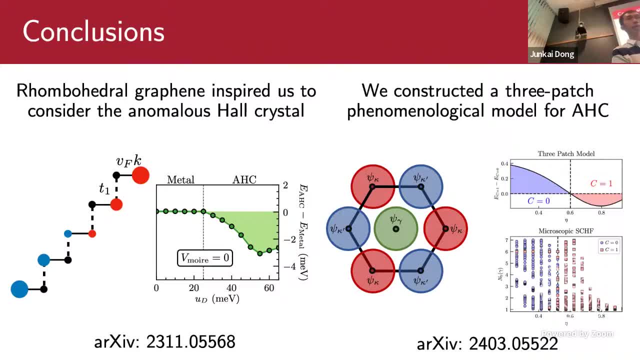 All the fractional calculations were done in a setting with Mori potential And you know if, even if we obtained something in the fractional setting without you know, even if we got a fractional state that spontaneously breaks translation symmetry, I don't think we have, you know. 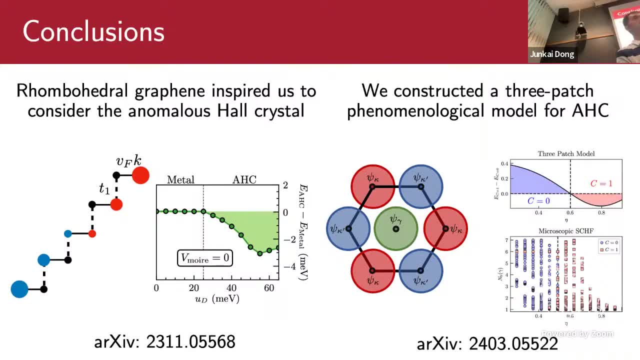 the capacity to claim those states right now. Right now, the only responsible claim that we can make is that the integer state in our numerics is translation, is translation symmetry. The fractional states are not and we do not have capacity to claim them. 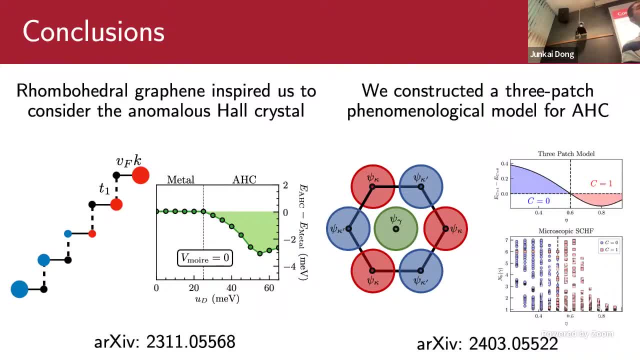 Yes, I don't know about the other calculations, but your electron, your electron state, your electron band, Yes, That form, the chair and stuff, Yes, Are the same as the electron band that you that you were talking about, right?